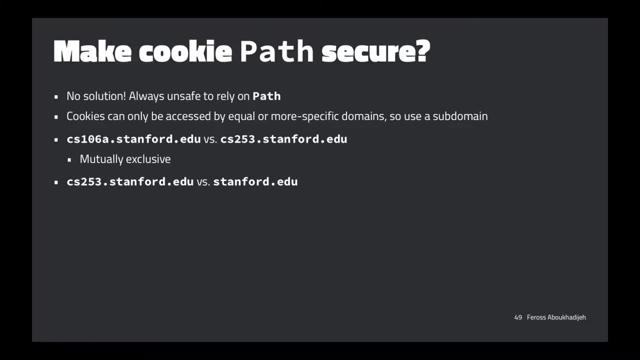 the rules specify right here. So cookies can only be accessed by equal or more specific domains. So the two domains are on an equal level, can't access each other. But what about this example? here We have 253.stanfordedu and stanfordedu. So, based on the rule, what do we think is gonna happen here? Should? 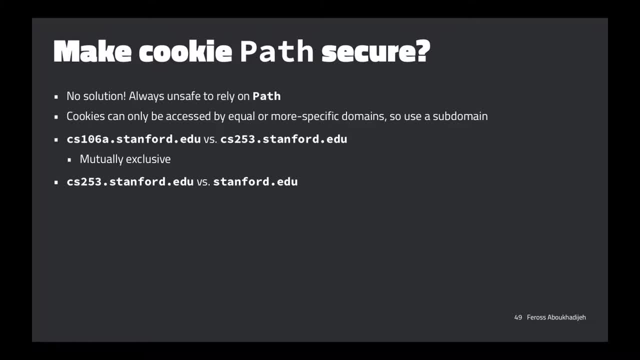 these be. should these be able to access each other's cookies? Yeah, go ahead. It seems like stanford should be able to access 253's Cookies can only be accessed. oh, so it's actually flipped. yeah, So it's cookies can only be. 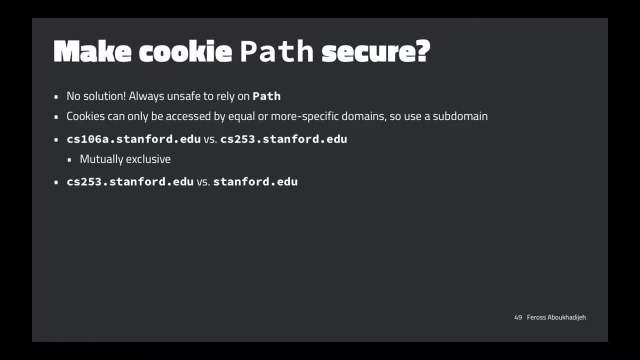 accessed by equal or more specific domains. So that means stanford's cookies can be accessed by stanfordedu and more specific. So this is like what they mean by more specific, Like more things tacked onto the end. Yeah, so it's. 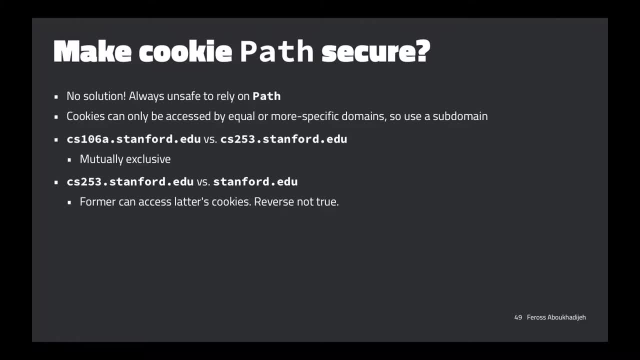 the former can access the latter's cookies, But the reverse is not true. It's kind of weird, but that's sort of just how the rules are. That's actually a reason why, in the case of the stanford login system, they put the cookies for that on a. 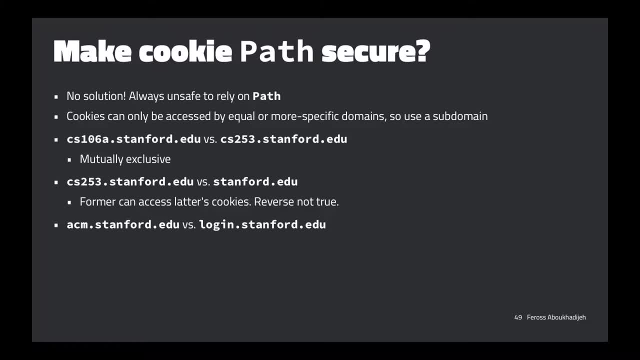 completely separate subdomain. So loginstanfordedu is where you go to sign in and when your password is correct, it puts a cookie on that subdomain And And that means that, like the ACM club, for example, couldn't go ahead and read those cookies. 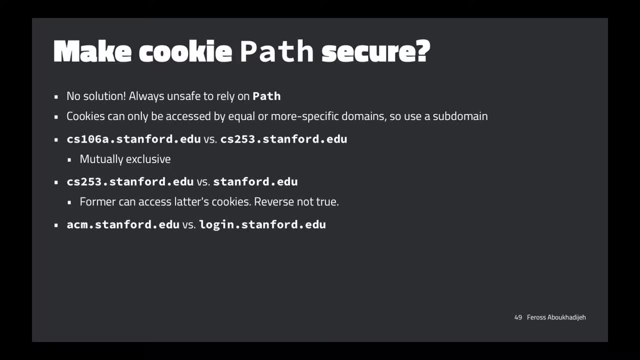 because, again, it's not a more specific subdomain. So, yeah, these are sort of separate cookie jars. And then what about this example here, Just to make sure we're all on the same page, Which can access which in this example? 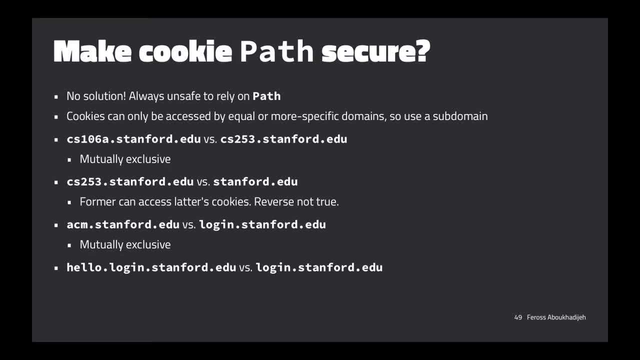 Mm-hmm. Oh yeah, go ahead, Right, exactly. yeah, That's right Cool. So, because of this, like, we sort of just shouldn't rely on path. One thing, though, is: the default value for this path is actually the path that you're currently on. 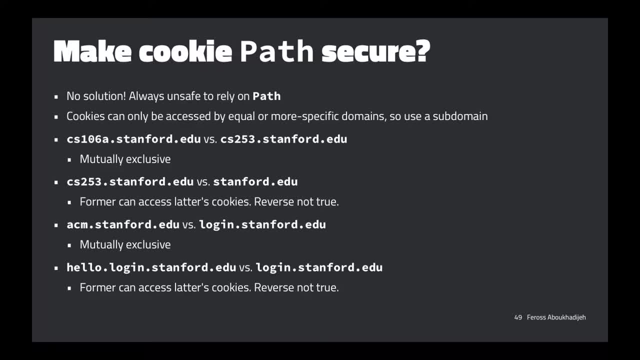 when the server attempts to set the cookie. So if you're on, like the 106a page, and you don't specify path, because I just said, don't do that, it's not secure, don't rely on it- So you just omit it. 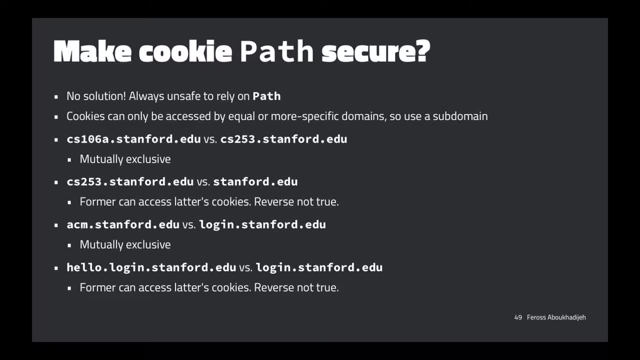 Then it's gonna end up giving it a path of the page that you're currently on, which is maybe unexpected. You might want the cookie to be available everywhere, since we're not relying on this as a security mechanism. So let's just not fool ourselves. 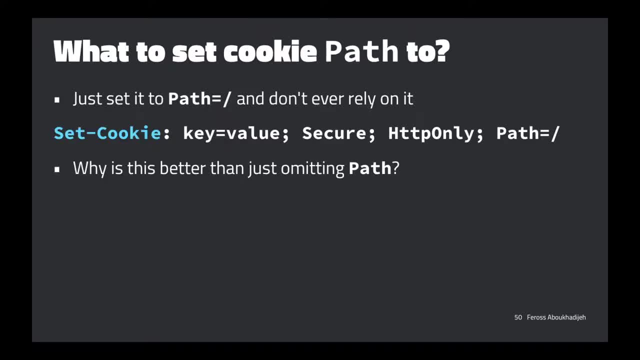 and just like, let's not use path at all. So what we really need to do here is actually explicitly set path to the root of the site. If you do this, then it's sort of- I think it makes it clear, because you end up with: 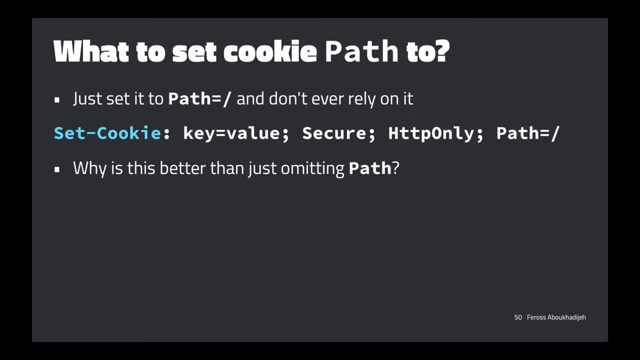 the cookies are very clear. the cookies are very clear. the cookies are visible everywhere where they're actually visible. you know what I mean. You're not sort of fooling yourself into thinking that this is doing something. So that's my advice. 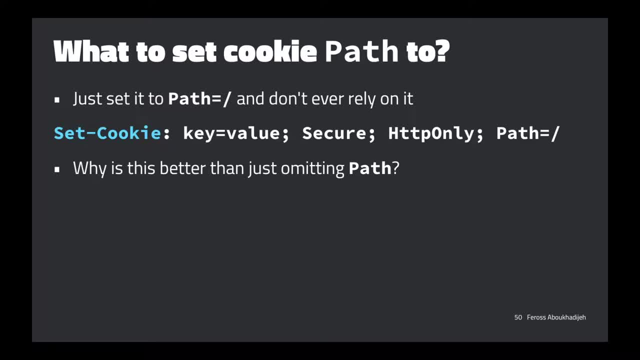 to sort of always set path to the root. So now this is sort of what our cookie setting looks like. We've done secure, so that the cookie's only sent over HTTPS. We've done HTTP only, which weirdly sounds like it's contradicting the last thing. 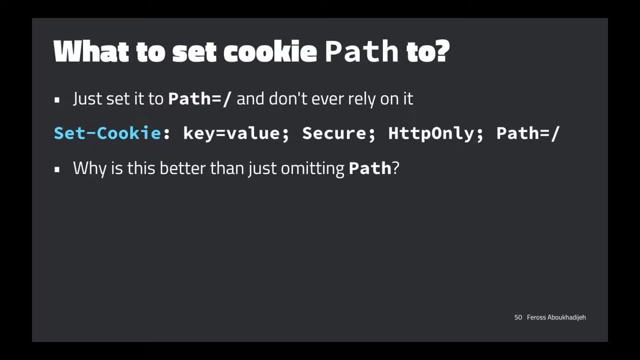 but who remembers what HTTP only does? Yeah, So if I bring this to not have access, so like this one's the image one so that you cannot. so the only HTTP request can access it. Yes, that's the one. yeah. 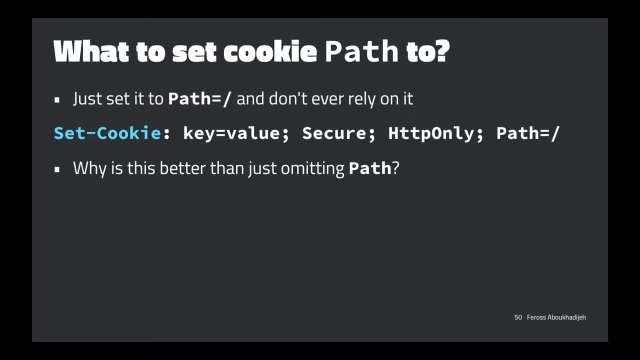 So, basically, if you're trying to attempt to access this cookie from JavaScript, so from JavaScript running in the browser, you won't be able to see the cookie. It'll be there in the browser and it will be sent to the server and HTTP requests to the server. 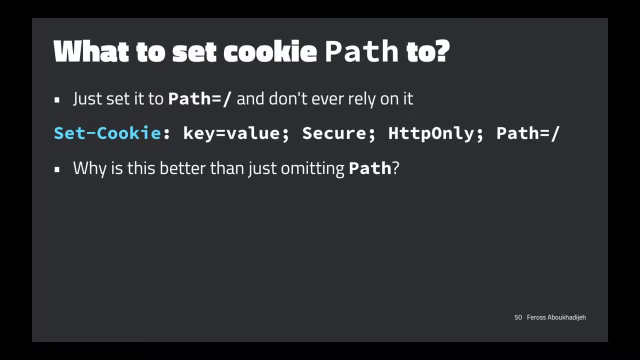 but code running in the page can't see that it's there And this is a nice defense against an attacker. gets code running in a page then sort of limits the damage that they can do. Okay, so we have those two and we throw in path. 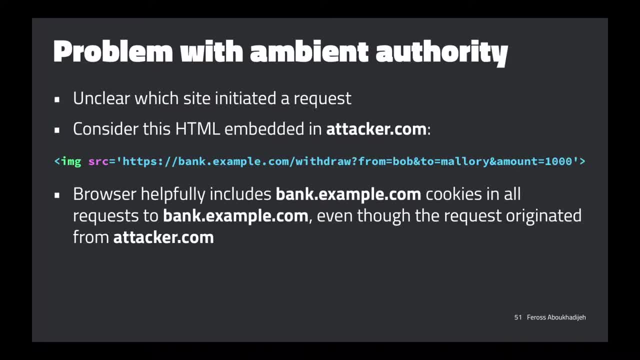 And so this is better for the reasons I said. So there's one other sort of general problem with this whole cookie design, which is sort of it's one of the benefits of ambient authority that we mentioned before is that it sort of automatically. 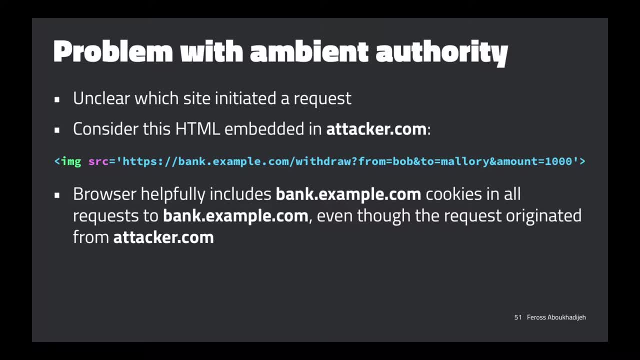 every request you make is sort of has the authority of this cookie, but it can create problems when the browser sort of helpfully includes cookies. So if you have cookies in requests that you wouldn't expect that it would, So in this particular example. 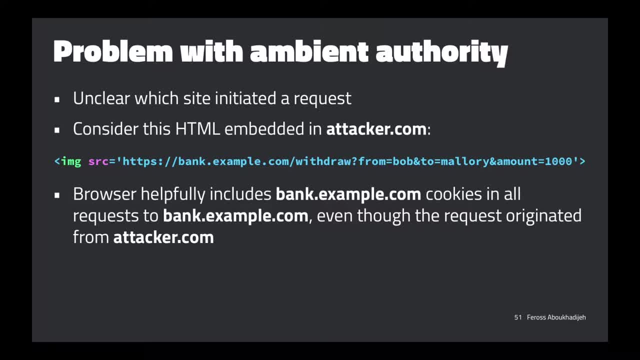 say that we're on attackercom. Okay, so we put the link. we ended up on a sketchy site And this site just embeds an image that goes through this URL. So this URL is attempting to withdraw from Bob's account to Mallory's account. 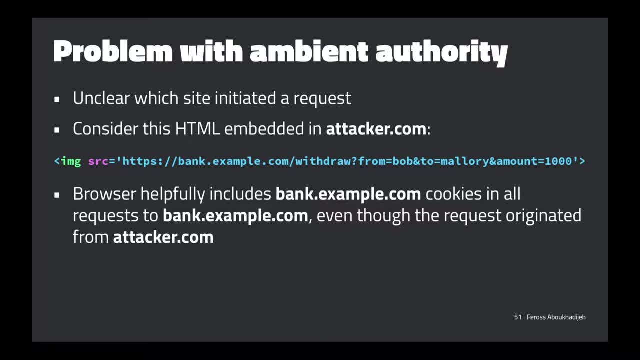 an amount of $1,000.. And obviously this list probably should have been, should have been implemented by the server as a post request, not a get request. That would be sort of one defense against this, But obviously this should have been. 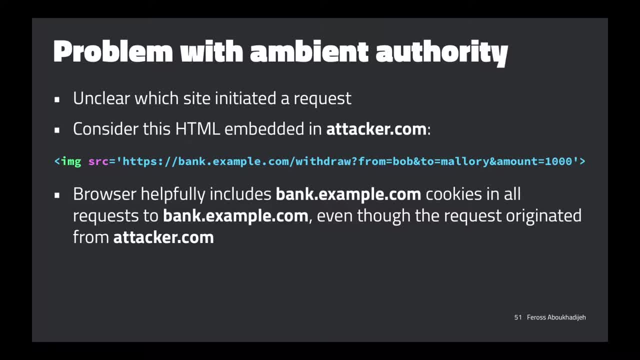 should have been implemented by the server as a post request, not a get request. That would be sort of one defense against this. But obviously this should have been. should have been implemented by the server as a post request, not a get request. 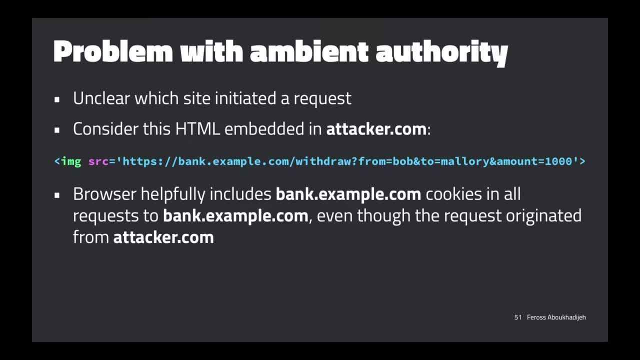 Let's say that. let's say that it's a get request, So the browser's gonna attempt to fetch this and, you know, display it as an image, And the response from the server, in this case, is probably gonna be some kind of JSON. 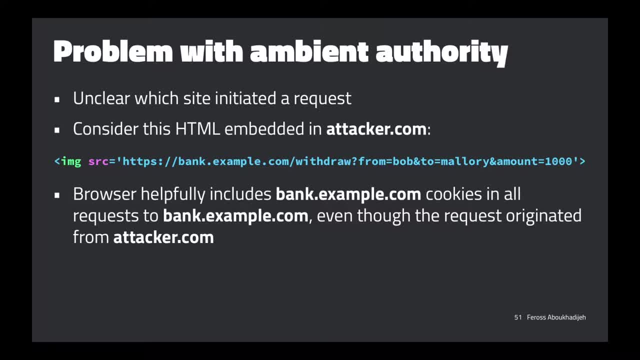 or something that's not actually an image, But that doesn't matter. The attacker doesn't care, because the request was able to go through to the server And the browser noticed: ah, you're sending your request to bankexamplecom And it's gonna look and see. 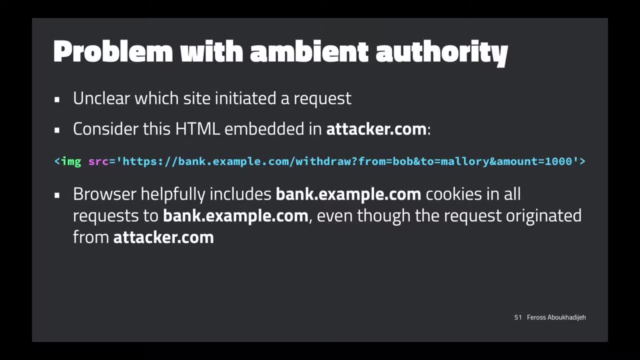 are there any cookies from bankexamplecom And say that the server is sending a request to bankexamplecom And it's gonna look and see? are there any cookies from bankexamplecom And say that the user logged into bankexamplecom? 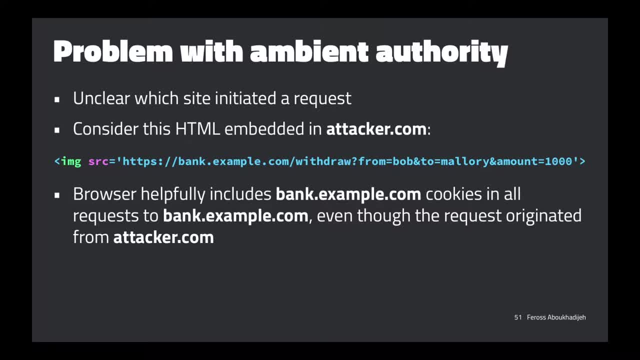 ah, you know, in another tab or you know maybe 15 minutes ago. So they still have an active session with the server And so their session ID is valid. The browser's gonna attach the cookies for bankexamplecom to this request. 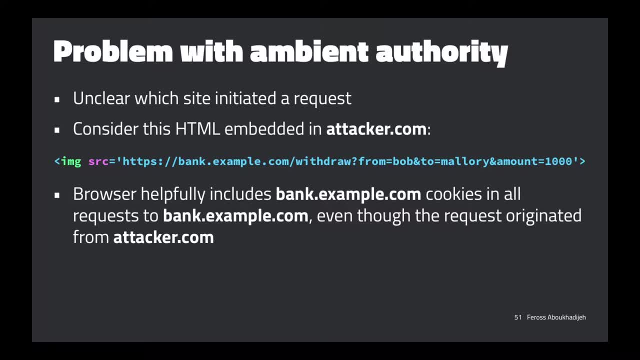 And then when the server gets it, it's gonna look and say: oh, this is like the user's logged in, They have a valid session. Oh, they're trying to transfer some money. Okay, go ahead. It looks valid to me. 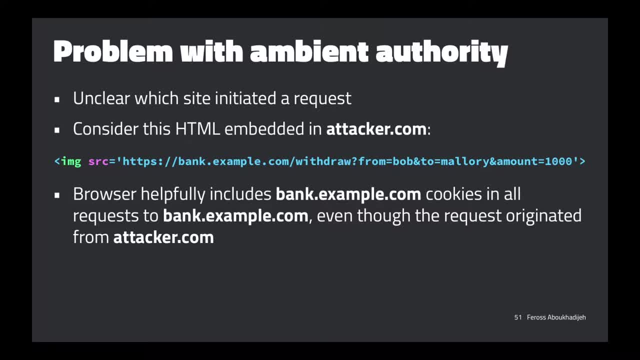 Right, And so this attack site has been able to sort of create a false ah, a false ah ah like a request on behalf of the user with the authority of the user, Right. So this is really bad, Um. 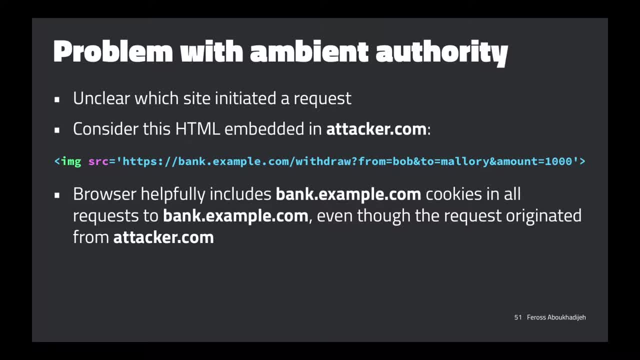 does this make sense? why this is possible? Okay, cool. Ah, I see some a couple confused faces. All right, Yeah. In the first example that you showed in the previous class was that. was that like I thought it was? 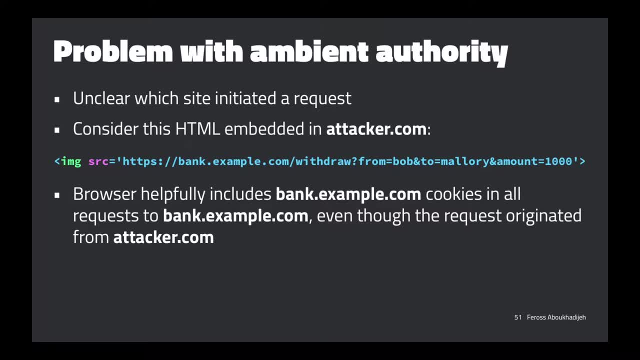 like an attacking website, or was this always like a different website that was attacked, or something like that? Yeah, So this is. this is not controlled. Uh, which example are you referring to? Like the image is like: 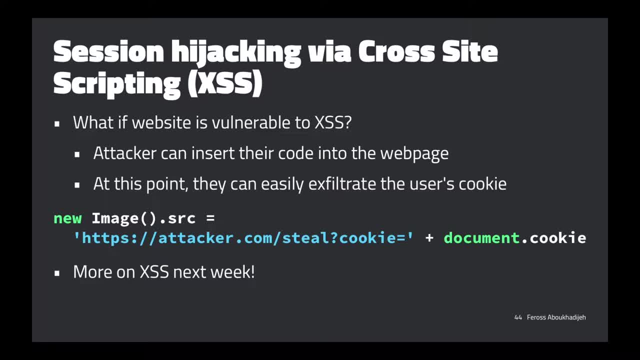 the same example in the previous class. Uh, was it this? Let me see This one. Yeah, yeah, oh yeah. so this, this is just. this is just a method to sort of exfiltrate data Um. 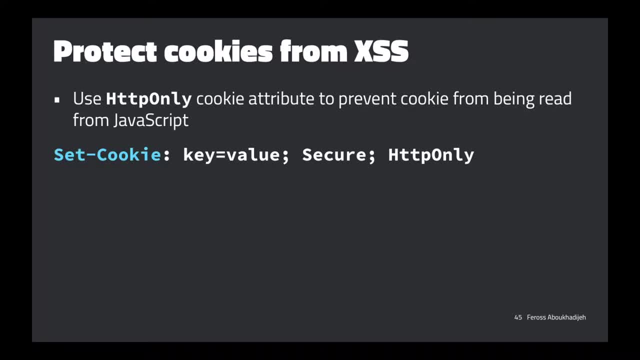 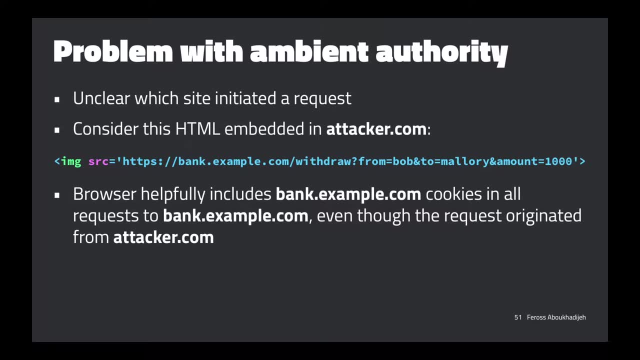 this is just sort of a way to sort of send a get request to to the attacker's server with some information that the attacker wants. Um, we're on a different website, We're on the attacker's site, so it's sort of. 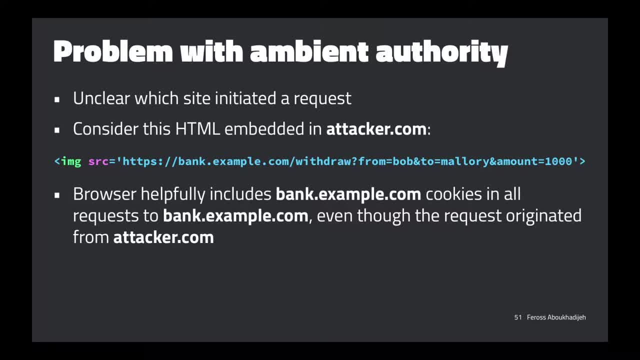 it's sort of the reverse: We're on the attacker's site and we're sending a request to a legitimate site that the user is actually um logged into, And because the browser has this behavior where it tacks the cookies on automatically to any site. 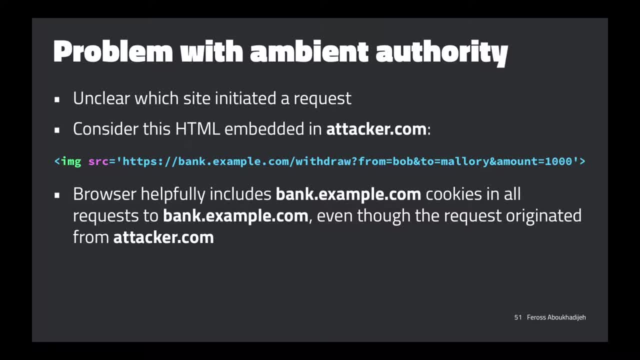 that that has associated cookies, then the the server. if it just sort of naively, uh looks at this request, it'll think that it's actually authorized by the user. It's gonna see a request come in with both the correct cookies. 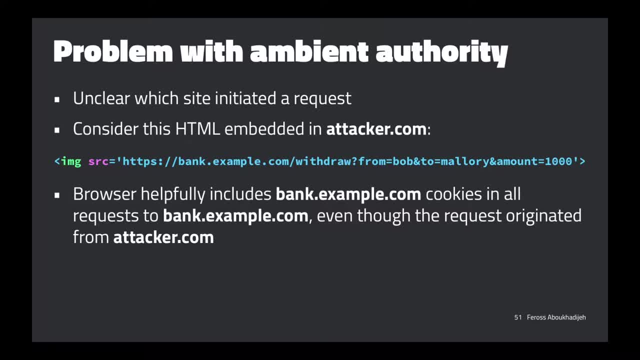 and then it's gonna go ahead and do on behalf of the user: Uh-huh. So in the first attack we would need to have the same to be in the same domain or be a more specific subdomain, Right? 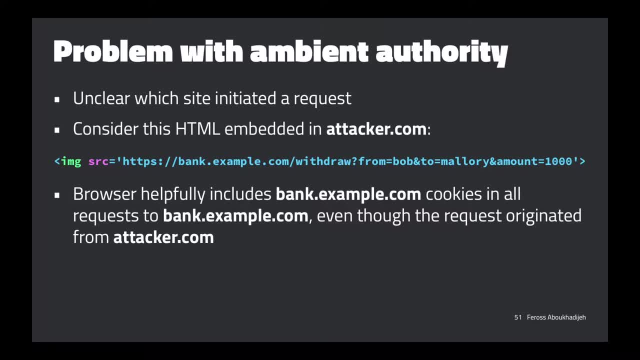 Couldn't you intercept, like, since you're young enough to say: like this HTTP request and just steal the cookies too, Like, just send any any request to the bank for like simplecom and just like send also? 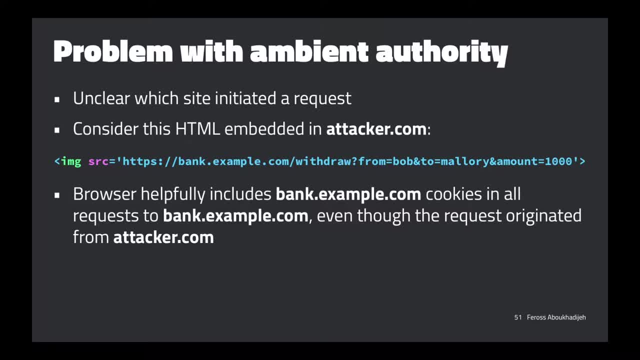 like those. you know the attacker's servercom and then you're sending this request to bankexamplecom. Is that what you're saying? Yeah, So I'm. I'm like the attacker's server, Okay, And I'm sending. 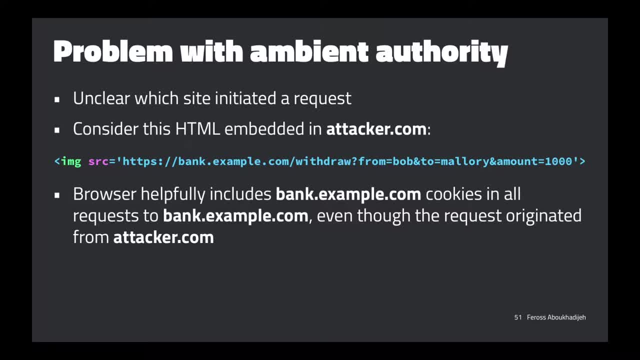 so now I send the, the attack to, I send the the image to bankexamplecom and the browser would: would tag the cookies right? Uh, are you sending this request from this attacker's server, From the client, From the client? 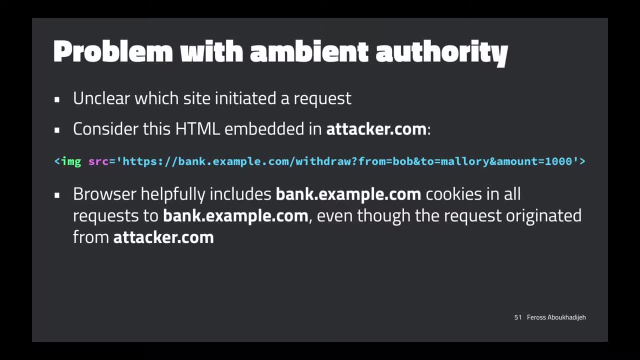 Yeah, so if you're, anytime you send a request to this server, the browser will attach the cookies for that site automatically. So could I intercept the No? you can't. So yeah, that's a good. so it's a good question. 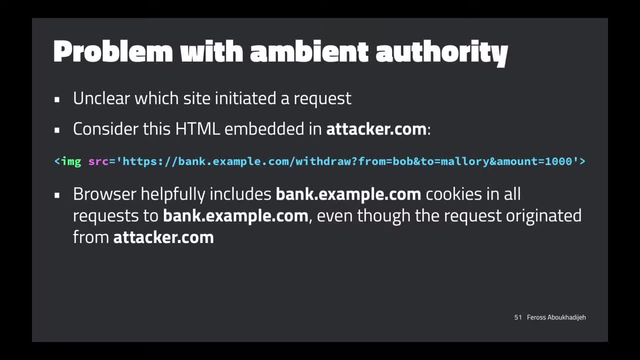 So, in this situation, the site that's embedding this image, so the attack site that's embedding this image, it actually can't see the actual request that's going out. The browser's just gonna gonna fire that off, and it's not like. 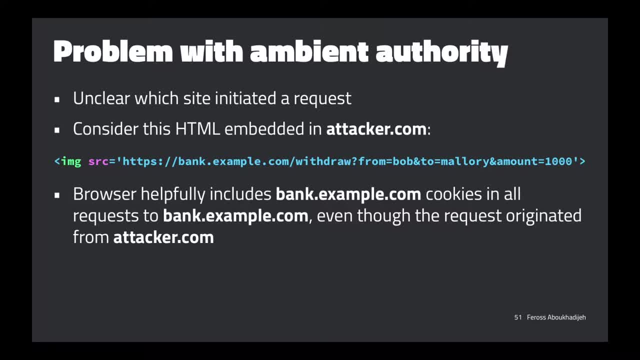 it can observe it or anything like that. All it can do is there's not really much that it can see. One thing it can do is it can attach event handlers to this image. It can attach on success and on error and it can sort of find out. 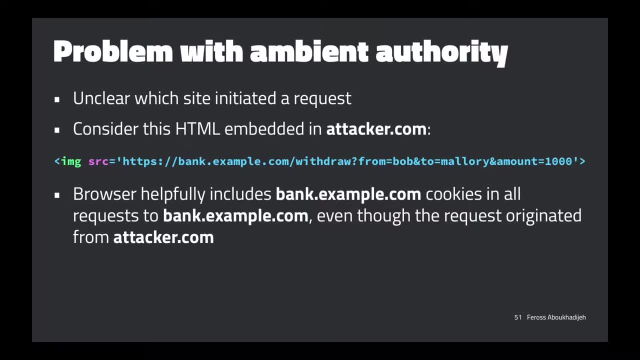 whether what was returned by the server was a valid image or not. It can detect that, but obviously it's not gonna be a valid image in this situation. That's pretty much it, yeah, Mm-hmm, Can you do the same thing? 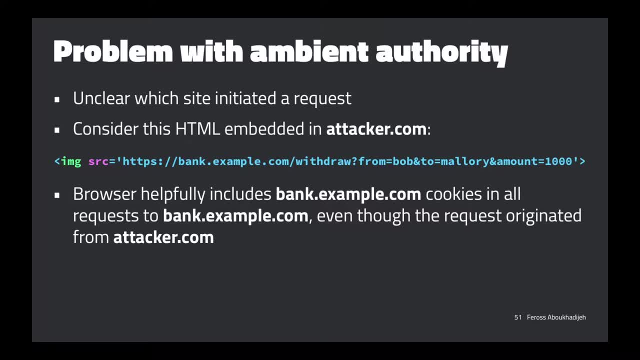 in JavaScript with like KJACK requests. Uh, yeah, so that's a good question. So we're gonna get really into all the nitty gritty that's gonna happen in a couple minutes, Um, but uh, but in general, 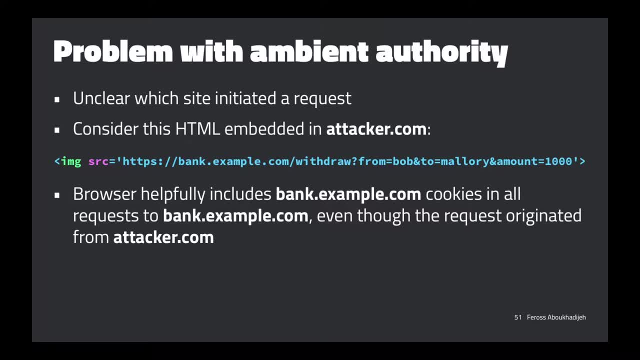 uh, in general, no, Um, when you're firing off an AJAX request, um, actually we'll just save that for. save that for a little bit, We'll. we'll get into that in like a couple minutes. 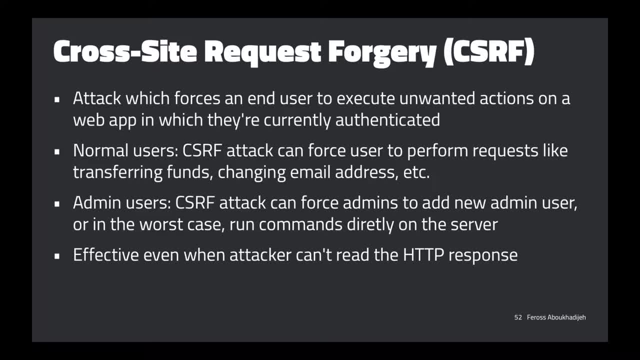 I promise Okay. so so this whole, this whole idea here is is called uh, is called Unwanted By The User, Um and uh, and it's enabled by the fact that the user's currently uh. 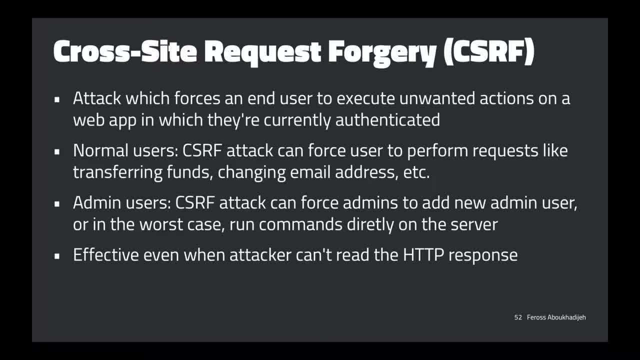 like authenticated or, you know, or logged into that web app. Um, so why would you do this? Uh, we just gave an example at the bank. Uh, so that's like a, a normal user. you're sort of executing. 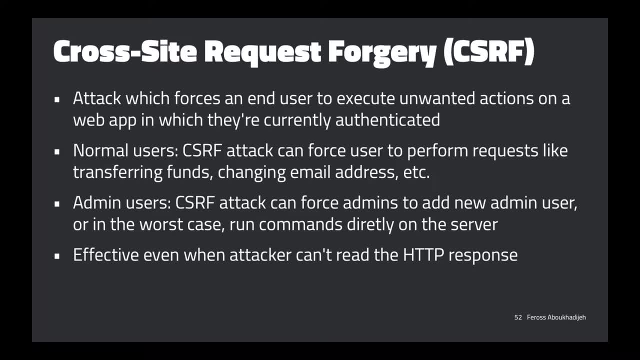 an attack that's forcing the user to perform some kind of request that you want them to do, like transferring their funds or changing their email address or resetting their password or whatever kind of request. maybe they're an admin of a WordPress site or something you can. you know that request can be much more damaging. 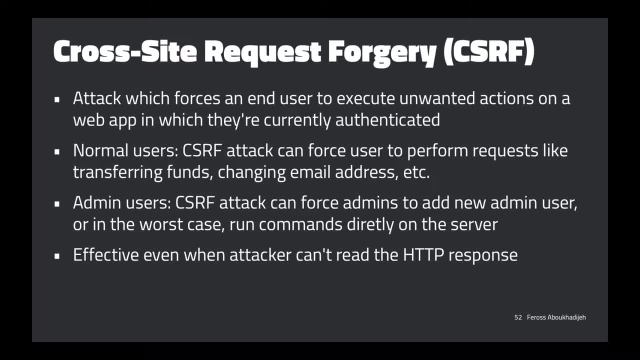 You can. that request can potentially, you know, create a new admin user on their site, or it could, in some cases, allow you to just run code on the server. If you're logged in as an admin, oftentimes you can just send a request. 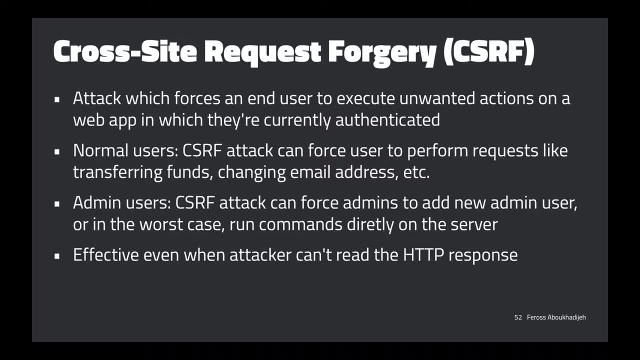 that will just like shell, like run a shell script on the server as a server user. So it's pretty, it's pretty damaging, Mm-hmm. But to create an admin user, for example, the attacker needs to know what kind of like paths, like endpoints are there. 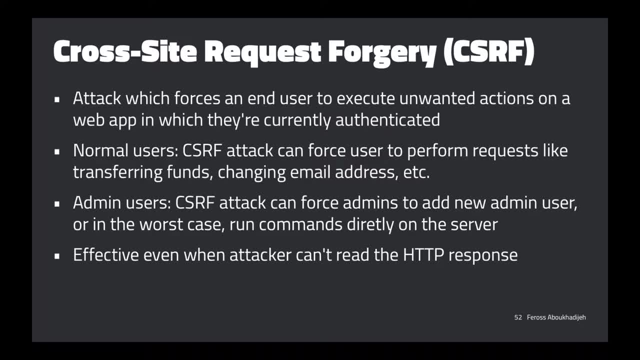 at like the server, right, Yeah, there's a little bit of knowledge that attacker has to have here. They have to first of all know like what the? yeah, exactly. they have to know what the path is. They have to, they have to. 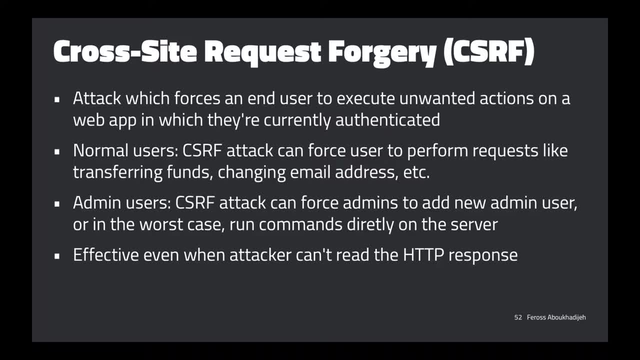 they're assuming the user's logged in, right, If the user's not logged in, then this request will fail, and things like this. Yeah, that's true, But you can imagine this being used in a phishing attack, or you know something like that. 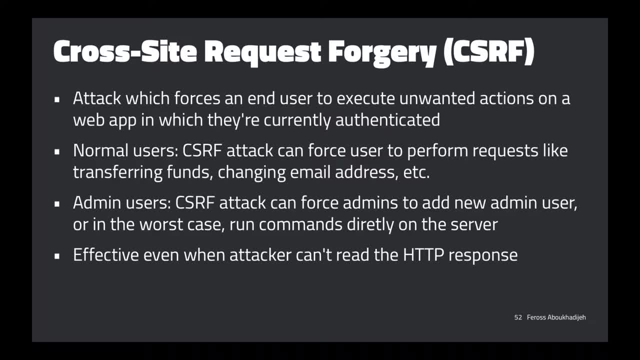 where you send a targeted email to somebody you know they're a member of a particular site, Or maybe maybe you know that, maybe you know that they're a Bank of America you know customer via some of the other attacks we're gonna talk about where you can learn this information. 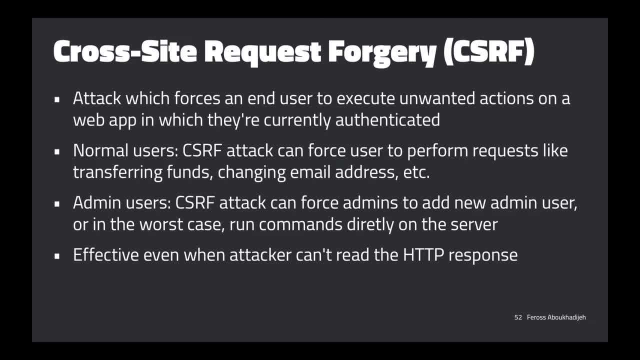 And then what you can do is you can just target your request specifically to the bank URL that you know that they're a member of and just hope that they're logged in right. Yeah, cool. So and then notice it's really important here. 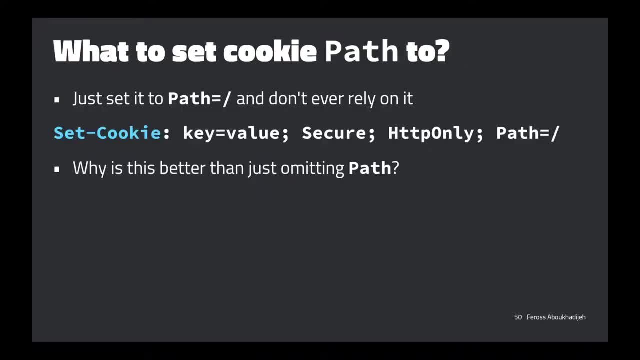 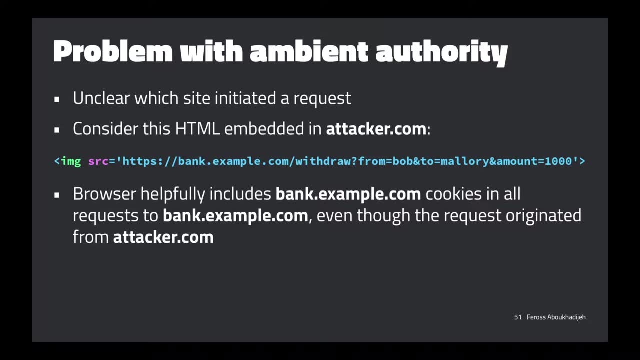 that we didn't actually need to read the response to do this attack right, Because what we actually did here was like this image came this response from, the server came back and the browser attempted to render it as an image, which is gonna fail, but we don't care. 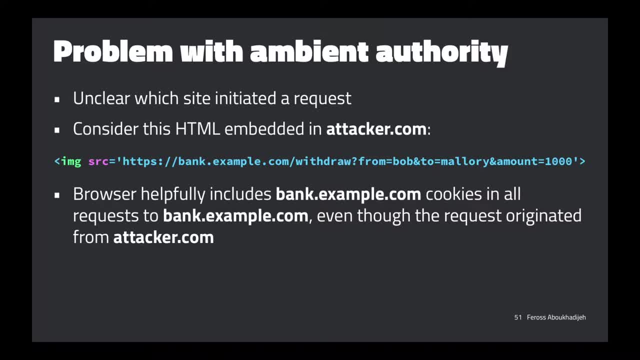 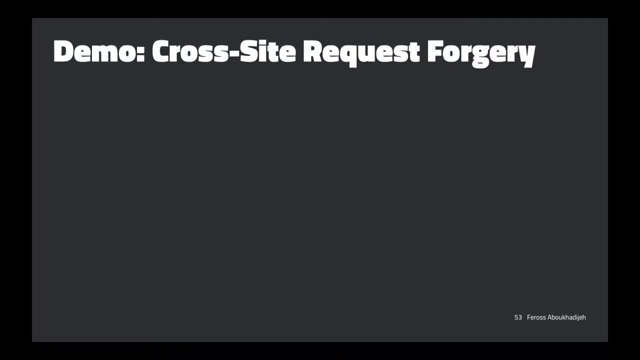 Like the request was sent, the damage was done, right, Because the server received a request and it sent back a response, so the damage is done. Does that make sense? Okay, cool, So I'm gonna just do a little demo of this, actually, 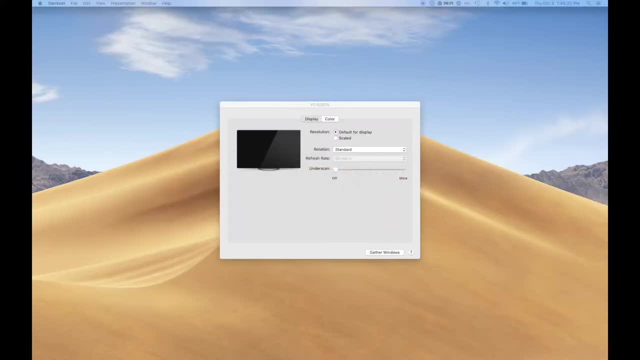 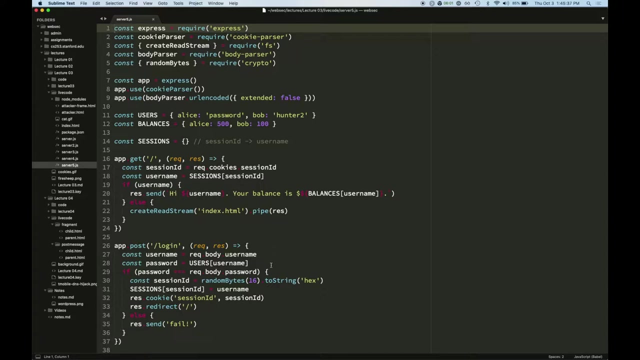 in action really quick. So I really like doing demos. I think they're fun. So let's see here. Okay Cool, everyone can see this. Okay cool. So we have. here is the code from last time for our bank website. 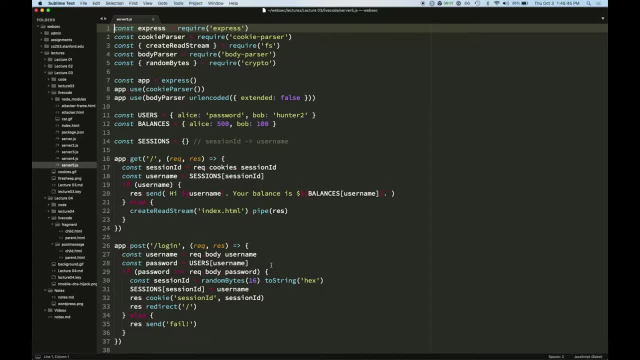 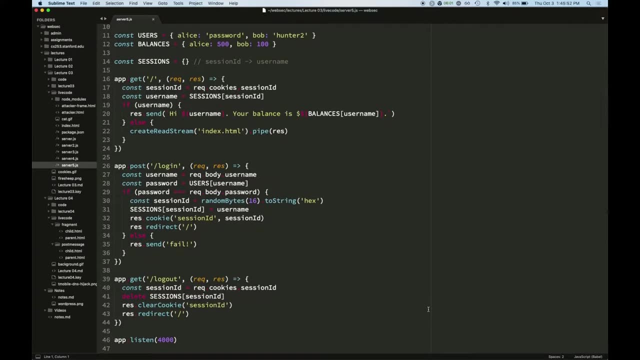 And we're gonna do here is add a path, a new route, to it. So just re-familiarize yourself with the code really quick if you've forgotten. This is the most important part right here. Cool, so let's add a little bit of additional functionality. 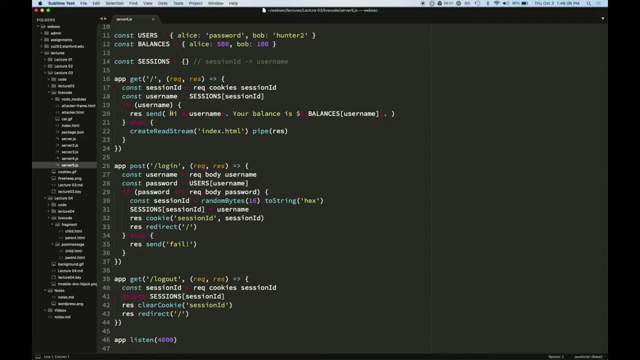 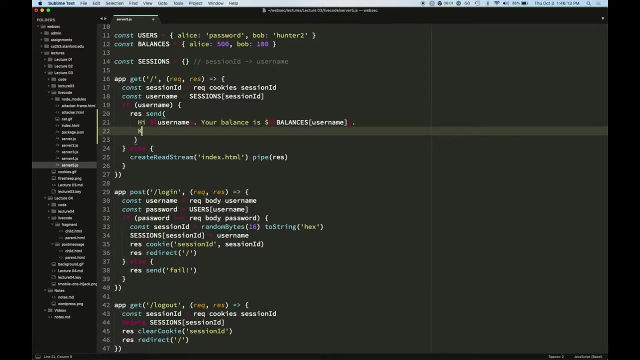 to the site To make it more interesting. So right now, when the user's logged in, we just send back this string here. I think we should change it and make it include a little bit of additional HTML. So I'm just gonna put it right in line here. 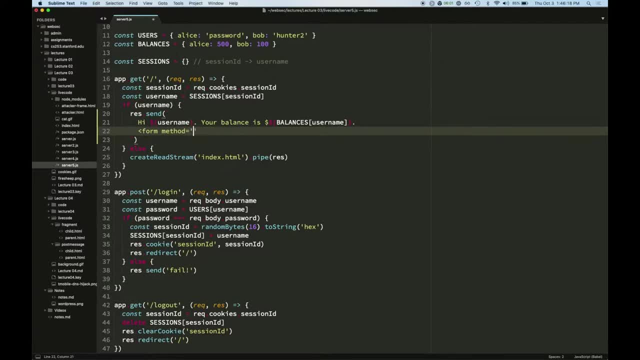 because that's easiest. So let's make a form, And this form will let the user transfer money to another user. So let's go ahead and make the action of this be. it's gonna submit to slash transfer, So we're gonna have to go ahead. 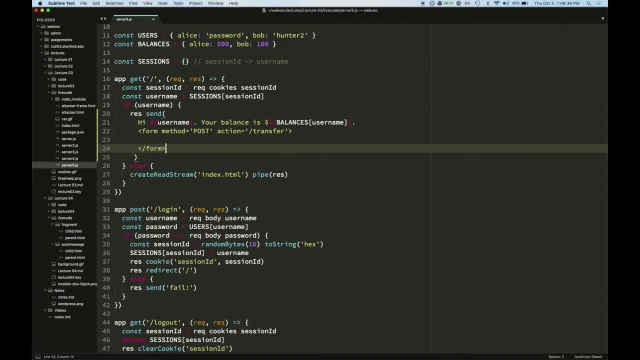 and write that route in a second. Okay, so we have a form. It needs to have a send amount, which will be an input- Let's call the input amount- And then we need to have a to user to send the money to. 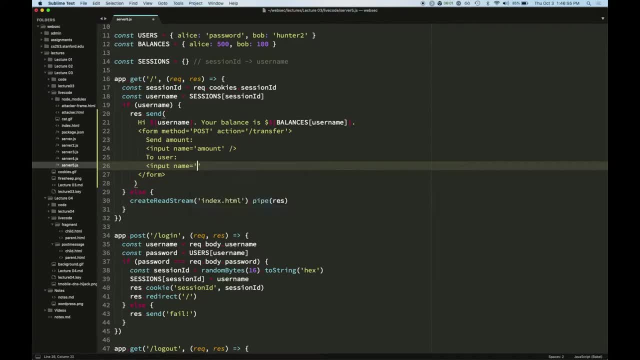 Let's call that to, And then oops, okay, there we go. And then let's just make a submit button. So: type equals submit. Oh, is this big enough for everybody? Okay, type equals submit. value equals send. 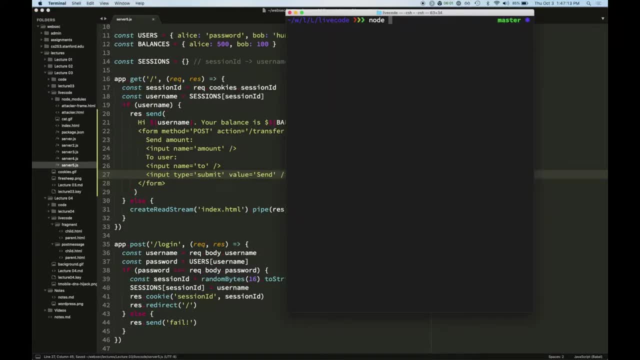 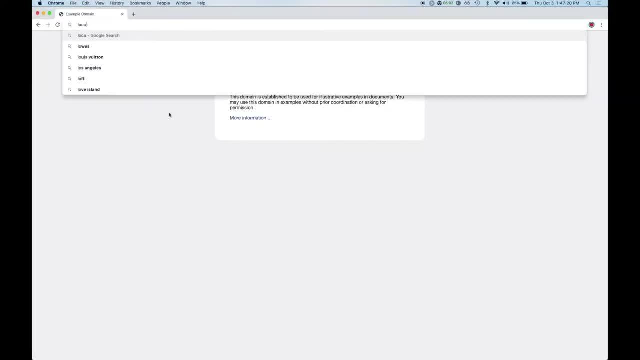 That'll be what shows up on the button. Okay, let me. let's run the server here. Just make sure that that worked. Okay, so if I log in- Cool, I have a send and a to now- cool, Okay, now let's implement the actual route. 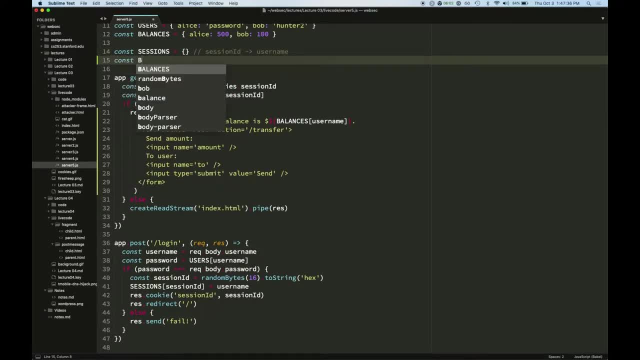 Actually, first of all, let's also add a balances table here. So we'll just give every user a different balance. So we'll go- this will be a map from username to balance, basically. So let's say that, oh wait, we already have that. 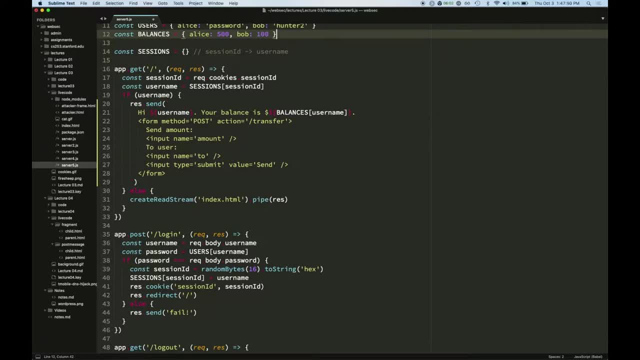 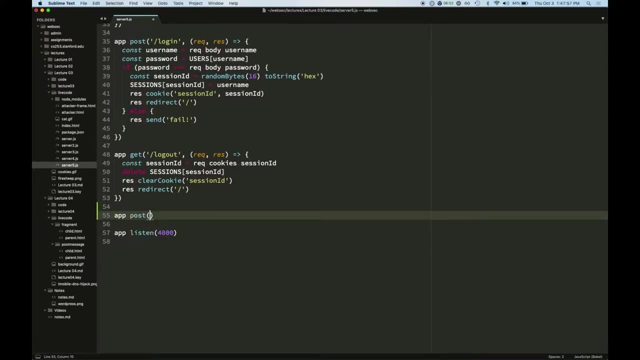 Oops, sorry about that. Yeah, okay, I'm being goofy. We already have balances, okay, So then now we just need to do transfer. That's okay, let's do that. So let's add a route called that's gonna be a post. 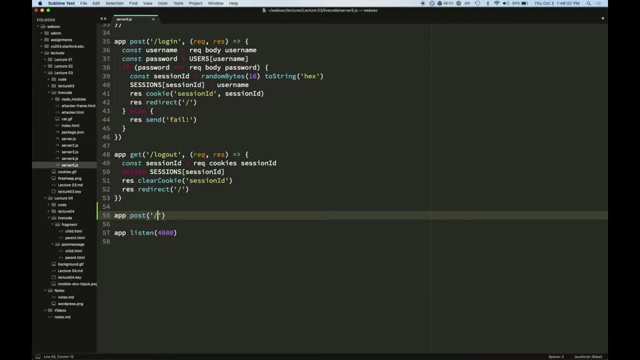 So nice thing about this being post is that the an attack is a post. Attacker can't use the image trick that we just looked at a second ago, because image tags cause a get request to get sent to the server, not a post. 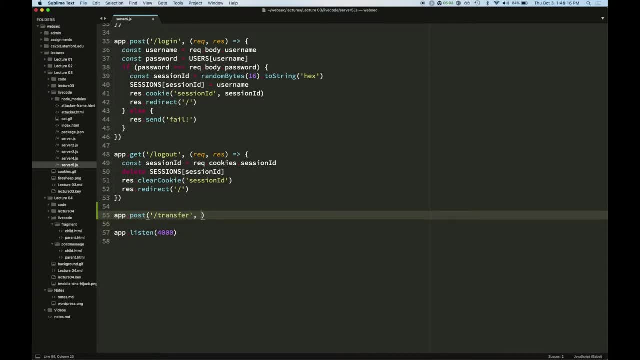 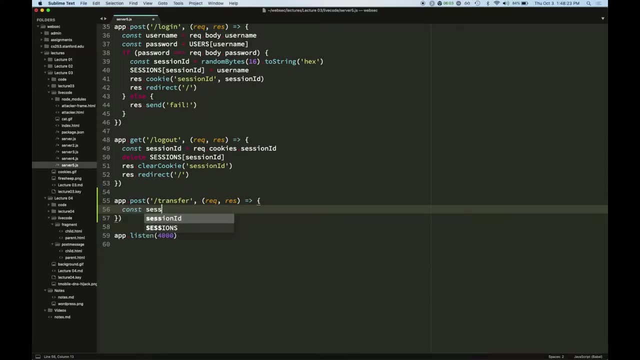 So let's, maybe that'll protect us, Maybe not, we'll see. Okay, so we're gonna say, when somebody posts to the transfer endpoint, let's get the session from their cookies. Okay, and then we'll look them up in the sessions table. 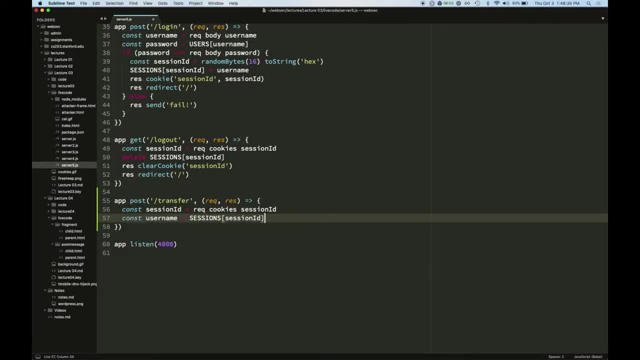 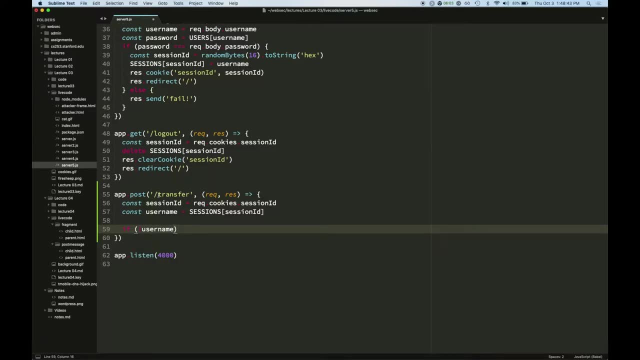 and make sure that they have okay. okay, So let's say, we have an active session, okay, So then this is either gonna be set or not set. So let's say, if it's not set, so in other words, the user sent a post request to transfer. 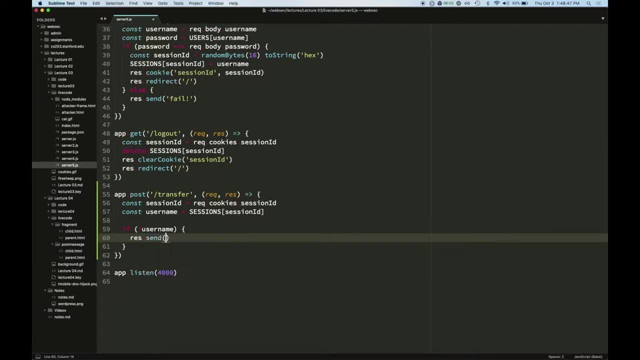 and they're not even logged in. well then, let's just tell them to go away, because that doesn't make sense. We can't have an unauthenticated user trying to transfer money, So let's just send them back the string fail and then do an early return. 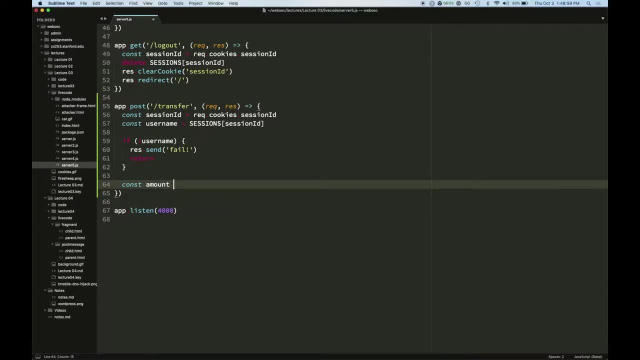 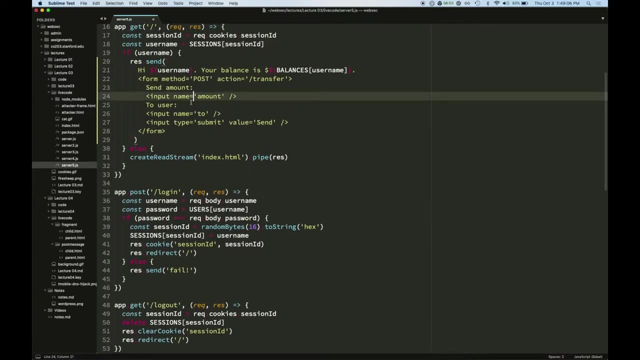 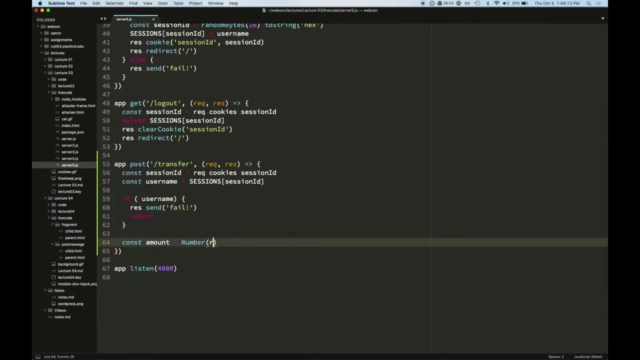 Okay, otherwise let's actually do the transfer. So what I'm gonna do here is I'm gonna so remember in the form here. we had two fields. we had amount and two that are being sent. So what I can do is I can get the amount from the body. 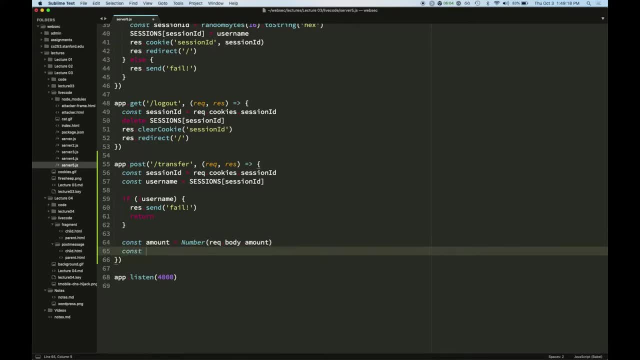 and it's gonna be a string, so I'm gonna convert it to a number And let's also get the two value as well. So two is gonna be the name of the account to send the money to, So that'll just be under rec body dot two. 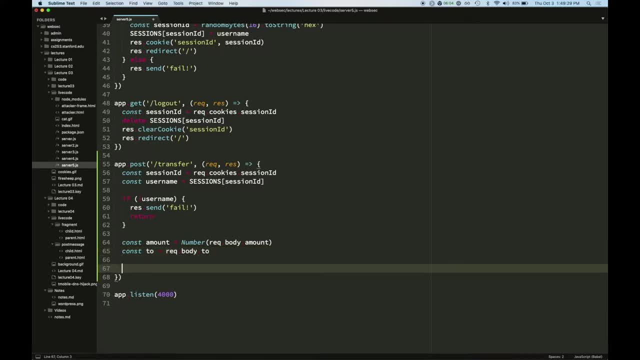 and that's already a string, so we don't need to convert it. Okay, so now we know what we need to actually do, so let's do it. So we're gonna take money from username, which is the logged in user. 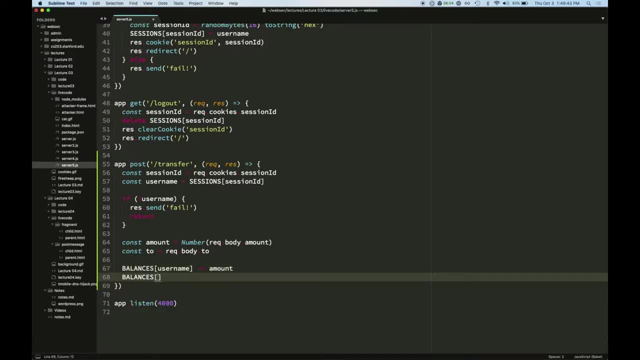 We're gonna decrement by amount and then we're gonna add the amount to the two account And then we're gonna- let's just redirect the user back to the homepage to finish things off. Okay, so this is just like a really simple. 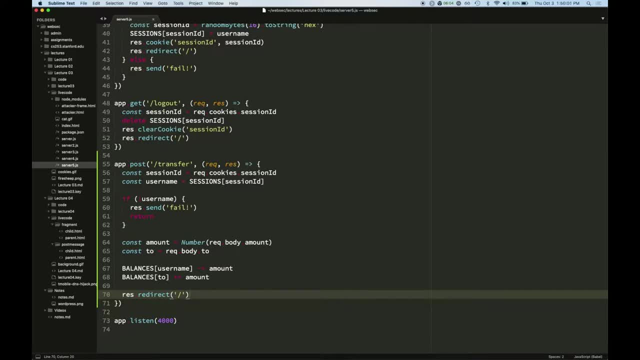 naive sort of transfer system. Probably in a real system we would wanna do some kind of transaction. So if the server crashed, like right after this line, that we wouldn't have something, that a state that doesn't make sense, but whatever. 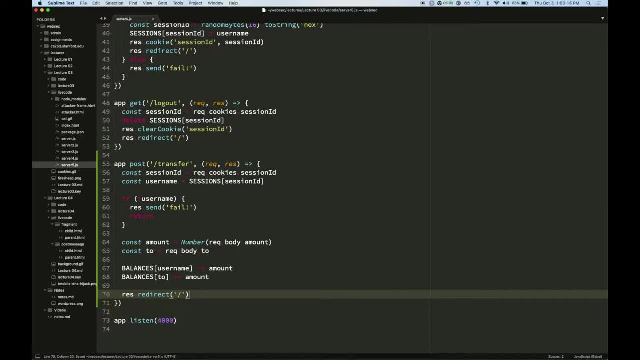 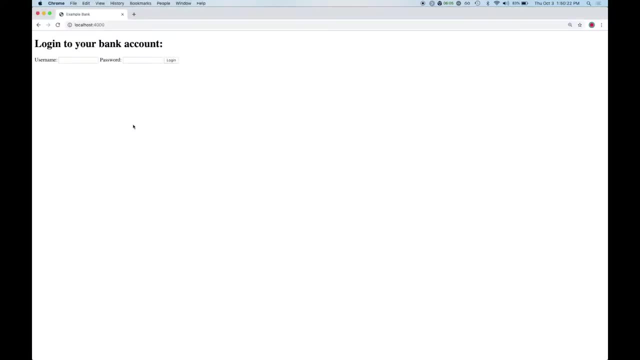 This is a simple example. Okay, cool, So now let's just test that it works really quick. So the server's already running. Oh yeah, I need to restart it. Okay, I'll do that. Okay, so refresh. Let's log in. 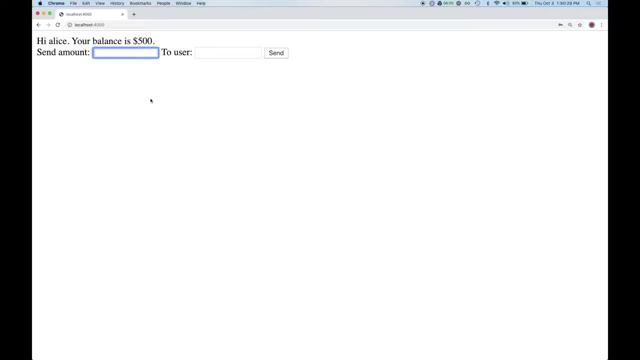 Okay, and so I have $500.. I think Bob had $100, right, So let's send $100 to Bob. Cool, okay, Not only like log out and just make sure Bob got it, just to make sure we don't have any bugs. 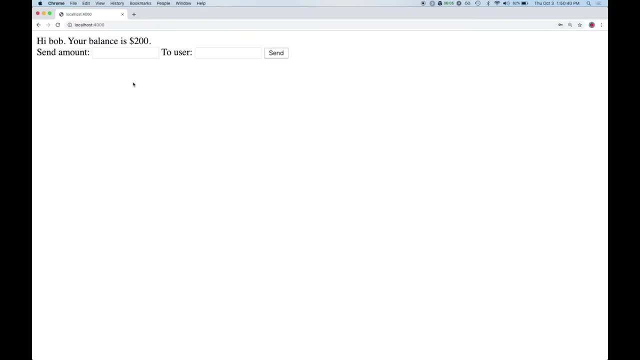 So Bob and then Hunter. two. Okay, Bob has $200 now, So it works cool, Okay, so there's a problem with this approach. This is even though we switched to using post request for this endpoint, an attack site can still cause a request. 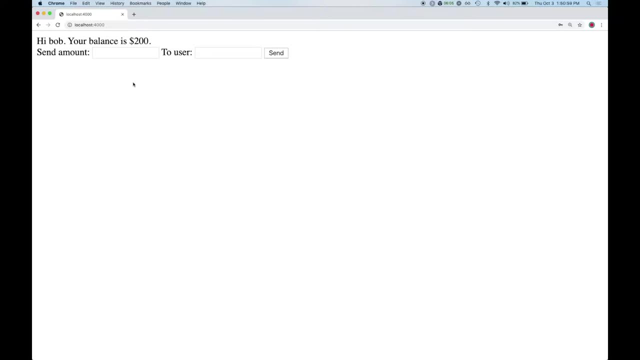 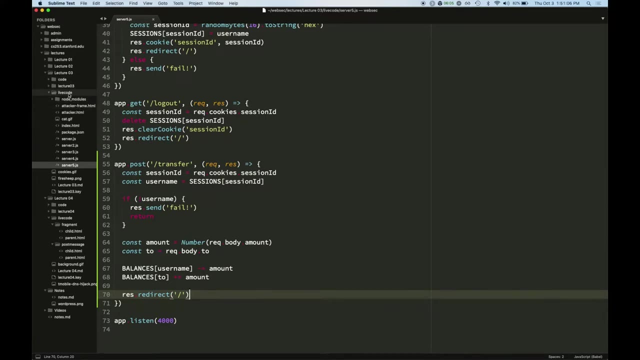 to get sent to the server, that the server will interpret as a request to get sent to the server. So that is valid. So let's see how to do that. So what I'm gonna do is I'm going to make- let's make, just make- another file here called attacker. 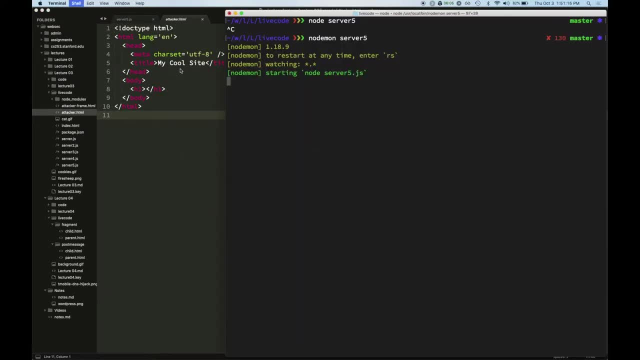 Okay, let's do that. So I have this file here called attacker, And what I'll do is I'll start a second server here, And this is just simulating a completely different website, right? So what I'm gonna do is just start up a server. 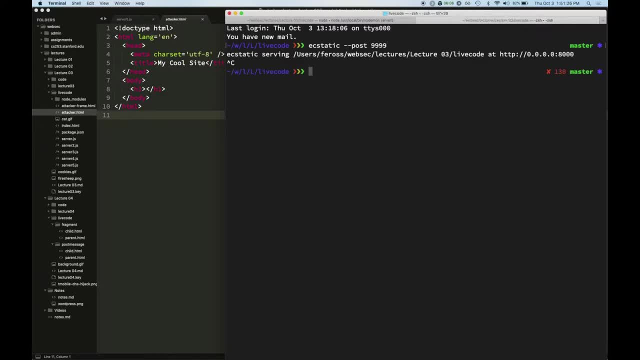 on port 9999, which looks like an evil port number. So that should help us know which is the attacker and which is the target. Okay, so, okay, so cool. So let's see. what should the attacker do? So well, let's, let's see. 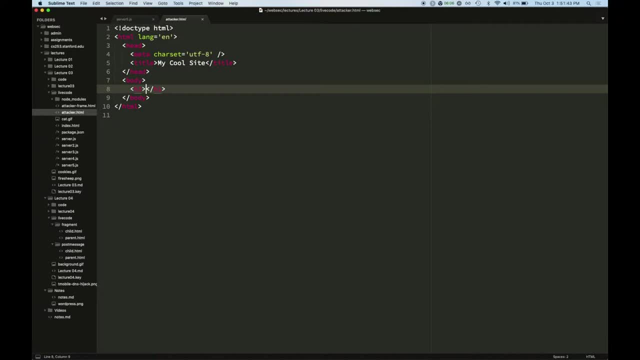 So let's make a page where the page looks kind of innocent, So somebody might come, you know, come to it and then be sort of browsing around, maybe looking at cat pictures or something, and not realize that this request is being fired off in the background. 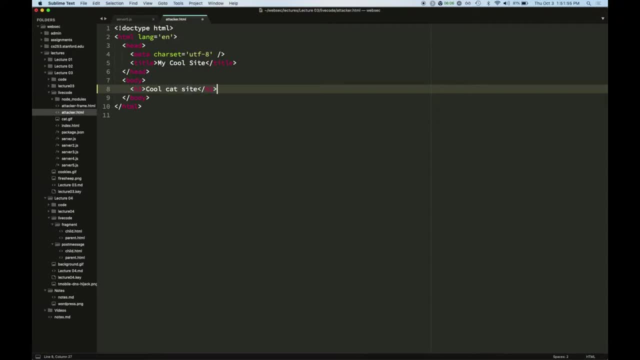 So let's make it look kind of innocent. So cool cat site. And then I have a cat. I already downloaded catgif Cool, so that'll keep them distracted. Meanwhile, what we're gonna do here is I'm gonna go to the code. 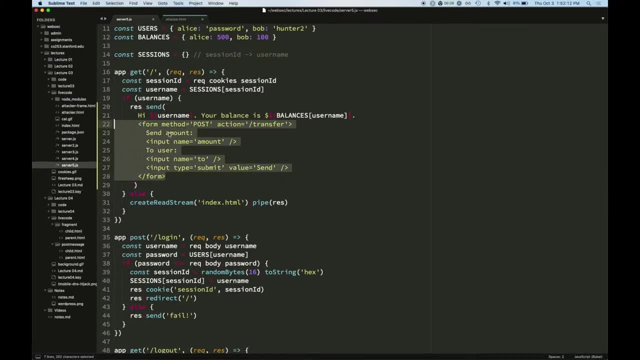 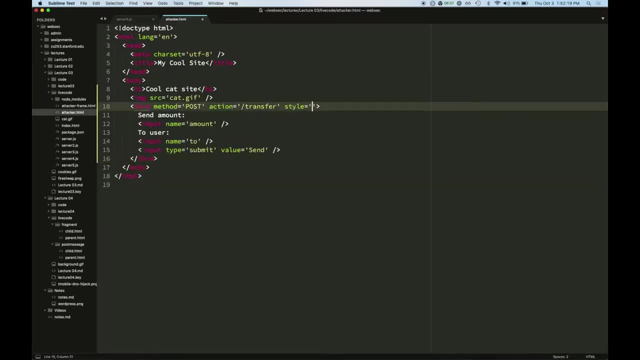 So remember this code here, this form here, that includes the sort of amount and the two and all this. Let's just copy that right there, right directly here into the attack site And we can go ahead and hide it with style display none. 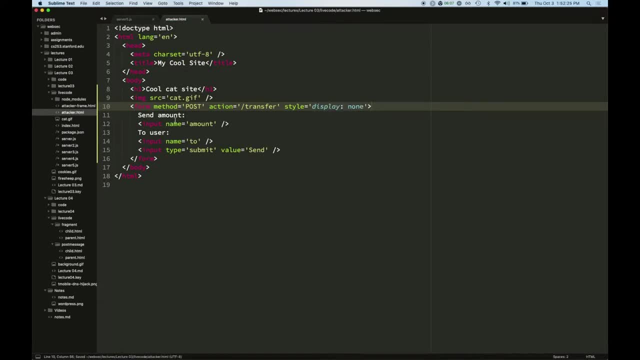 So users are not gonna see that this form is even here, right, And we can remove this text. This text doesn't do anything. Let's just clean it up a little bit. So we have the form fields here And one of the things that we can do here. 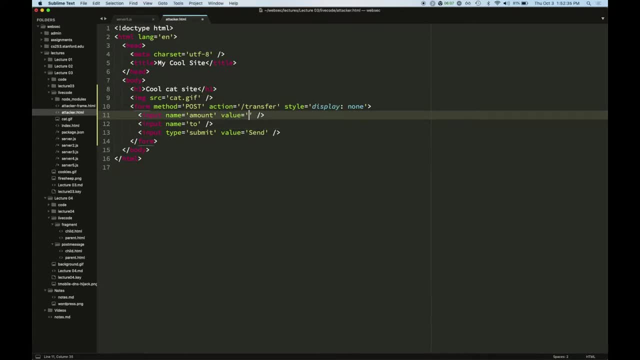 one thing we can do is we can just put a value into it, so it's sort of pre-filled with the value that we want. So let's say we wanna send $100.. Let's say, let's see, Alice is the attacker here. 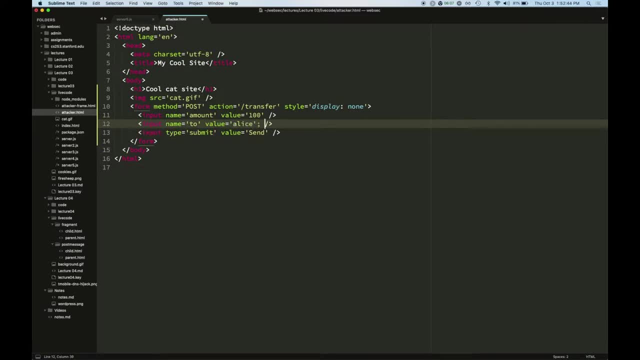 So we'll send $100 to Alice, Cool, and then we need to actually submit this form. Oh yeah, one thing also. one other thing we need to do here is the URL is wrong, So we're on the attacker's site. 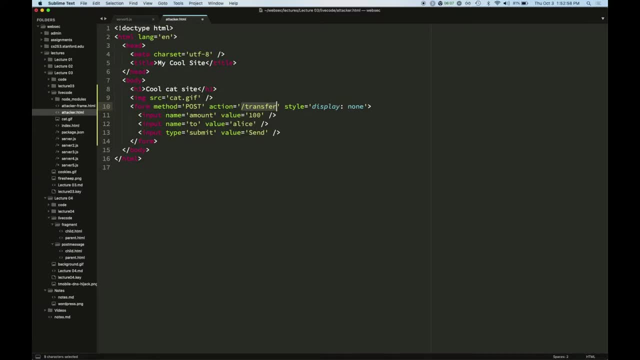 So it's not enough to sort of submit this form to slash transfer. That would actually submit it to the attacker's own site, which isn't gonna do anything. We're trying to sort of, we're trying to forge a request to the actual target site. 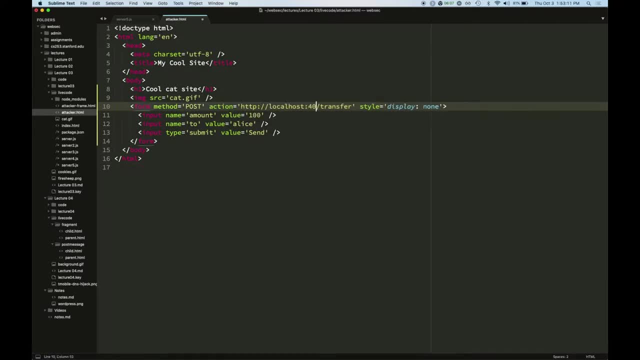 So let's actually put in the URL of the target here, which is localhost 4000.. So we're on localhost 9999, and we're gonna fire off a request to localhost 4000 slash transfer. Okay, so now it's actually fired off. 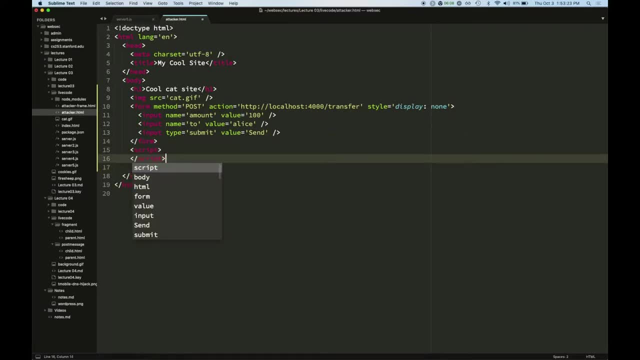 So we do script. We'll just put a script in here And then this is like kind of bad code style, but it gets the job done. So there's this sort of global called documentforms which just gives you, gives you an array of all the forms on the page. 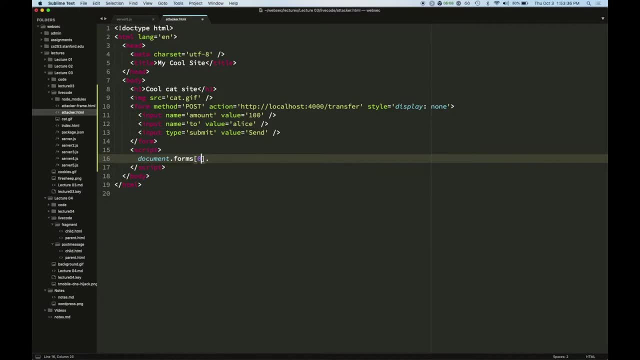 And so we'll just let's use that. The reason why this is kind of bad is because if the form order sort of changes, then you're indexing, you're gonna get a different form, but we only have one form here, so it's fine. 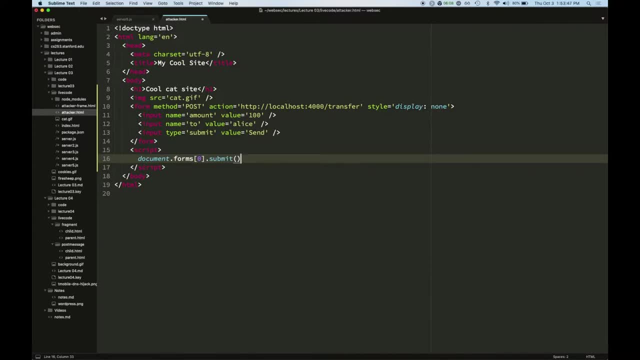 And then we'll just call submit on the form, So that actually basically clicks the submit button on behalf of the user, effectively, right? So there's one problem with this right now, as I've written it, which is that the user is gonna come here. 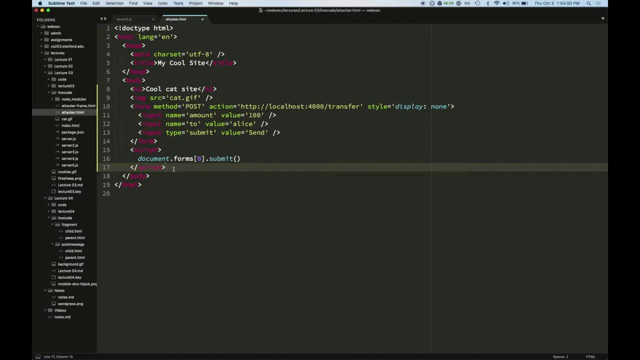 and sure they're not gonna see that this form is here because we hid it. But one thing that's bad is that when you submit a form, the sort of default behavior of the browser is to actually send you to a new page. So they're gonna get kicked off of the cat page. 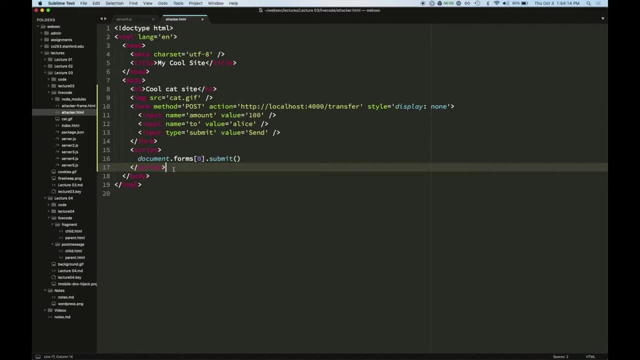 that they're on, which will be kind of fishy. So let's clean this up just a little bit. So what we can do is we can take the form here and just we'll copy it out and put it into a different file called attackerframehtml. 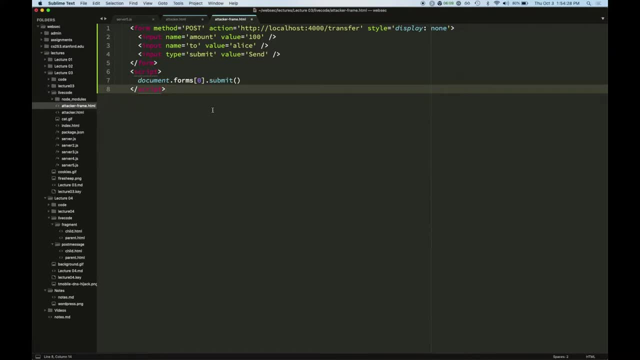 Can you see that right there? Yeah, so I just have a separate file and we're just gonna paste the same exact code in here, And then what we're gonna do is just include a frame that points to that file. And so what does this accomplish? 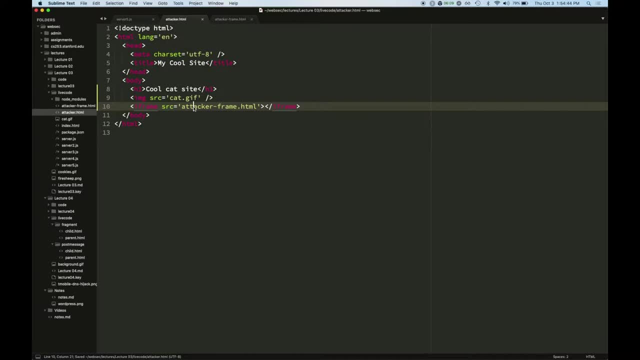 Well, what this accomplishes is that now this frame, it's gonna load up that HTML Here. actually I'll just remove the style and we can see it in action. So, and actually I'll comment out the submit button for a sec so we can just see what this looks like. 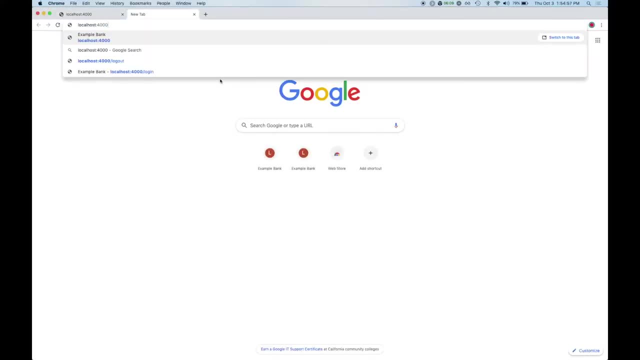 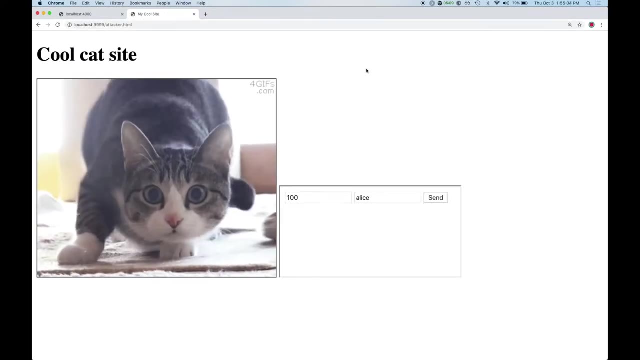 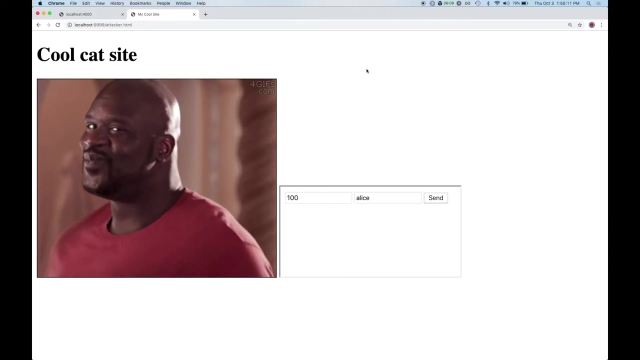 Okay, so let me go to the attacker's site. oops, Okay, okay. so we have our distraction and then we have our frame, And so what's cool about this is now, if I click send, then it's gonna navigate this frame. 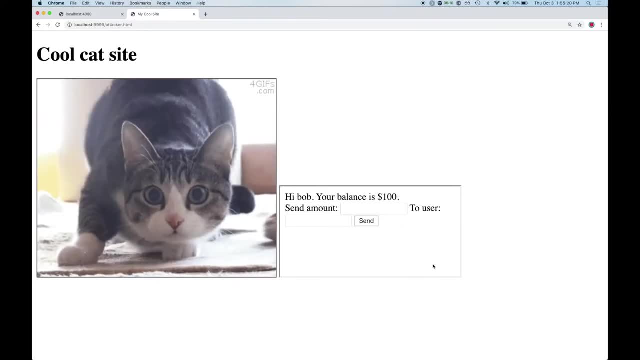 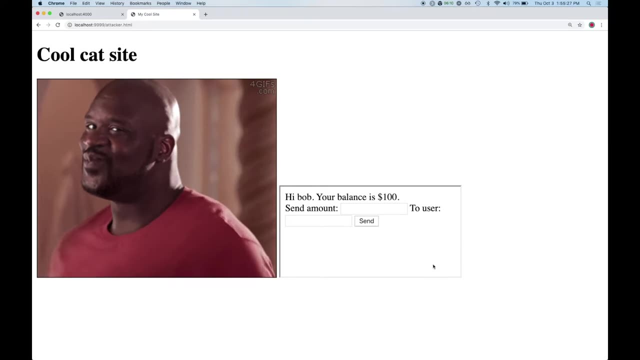 but it's not gonna navigate the entire page. So that's the idea behind that. It just sort of cleans up the attack and makes it a little bit less noticeable. So okay, so let's see here. So now let's actually just sort of do it completely. 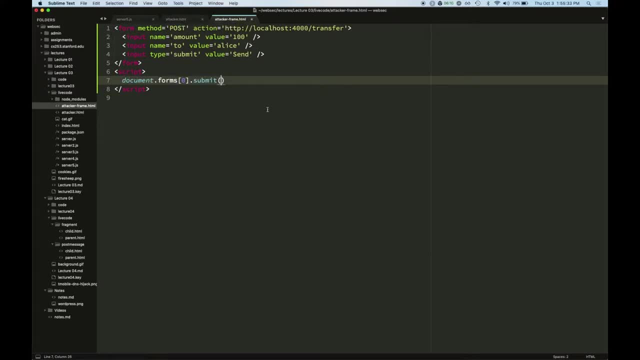 So we'll go here. We'll go back to the. so I actually wanna automatically submit the form again, and then I'm gonna go here and I'm just gonna hide this frame with the same CSS as before: display none. Okay. so now, if I so, let's see here: 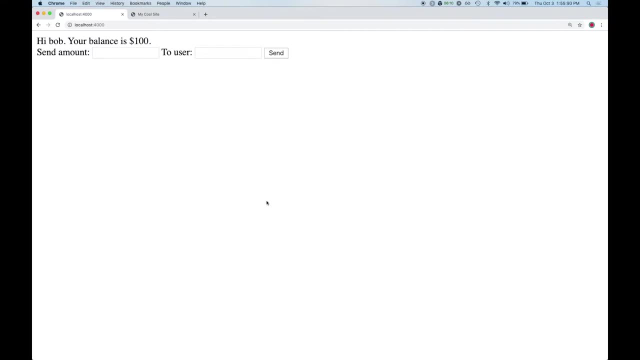 So we have to start off on. so the way this works is: the user has to be logged into, the user has to be logged into the bank. So we just check here. we're logged in, right, We're logged in as Bob, so that's great. 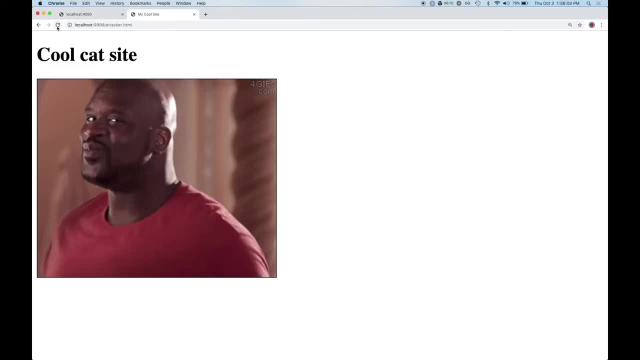 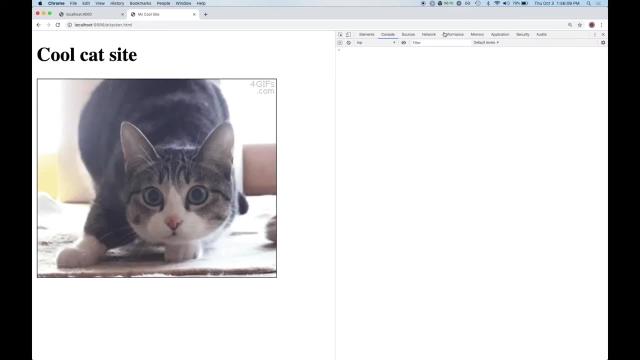 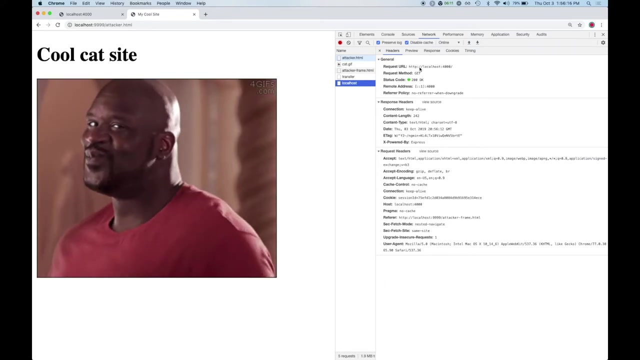 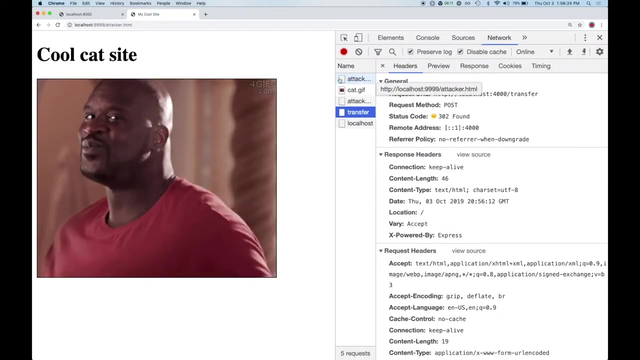 So now, if I go to this site and I actually refresh, let's go back now and check my balance. Wait, that shouldn't have happened. What happened here? So we sent a request to localhost 4000 slash transfer and it contains amount 102.. 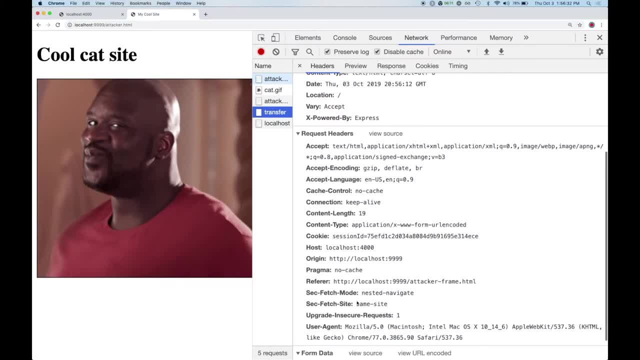 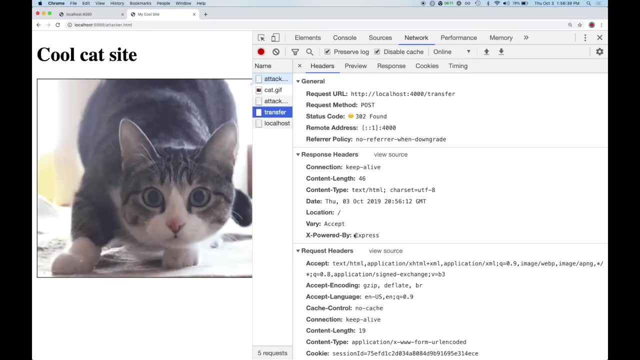 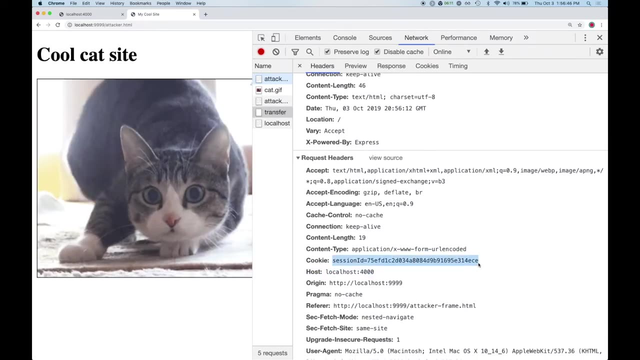 Okay, So I'm gonna go back to Alice and let's see here What's the reason why this isn't working. So the server, so the request contained the session ID, which is great. That means the server should accept it, right. 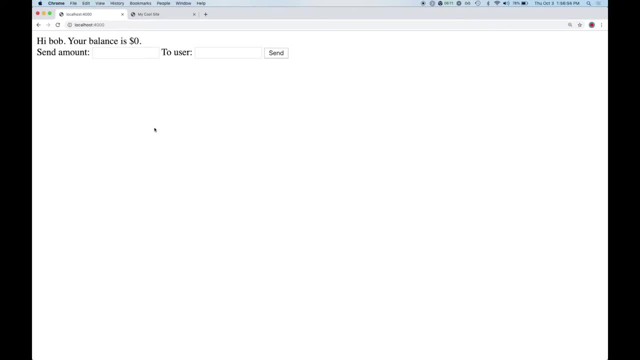 Oh there, it did. okay, I just needed to refresh again. Okay, anyway, there we go. So it looks like it worked. So let's go ahead and refresh the page one more time and then okay, So the bank has other problems. 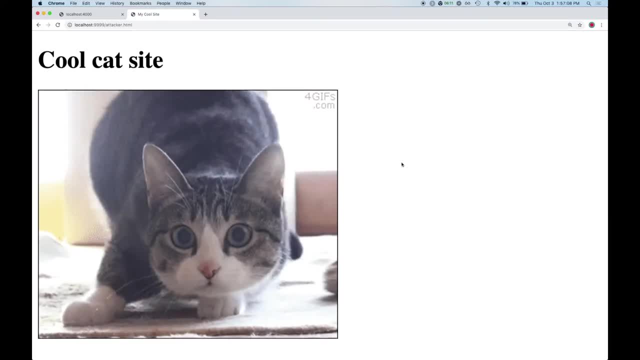 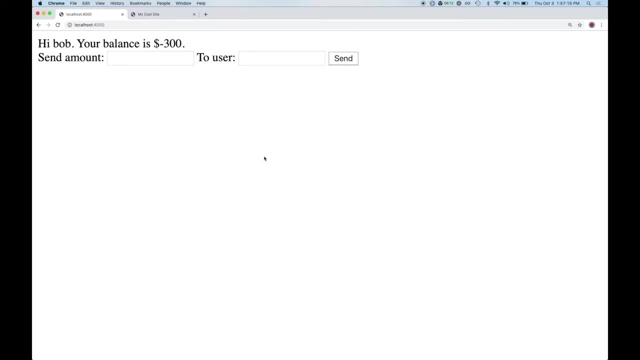 But we can see here that. so every time I come to this site, I don't see anything going on, but every time I refresh, we're gonna keep firing off these requests. So what's the lesson here? The lesson is that forms are also allowed. 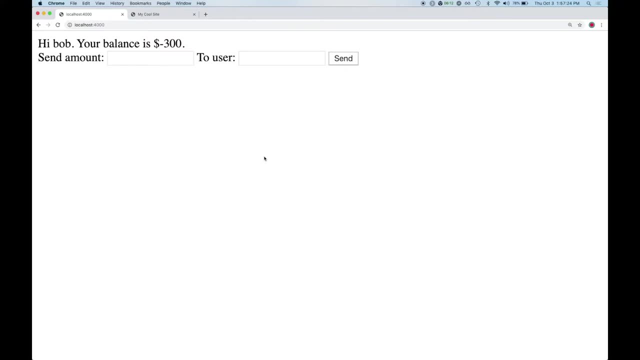 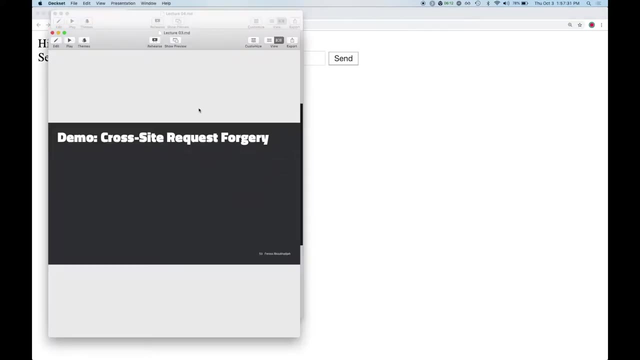 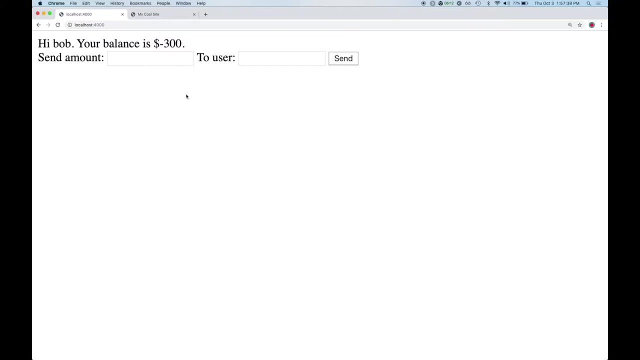 to be submitted from one site to another and we have to think about how to defend against this. This seems kind of like a problem, So cool. any questions about this? Yeah, go ahead. Do you just have like Chrome security settings disabled? 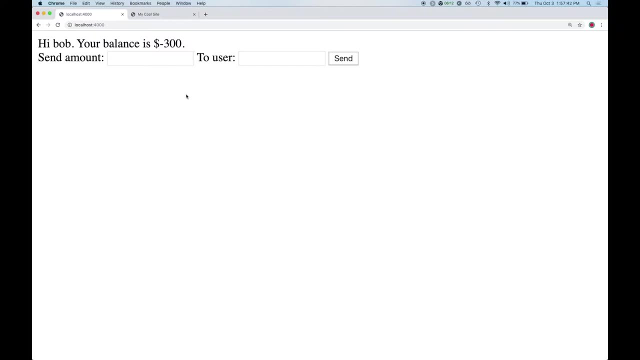 or is Chrome actually just like allowed this? This is always allowed. yeah, Oh, wow, Yeah, this is always allowed. So this is actually this is. the crazy thing about this is that a site has to sort of actively go out of its way. 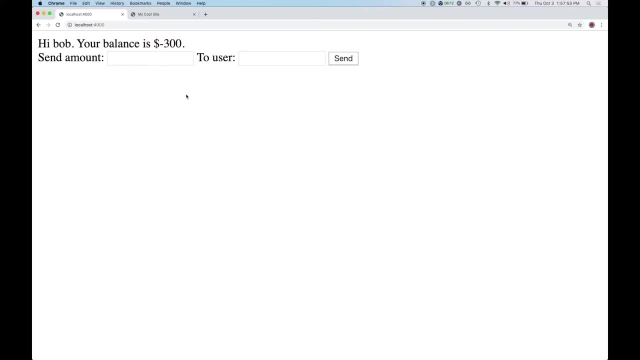 to implement a defense against this, because the defaults are kind of bad when it comes to this. yeah, That's just a sort of unfortunately, It's just an unfortunate reality with the web. yeah, Mm-hmm, Do people, let's say, for like Facebook? 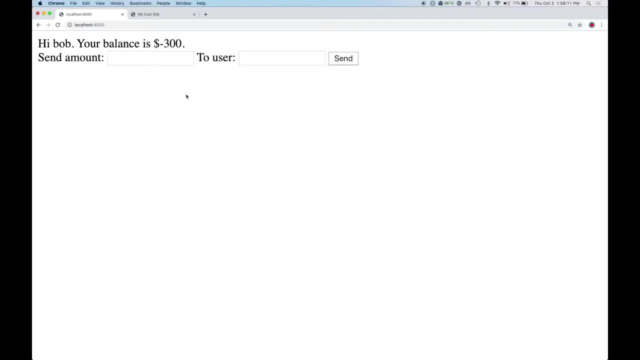 does Facebook use the form for login or, like they, use something else to, like, facilitate login? Do sites actually legitimately use forms? Use forms like this? yeah, Yeah, they do. they're really, really common still. yeah, So typically a site will use a form. 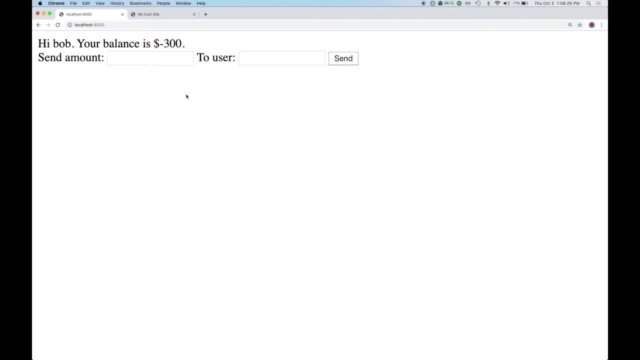 and then it will. it might do something fancier on top of the form, so it might sort of detect when the user clicks the site. will you know? it might detect when the user clicks the submit button and with JavaScript. 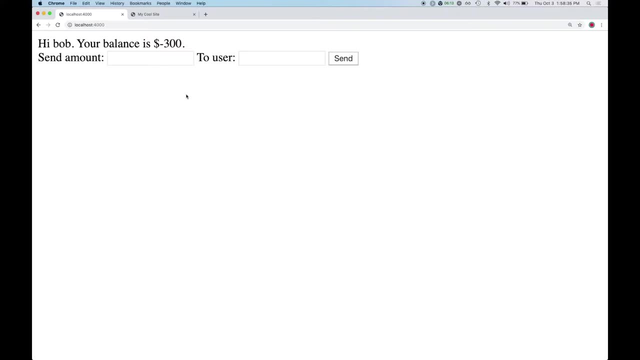 it'll sort of intercept that with, you know, with its own JavaScript on its own site, which it's allowed to do, and then it might sort of fire off a login request in the background without the page sort of completely refreshing, in order to improve the user experience. 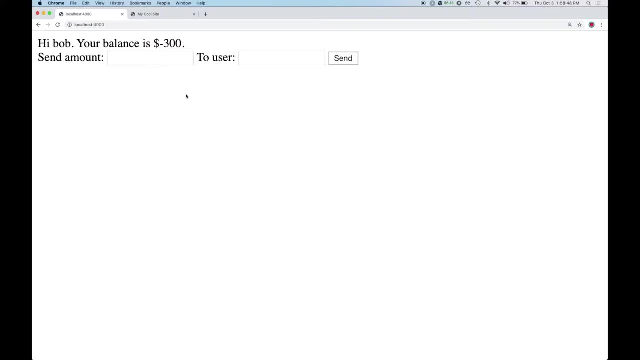 But if JavaScript is turned off, then typically, like, the form will just fall back to being a normal HTML form, which will still work, but it will cause this sort of page flash kind of thing. So people often, might you know, do this for user experience reasons. 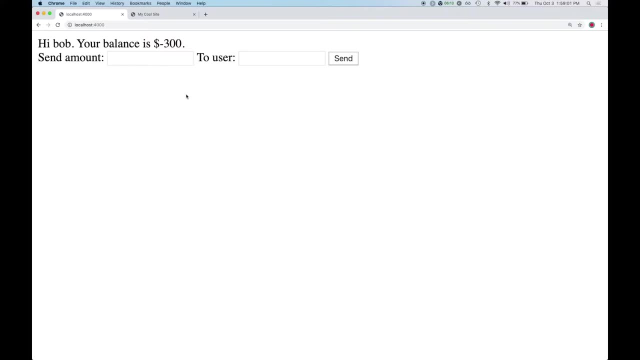 They don't want to. you know sort of. you know have the whole document sort of change when you log in, if that makes sense, Yeah, But yeah, forms are still really common. Yeah, Cool, okay, so let's keep going. 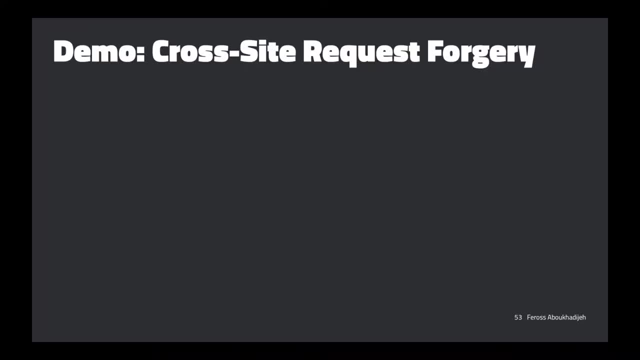 So I'll talk about a defense for this, like later, but I just wanna- oh yeah, actually, you know I'll mention one right now, but it's actually not a complete solution. So the one I'm gonna mention right now. 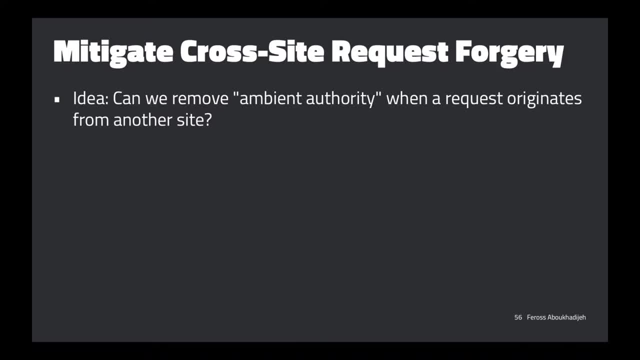 is sort of the idea here is: is there some way that we can remove this sort of ambient, this ambient authority that the cookie is providing when we know that the request is coming from not our site, from another site? Because if we could do that, it seems like it would solve the problem, right? What if we could just say: hey, like this cookie browser. please don't automatically attach it when you're sending requests to my server, unless that request originates from a page that's also from my server, right? 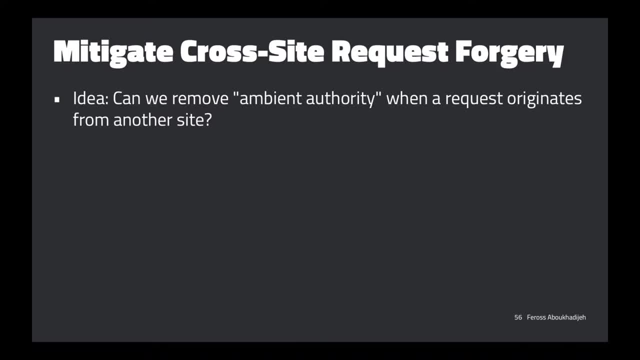 That seems like it would solve the problem. Well, the next point I wanna talk about is basically, the attacker could now do the same thing that we just did, but the browser would say: wait a minute. when I was given this cookie, I was told not to attach it to a request. 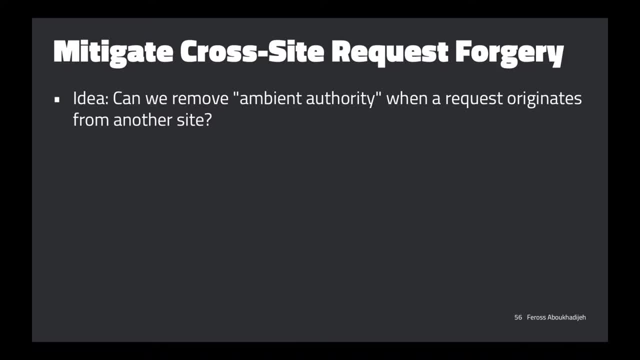 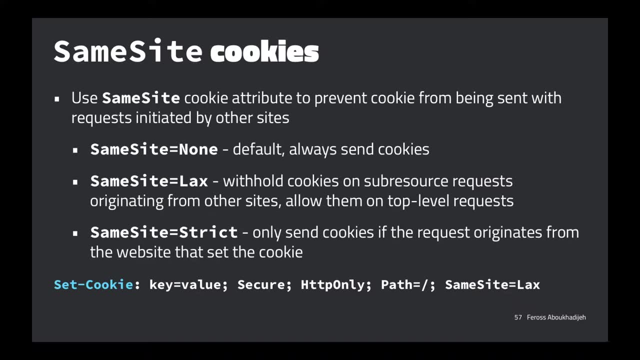 to this server because it's not coming from that same server. Does that make sense? Okay, so let's get into how that actually works. So this is another cookie attribute called same site. So if you attach this, you can sort of solve this problem. 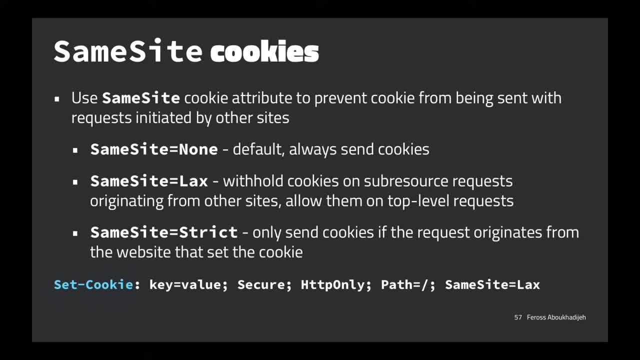 For the most part So. attribute that prevents the cookie from being sent with requests that were initiated by other sites. so there's three settings. uh, the default is none. so it's sort of just the default browser behavior is to always just send the cookies along if they um match the request. but you can do um lax, which. 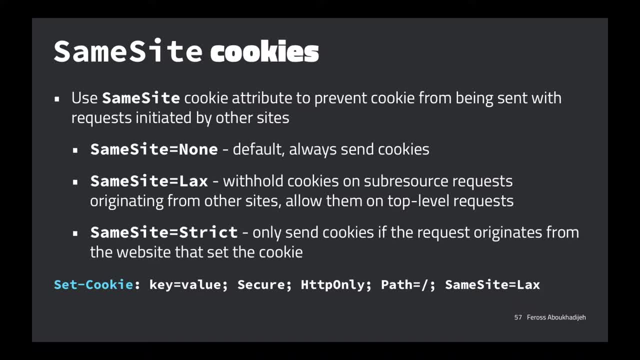 is: uh, basically, what it'll do is it'll say: um, anything that's a sub resource request, so that's like an image embedded in a page or a form being submitted from a page or anything like that. any request that's sort of coming from within a page, that's called a sub resource request. 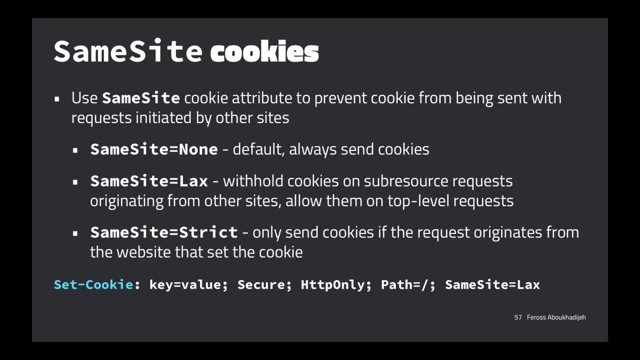 that's different than a like i would call. the opposite of that would be like a top level navigation. that would be if your browser actually goes to a url that you can see in the url bar. that's, that's a. that's a different thing. so, for just for the sub resource requests, 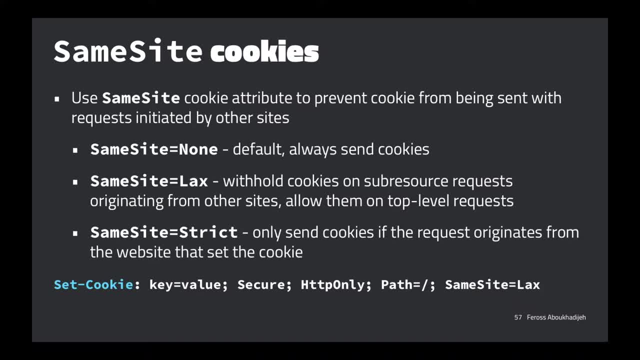 um, if those are originating from another site, uh, we, we want to prevent those, prevent the cookies from being attached. um, but for top level requests, uh, we want to let the cookies be attached. so this setting is, is, is, is, um, would stop the problem that we, uh, that we just had um. 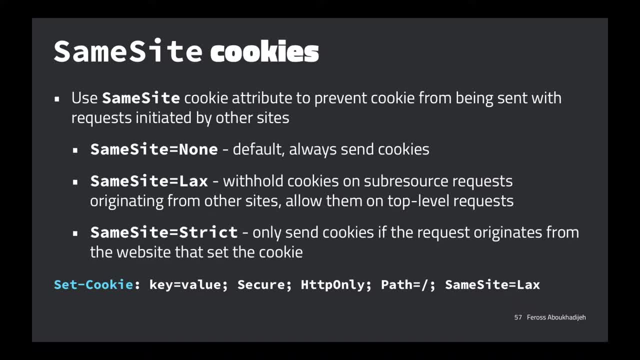 if you want to go a step further- um, you're extremely paranoid- you can go with the strict mode and what this says is: uh, just never send cookies if, uh, if the um the user was was, uh, if the user was sent to this site like another site, this is really aggressive. so, in particular, it doesn't even send cookies on top. 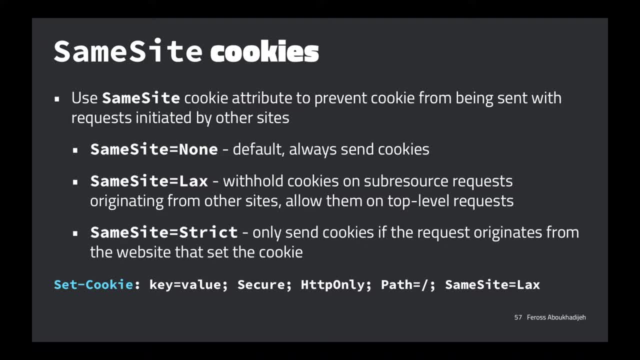 level requests. so what does this mean? this means that if, if i have a blog post and i'm talking about how much i love my bank, right- which i would never write but say i did um- i could link to that bank's home page and the user, if the user clicks that link, the whole browser is going to go to this new. 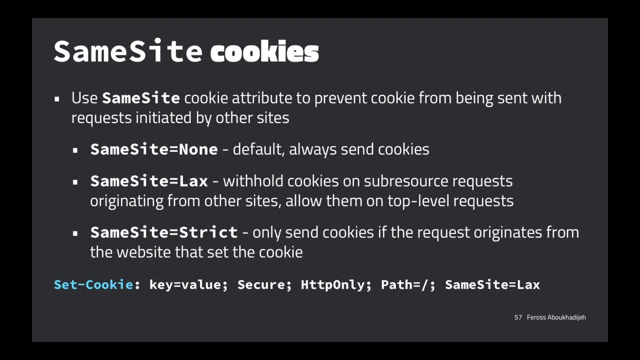 page right, but with the strict setting, the browser is going to say that request actually originated from faras's blog and so don't attach the cookie. um, so, even though that's a kind of a completely innocent request, i'm just sending them to the home page. the fact that it originated from from another site. um, even even at the top level, like 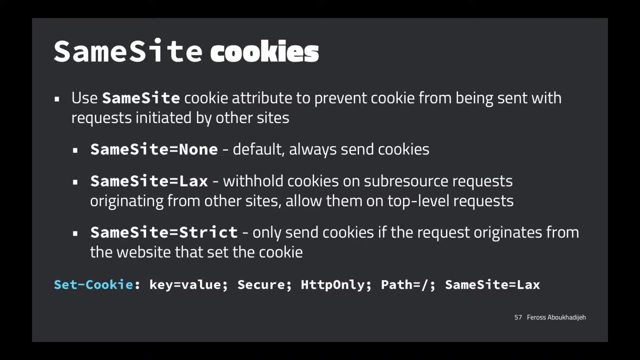 it's not a malicious request. it's literally just a url that the user themselves could have. could have, uh, you know, pasted into their url bar. that's not going to send the cookies. this can be a little bit confusing, you know, if you're, if you're, logged into a social media site and then you click a link. 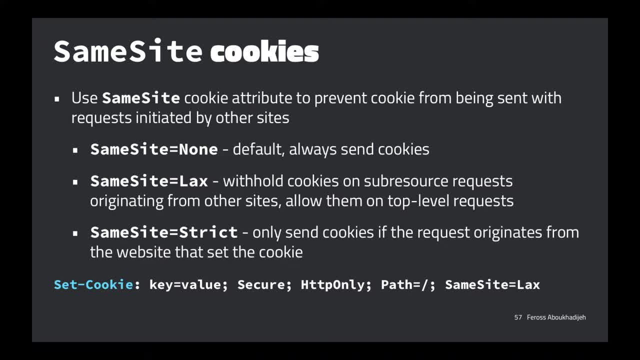 and they have this setting, then you're going to click the link and you might be logged in in some other tabs, but when you click a link from someone's blog, you'll end up not logged in in that. so this is actually kind of almost too aggressive, i would say. but if you're really into, you know if 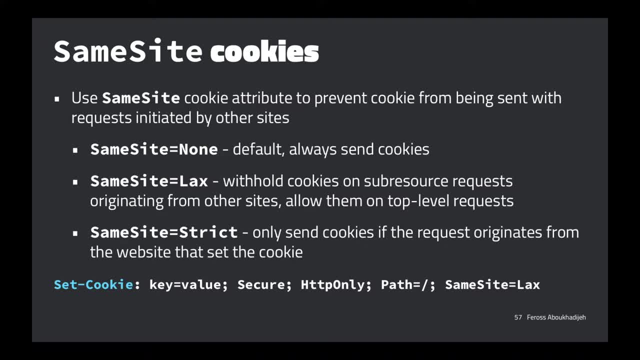 you're doing something in finance. maybe you want to, you want to do this, but this is actually probably the best setting for for the average, the average site. so understand if i create my frame and set document that location on that iframe to a site like that. get request is not a sub resource. that. 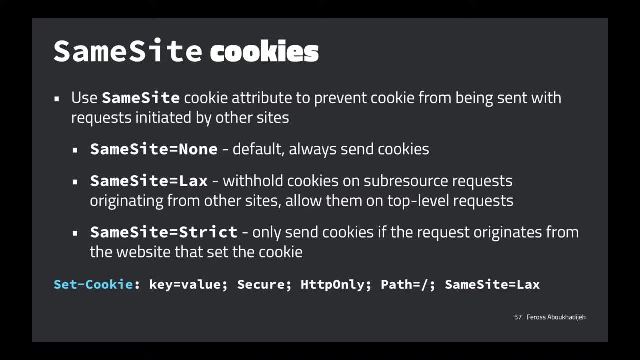 is. that is because an iframe is considered a sub resource as well. yeah, even though it's sort of it's, i guess it's the top level of its own frame, but it's still a sub resource. yeah, yeah, so lax covers. like most of the cases, it sounds bad because you're like: oh yeah, i'm like my. 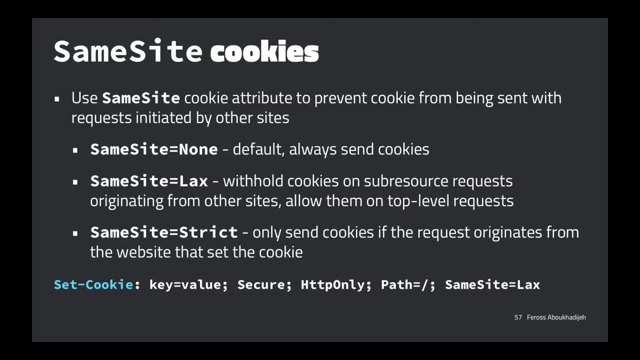 security is lax, but like it's it's actually. it's actually much better than none, uh, cool. so so now this is what our cookie line looks like. it's getting complicated, um, but yeah, any questions about same site? yeah, so if instead the default was lax, what are some use cases that would break? 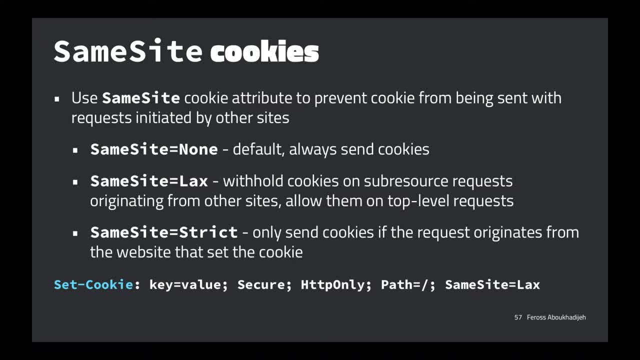 oh, if they just made the default lax, yeah, or like, are there any legitimate reasons why you wouldn't want that? uh, so yeah, that's a great, it's a great question, so it, uh, it would break some use cases. so, like one i can think about the top of my head is: have you ever been on a site and 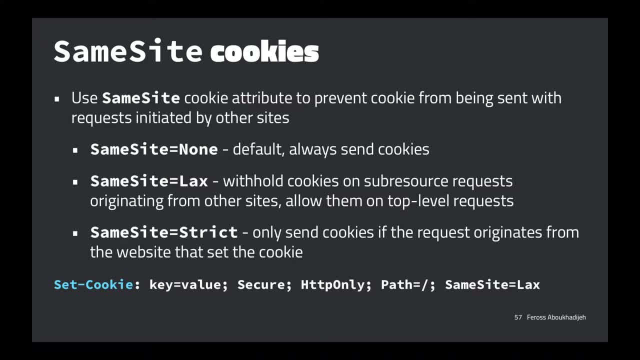 you see, like uh, comments by facebook, uh, so, uh, so that little box that's an iframe, right, and that that's going to make a request to, to load this little comment box, um, and because if they turned on same site lax, what would happen is, um, the cookies for that request would not actually get. 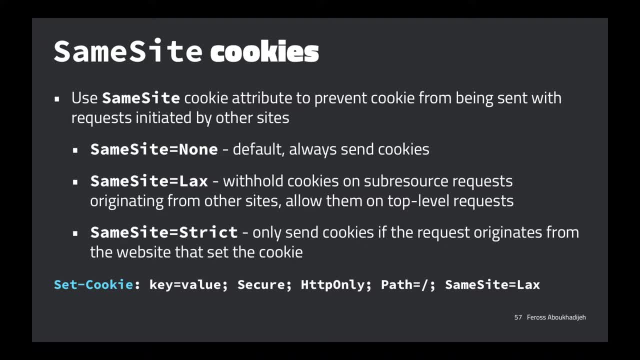 attached and it wouldn't be able to show you like your avatar there and have a little box that ready for you to type your comment in, like you wouldn't be logged into the comment box. basically it would comment box. you'd have to type in your username, password for for facebook and also your comments. 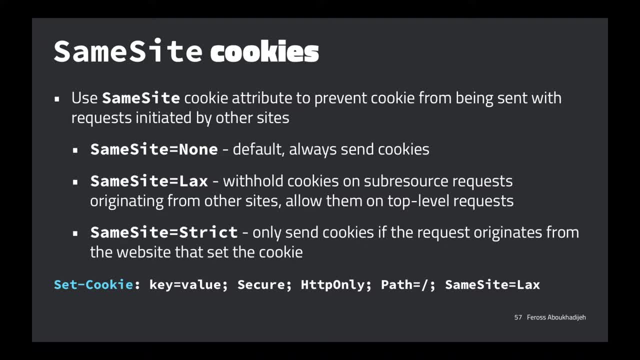 in order to make that that work. so that's a little annoying, um, uh, yeah, that's one thing. another, another, another thing is like um, ad tracking. um, they don't want to turn this on at all because, uh, they basically attach cookies to every request for an ad so they can know that it's you, um, and. 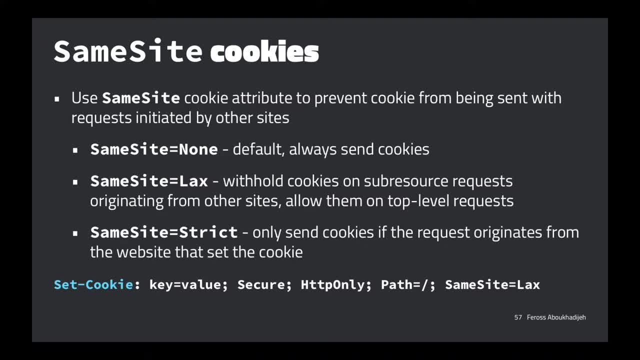 they wouldn't. you know they're very happy to have that tracking information attached to every request, so they would be. they would be unhappy with this change, probably, um, but yeah, i think those are. those are two, two, two use cases that would break um, but actually you know the thing. 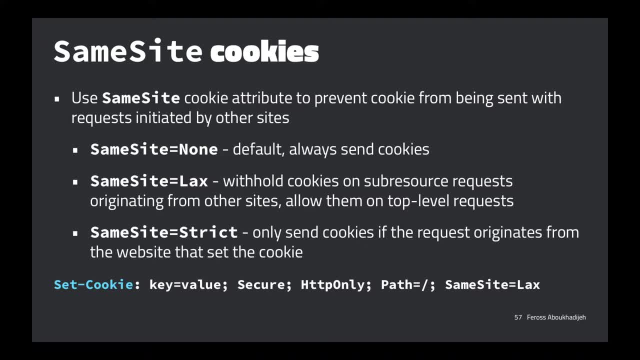 that the thing is interesting is these aren't actually that good of use case, like, like people are sort of the the threat of of of like this attack. plus, like people's concerns about tracking are actually sort of changing the the calculus around this and um, there's actually now a proposal. 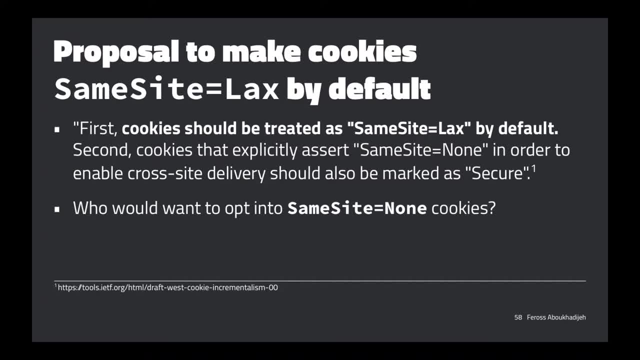 by google to just make same site equals lax be the default for all browsers. um, so this is what it says. first cookie should be treated as: yeah, this is basically a snippet i pulled out of the spec post, so cookies should be treated as same site equals lax by default. uh. second cookies that 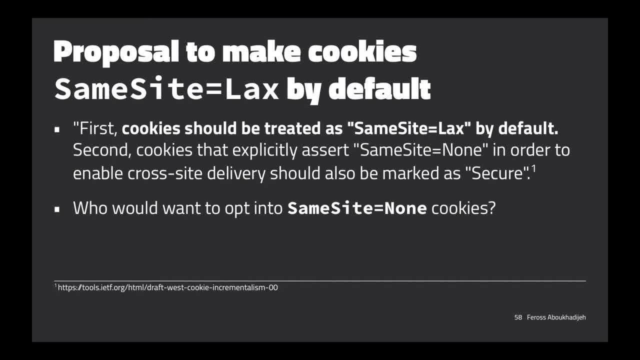 explicitly assert: uh. same set equals none. um, uh should also be marked as secure. oh, oh, yeah, so, so, um, the first part is what i already said. it's basically that lax would become the default. but the second part is kind of interesting. this is um sort of google's uh attempt to solve uh like. 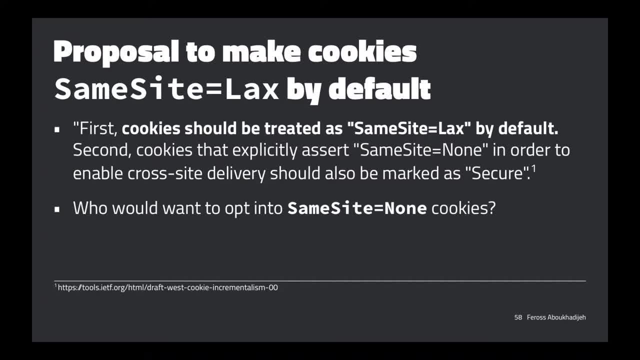 ad tracking, which is uh, uh to their idea is so. so if this is the default, if lax is the default, then the only people who are doing same side equals are probably ad people, or or, um, uh, that, yeah, maybe something kind of a little bit more sketch. 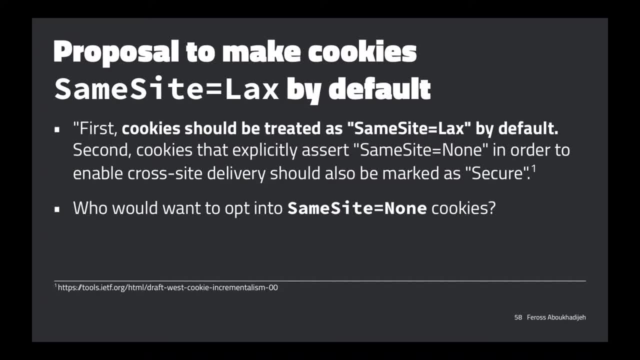 so let's, let's, let's, uh, force all those cookies to be marked as secure. at the very least. they're over that. that tracking data is going over https and uh people can't passively observe it. uh, if that wasn't true, then you know, in theory, these, these, these requests would have this tracking. 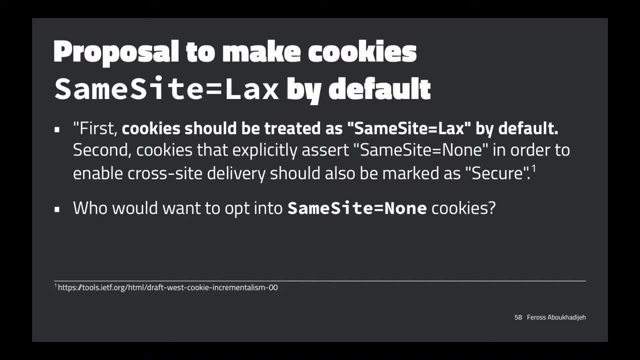 data attached that anyone on the network, like your isp or the nsa, could read and then learn that it's you right, because, because this data is being sent in the clear. so this is sort of like a slightly better situation. but yeah, so this is uh, this is um, this is a kind of a good improvement, i think. 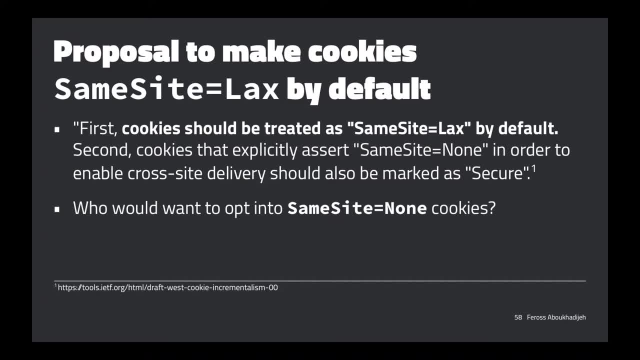 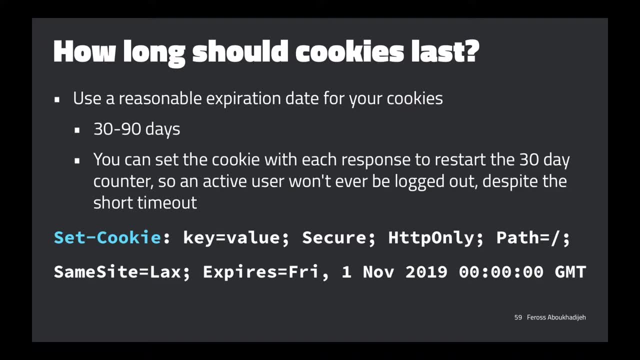 cool, any questions? so i think this is going to roll out soon in chrome, which is kind of kind of exciting, okay, so one last, uh, one last thing. so how long should you set your cookies for? i was, uh, i mentioned last time, like 30 days is probably sufficient, because you can sort of reset the. 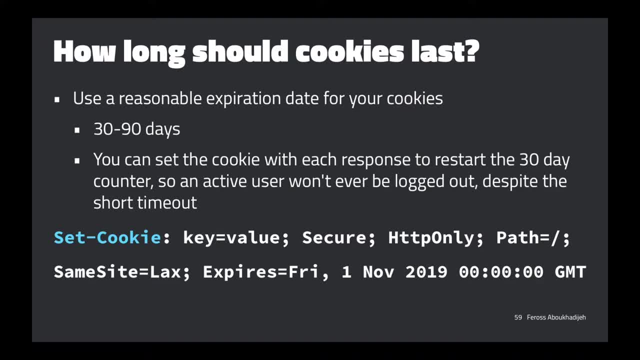 counter every time the user comes to your page by sending them this set cookie header again and it will sort of add: it'll, it'll be 30 days from that moment on. so now, if we add that in, this is sort of what our cookie is looking like. um and um. so now, um, what i want to do is actually want to go in now to our 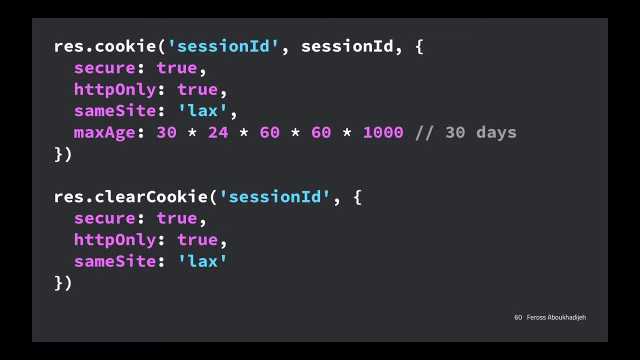 server and i want to add the all these options that we talked about. so express has these nice, this nice sort of api for enabling all these features on our cookies, and so let's go ahead and add that and see if it fixes. that fixes the attack. but one thing to note is when you actually 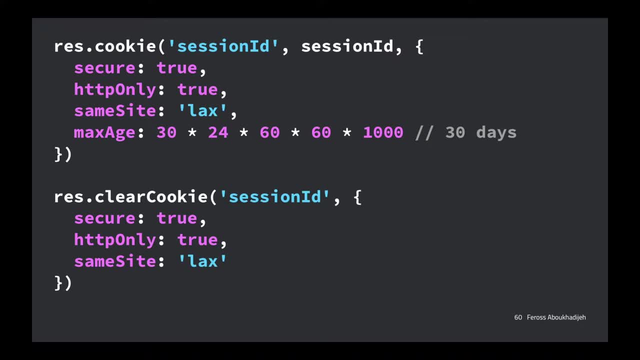 go to clear your cookies. uh, you remember how we we used to write a lot of work on the server. When we do that again, we give the cookie with the same name and then we tell it that it expires in the past, and then the browser clears it. 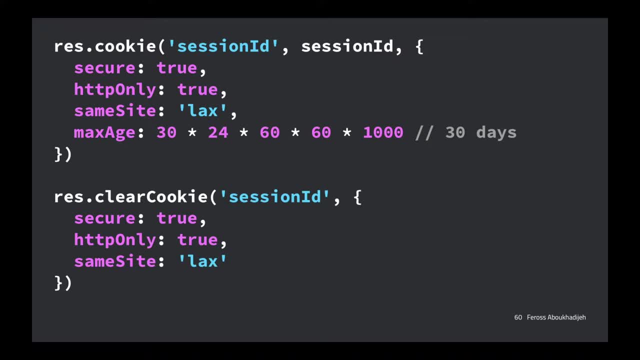 We have to make sure that all the other attributes are also exactly the same as when it was set. It's a little bit janky because if you don't do this, the browser thinks that it's actually a separate cookie with the same name. 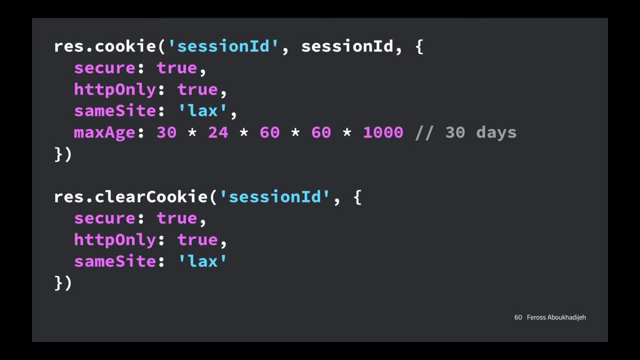 And you can actually have multiple cookies with the same name that have different attributes. So, anyway, you have to just make sure these are equivalent, except for the max age, because that's going to be set to the past, so we don't have to pass that in. 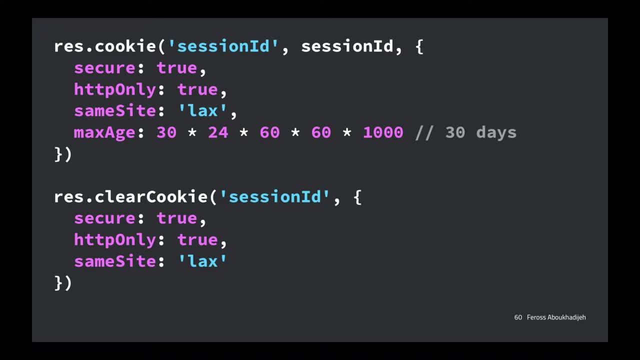 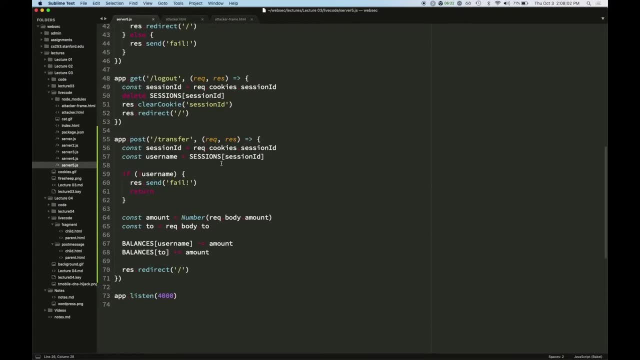 Everything else has to line up exactly. Okay. so I'm going to go ahead and try that. So let's go to our server and try to do this defense. So we're going to go in here and we're going to say, okay, set our cookie. 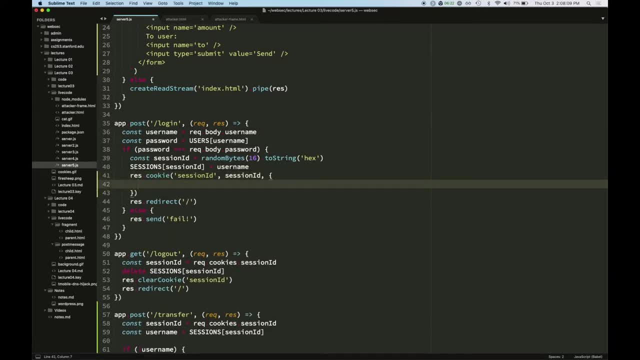 When we set it, we're going to make it be. what did we say it was going to be, It was going to be. so I want to do secure, true, but actually I can't do this because we're running on localhost, which is I just have an HTTP server. 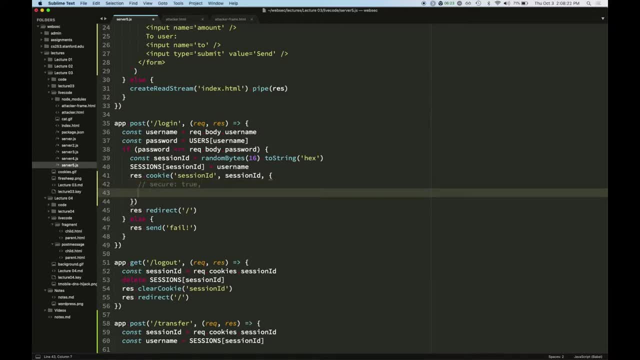 So I'm going to go ahead and omit this particular option. But we could do that on a real, On a real production server. But I'll do the rest. I'll do HTTP only to protect it from JavaScript, And then I'll do same site. 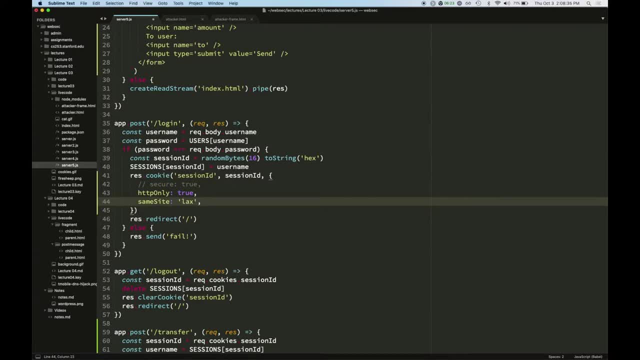 In particular, I'm hoping that this one is going to actually protect us against the CSRF attack. And then let's just set a max age, because- why not So? 30 days, 24 hours in the day, 60 minutes in an hour, 60 seconds in a minute, 1000 milliseconds. 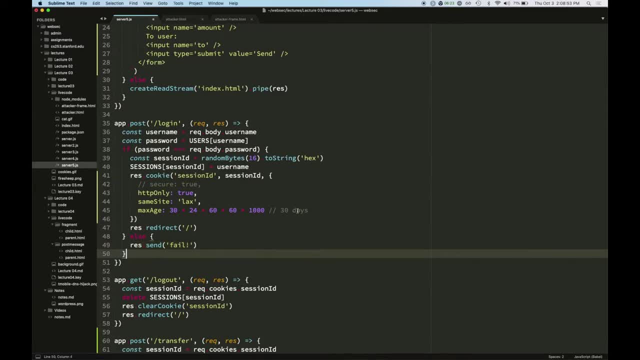 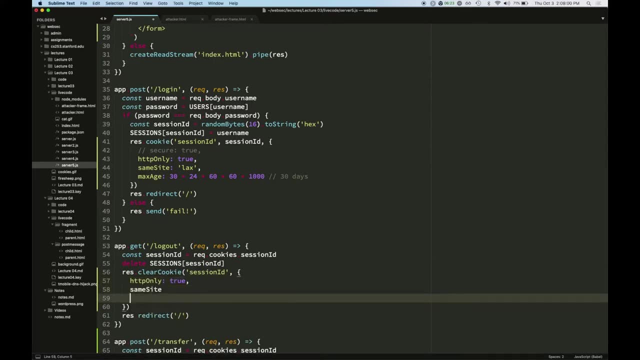 That's 30 days, Okay, And then when we clear the cookie, we have to pass, like I said, the serve same options. So let's do HTTP only, true, and same site lax, Okay, And I'll just omit secure again, because we're not doing that. 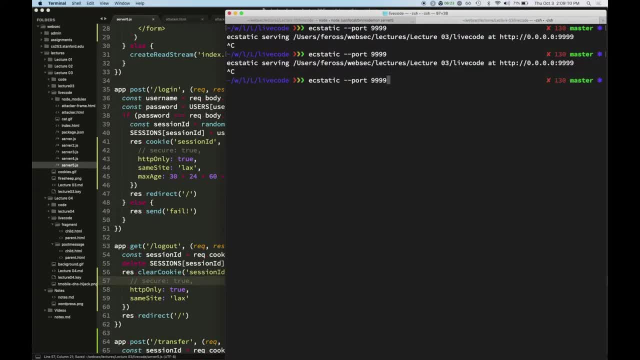 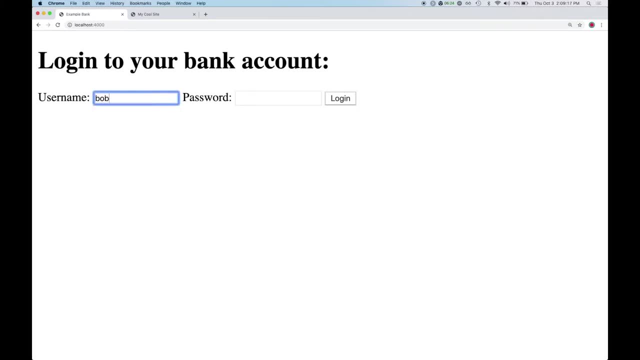 Cool, All right, That should be it. So let's see if it works. So I'll just restart these servers for good measure, just to be sure. I'll refresh my bank log in as Bob right, Because Alice is the attacker in this case. 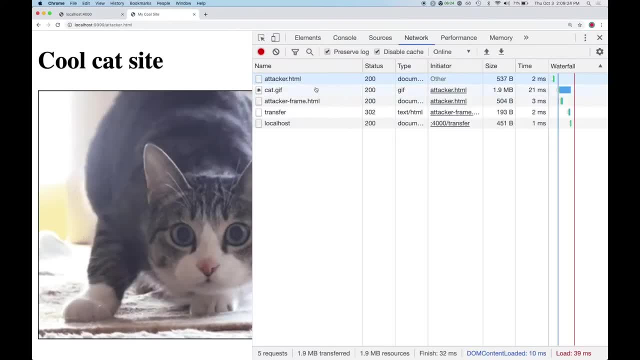 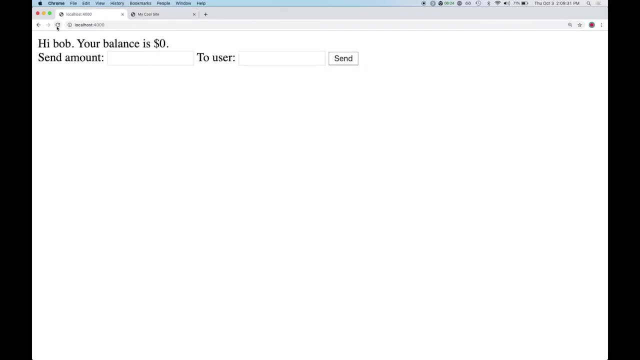 So okay, Bob's balance is back to 100.. Hooray, And we come here. We'll refresh the page, And now let's take a look at the. let's just check our balance first. Refresh- Whoa What. 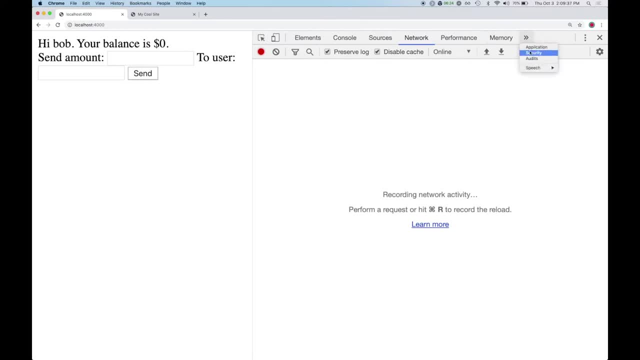 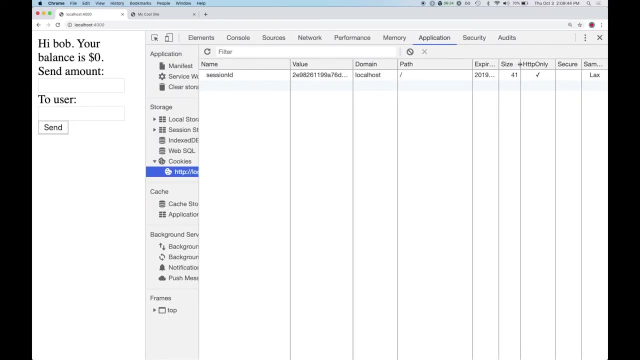 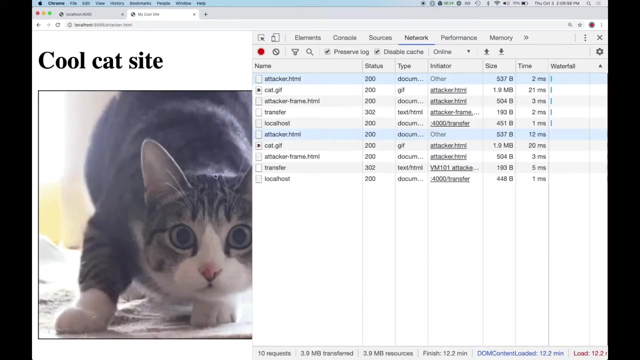 It didn't work. What the heck? Okay, Let's see if we can debug this live. What happened? So HTTP only is on and same site, lax, is on. What gives What? Okay, Let's see. As far as cookies are concerned, I mean, yeah, it's still local host, but I don't. 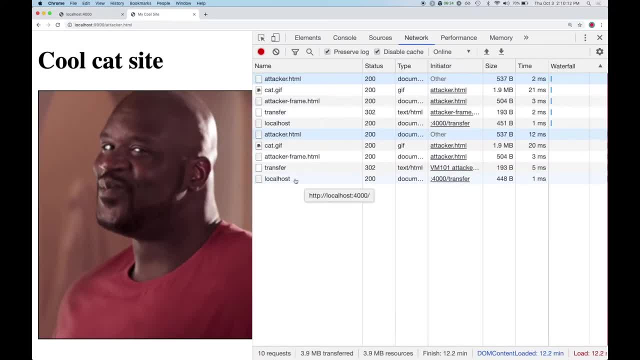 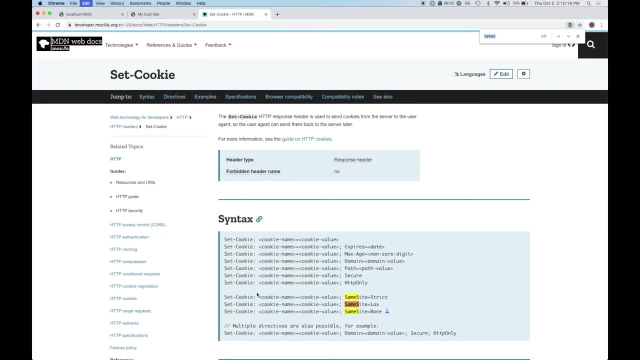 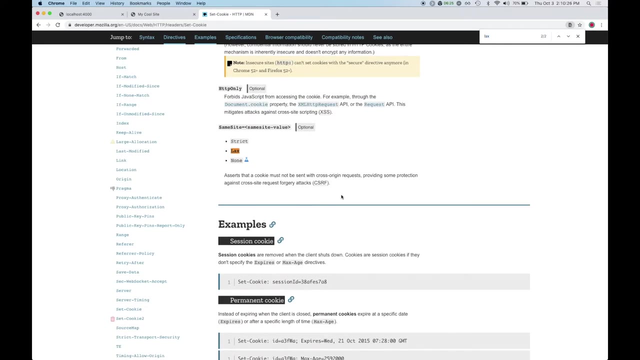 think that should matter, because same site is defined as: Okay, Let's see if we can. All right, I'm going to do some real time debugging here. Okay, I'm going to check this out really quick. Okay, This is not specific enough. 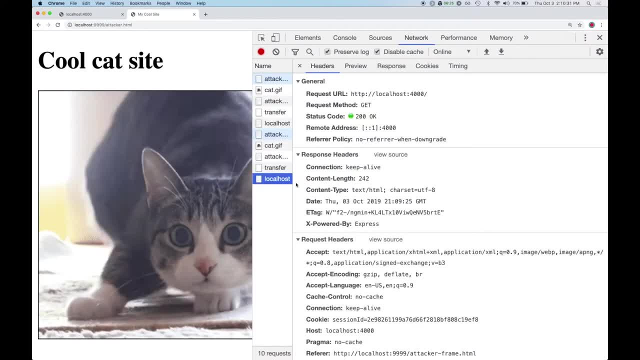 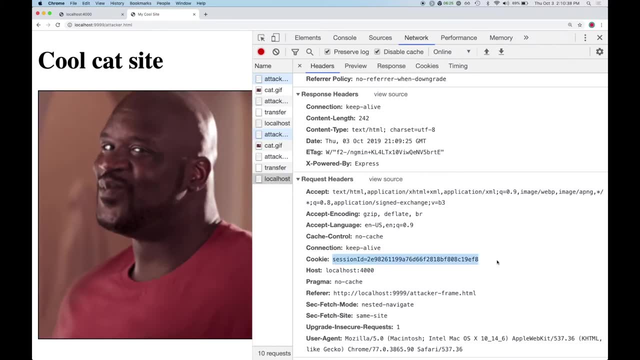 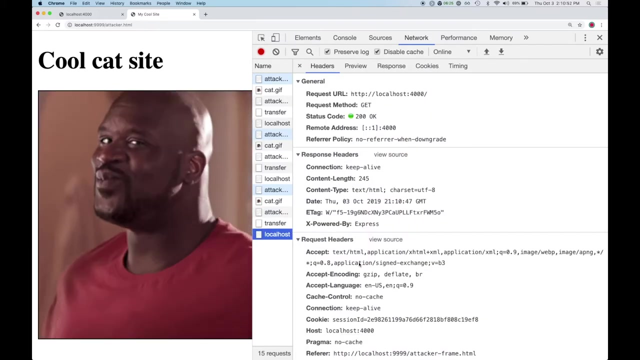 I need to dig into the spec to see what happened here. So our cookie was attached, despite the fact that it was same site. Maybe this is because, Actually, no, I can't figure out why this happened. I can't figure out why it would do that. 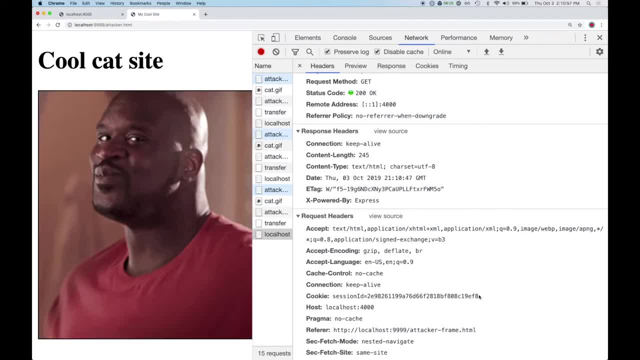 It could be that same site is because it's local host Here. Here's one thing we can do. I can, Actually, I don't want to do this. I don't want to do this live. Okay, Well, go ahead. 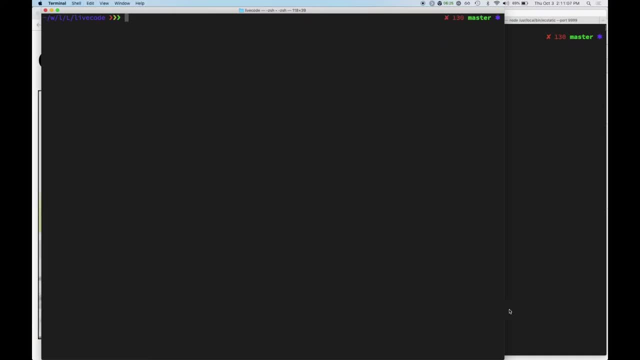 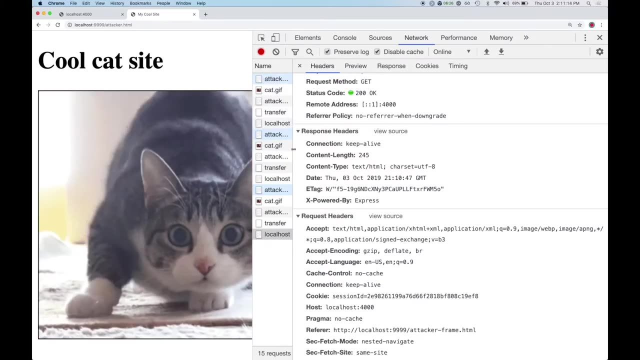 Suggestions. You said something about like lax, allowing the top level and the bottom level. Yeah, Yeah, I mean okay, Maybe that's what it is Like, let's just see. I don't think that's the case. 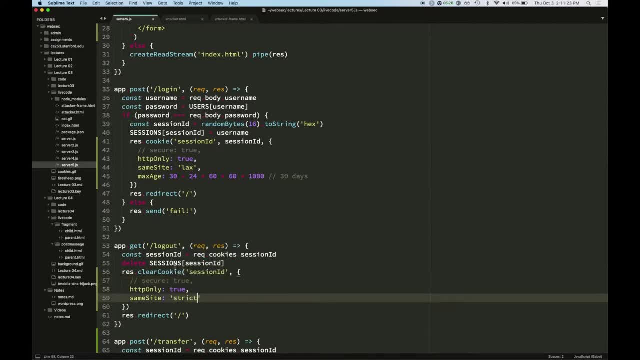 But let's rule it out. Okay, So I'll do this again. So cookies I should have. Let me just delete this. Refresh Bob Hunter 2.. Okay, So now I've been given a strict cookie. 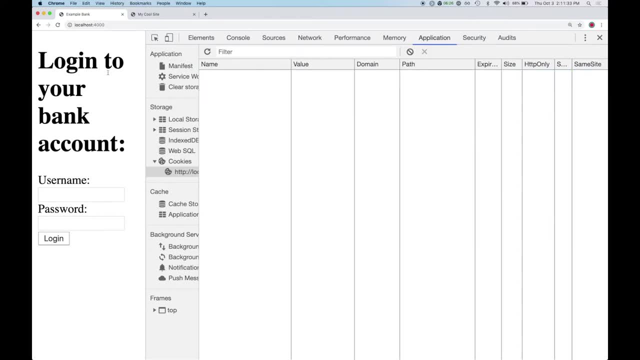 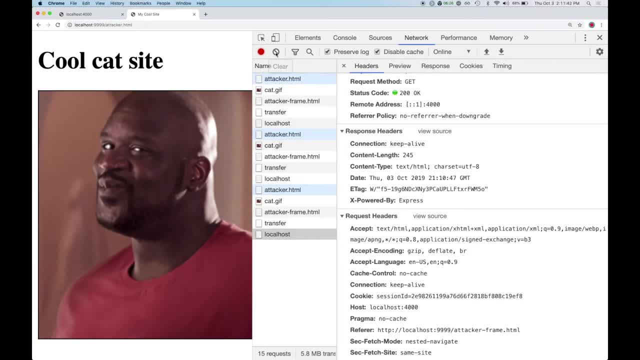 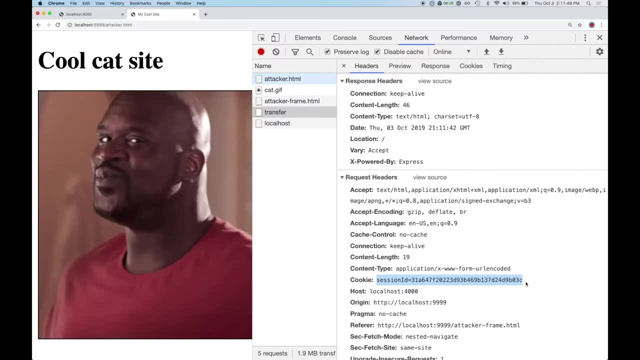 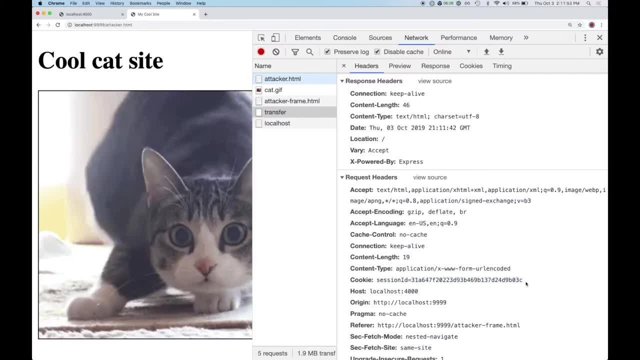 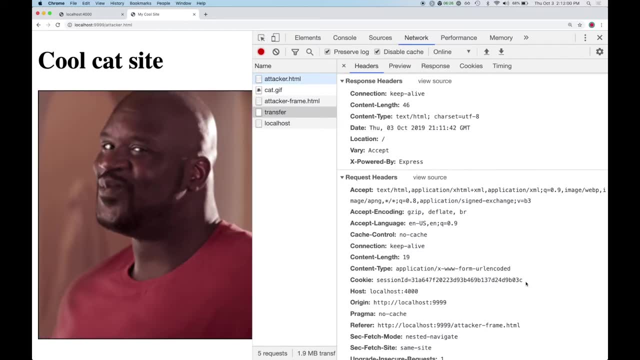 The request header still includes the cookie. Okay, Okay, I'll just I'll debug this offline and I'll get you guys an answer next time about why this is happening. So, cookies, The cookies, and also same-origin policy, which I'm going to talk about in just a sec, don't. 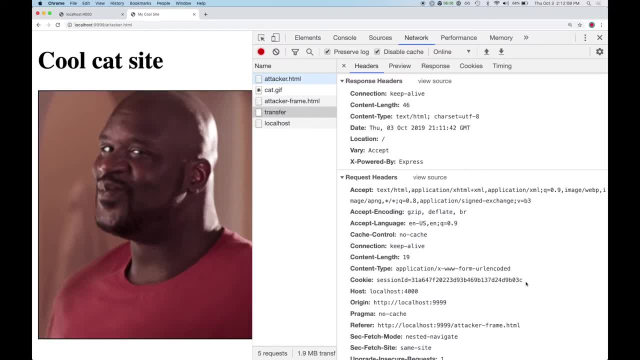 actually care about the IP. They only care about, like, the domain itself. Yeah, And in the case of same-origin policy, we care about a couple of the other things in the IP URL too. But yeah, maybe what's going on here is it's because the domain is the same and 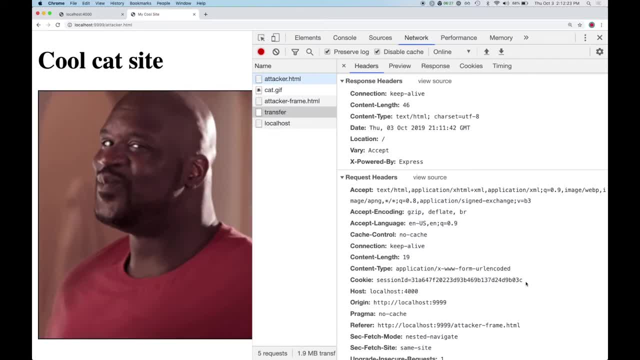 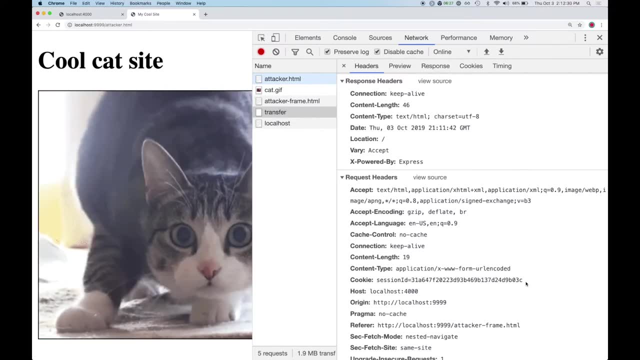 cookies. might be looking at that, but I'll get you guys an answer next time. I'm not sure why this happened. Doesn't the setBitch site, the same site, give any clues, or is that useless? Oh, that's actually very useful. So these are sort of new security headers that the 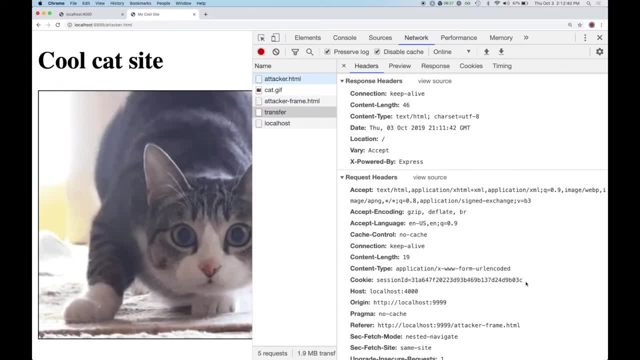 browser attaches to help you figure out where a request is coming from and how it was triggered, so a site can make more intelligent decisions. And you're right, it does think that it's the same site, So I'm guessing this is because of localhost. 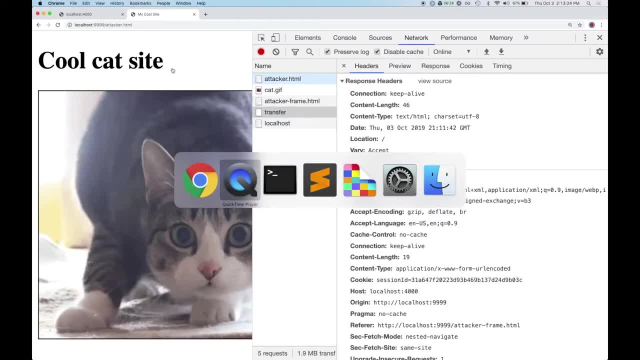 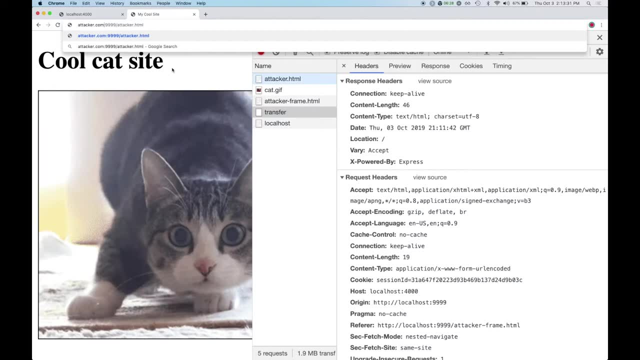 Okay, here I'll just try one thing really quick. So we're back in action. So what I did was I basically just added a mapping from attackercom to my local computer. So if I type in attackercom now, it's going to actually just fetch a page off of my own. 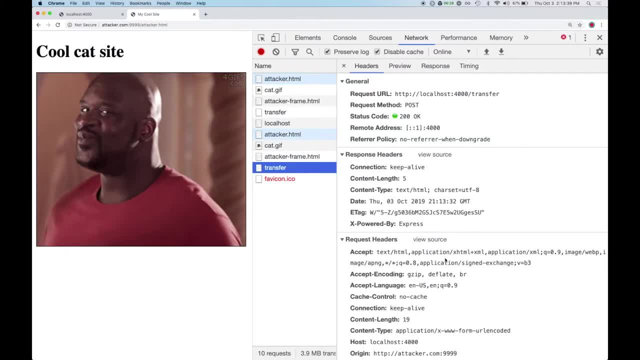 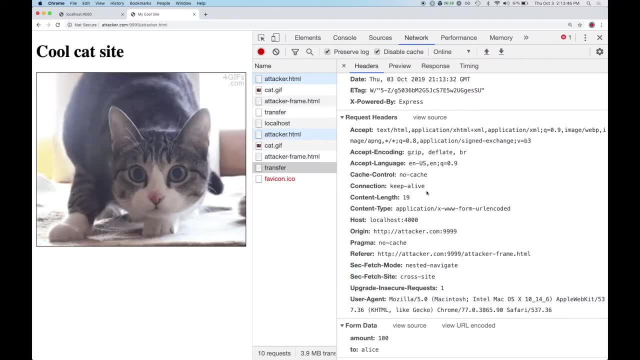 computer. Okay, So now let's see what happened here. Ah, secFetchSite is now cross-site And The cookie's not sent. So yes, Thank you, That's it, Yeah, Cool, So okay, so let's. 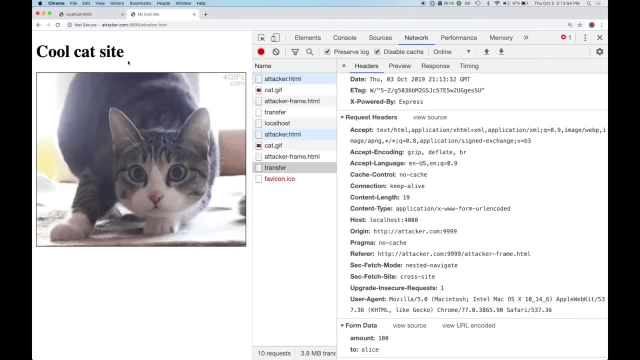 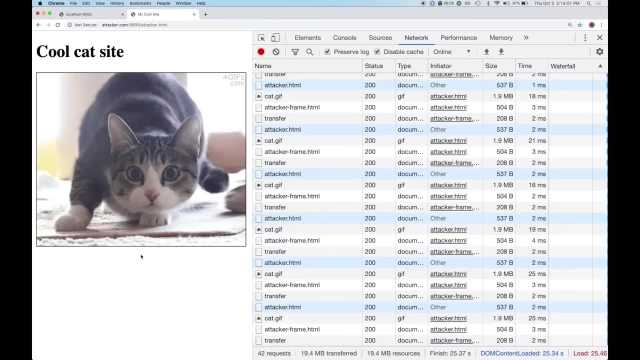 see how much of the balance is at now. Okay, so well, it's probably at zero because of the other one succeeding, But if I refresh this a few times now I come back here, it's okay, Those requests are not succeeding, Excellent. Okay, so this is because cookies are looking. 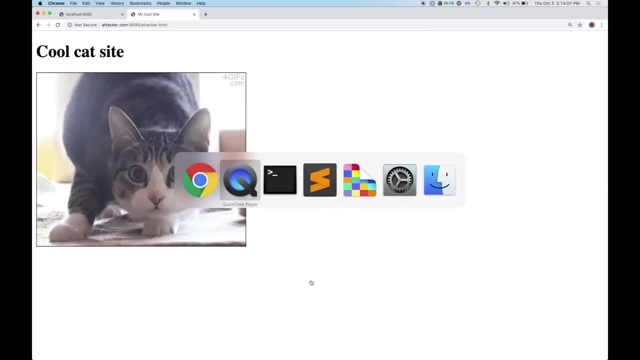 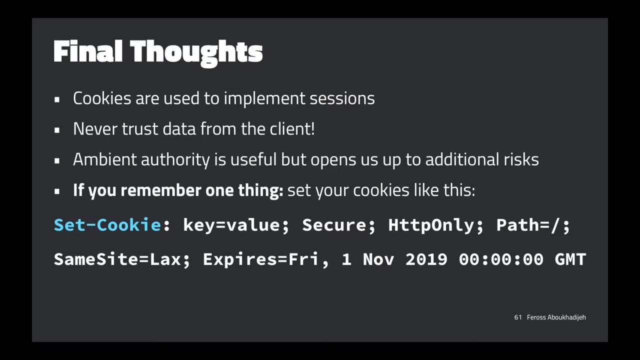 at just the domain, not the whole origin. Okay, Excellent, Cool. So just final thoughts on cookies. So cookies influence sessions never trust data from the client. So yeah, ambient authority is useful, but it opens you up to some risks And if you remember, 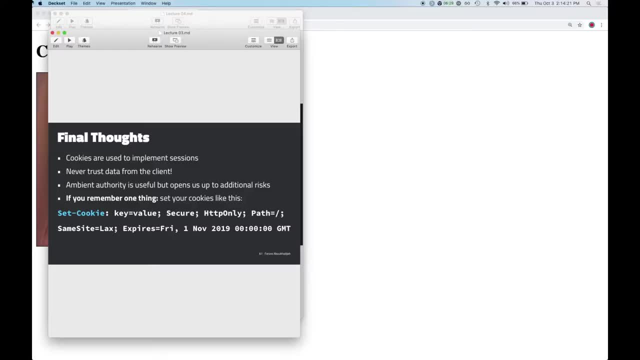 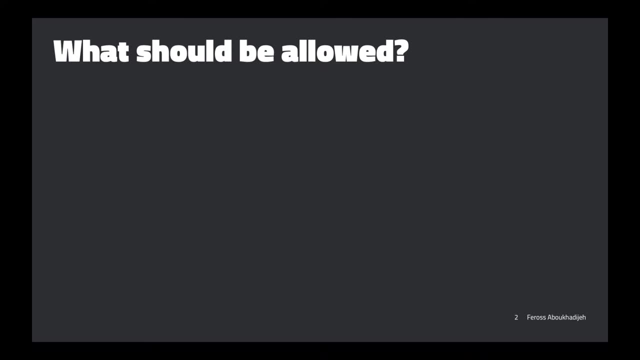 only one thing: set your cookies like this, Cool On to same origin now. So all right, For same origin policy. basically, the idea here is: we want to think about what do we want to allow and what do we want to deny. So let's go through some scenarios Should. 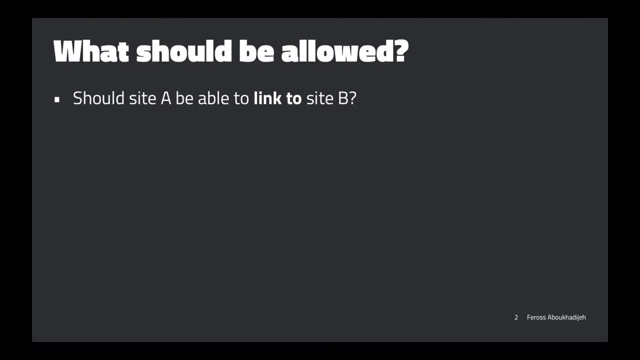 site A be able to link to site B. What do we think? Should we allow this? Yeah, I mean, this is the way the whole web works. So, yeah, this is too useful to not allow it. Okay, Should a site, should site A, be able to embed site B? What do we think? Yeah, Okay, Anyone. 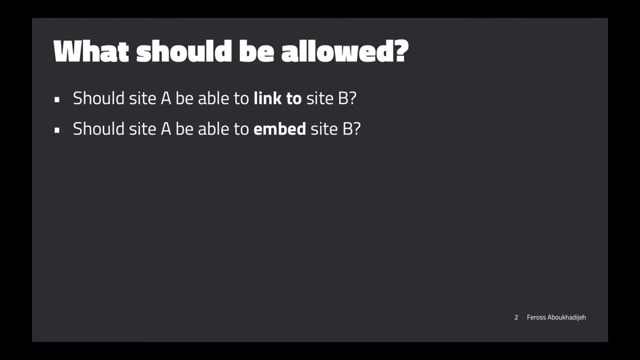 think, no, Yeah, It kind of depends Like I don't know, this seems like it's kind of useful sometimes, but it could be kind of dubious, Like maybe I don't know, maybe you can do something bad with this. 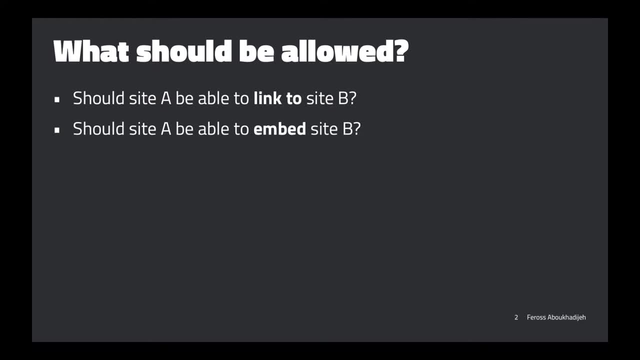 Yeah, So this could enable some sort of- maybe weird- interactions between the sites. So, yeah, this is maybe not- I don't know- maybe not a good idea. Should site A be able to embed site B and then go into that frame and modify its contents? 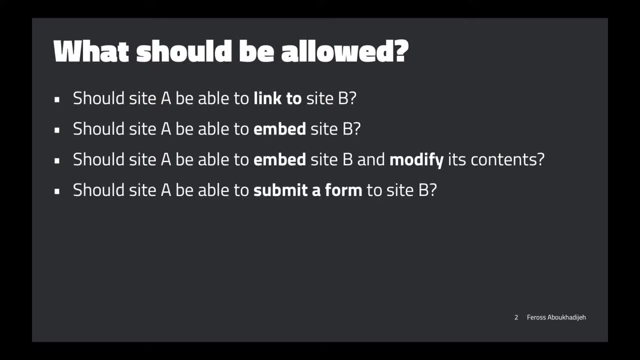 Probably never, right? Yeah, This seems kind of bad. What about submitting a form? I think we just saw that's kind of a bad idea, but yeah, that actually seems like it's allowed. Should site A be able to embed images from site B? 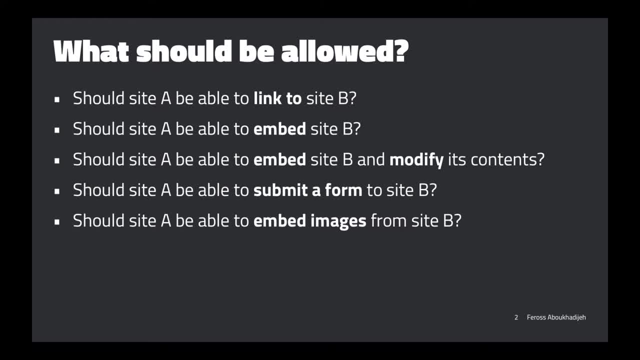 Yeah, Sounds like a good idea. Yeah, It seems like it's probably more useful than not useful, but I don't know Who thinks no. Yeah, Why Is embedding really that useful? Is embedding resources from other sites useful? 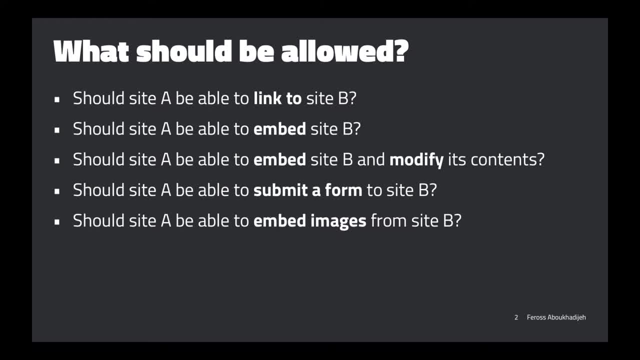 Right, Like it doesn't seem so fundamentally that it does Mm-hmm, And I just can't think of in my head a time where there's absolutely no way around it. like from a product standpoint, The design has to be embedded. 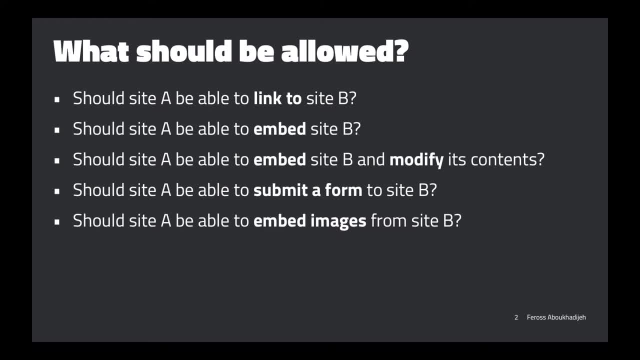 Mm-hmm. Yeah, I think that's the right way. Okay, Yeah, So I think that's a good idea. Yeah, Yeah, I think that's valid. Yeah, I mean it's. it's kind of useful to be able to like link to someone else's image on your on your site. 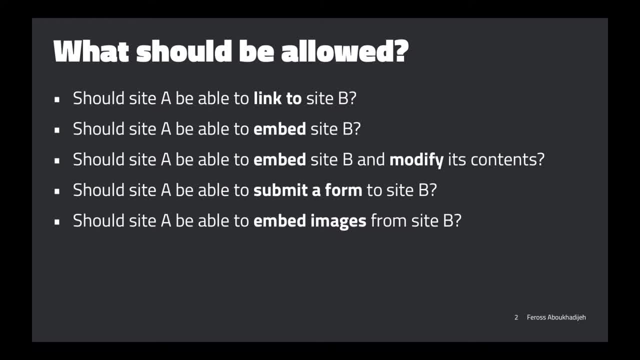 So you don't have to like re-upload it to your own page. But but yeah, I mean if we were doing this again and maybe we would just design things so that everything is isolated from everything else and the only thing you can do is link and 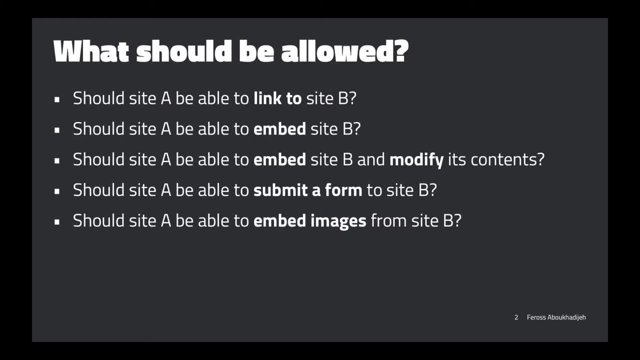 And then you could sort of peel off the security if you, if you want to, But yeah, Yeah, we can't, we can't, but can't go back and do that now. Is there somebody else raising their hand? Mm-hmm, Yeah, that's, that's a good use case. so this is the CDN use case. 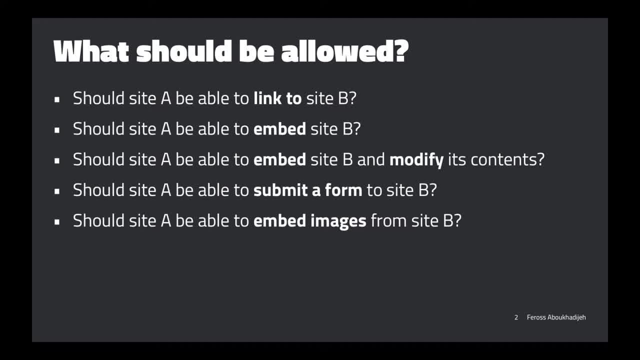 So the idea here is say that every site is just including the same JavaScript library that helps them build their site. You can just have all the sites just reference the same URL To this, to this file, and then, once you've been to one site that uses it, it'll be in your cache. 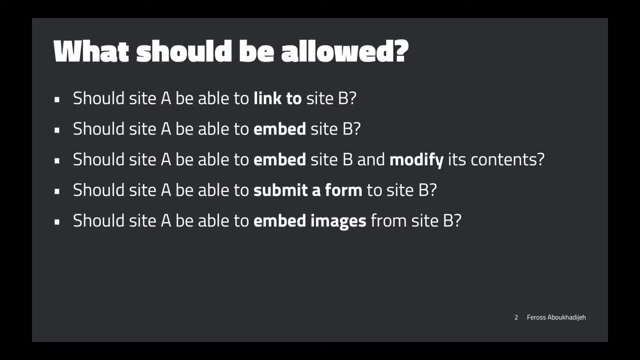 So the next site you go to it'll be like: oh, We've already, We already have that file and it'll just the sites will load faster. This is like less useful these days because people often the builds are so complicated and there's so much custom code that you can't really get. 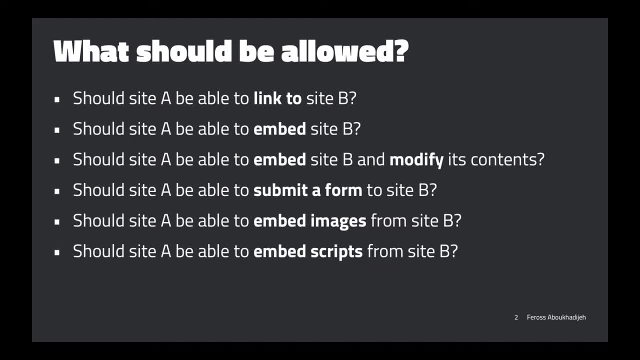 Much reusability across sites. but yeah, that was, that was useful at one point in time. What about embedding scripts? should I be able to embed a script that another site published into my page? I Mean, yeah, I don't know, that seems like okay, There's some, some, some, some shaking, shaking heads. What about reading data? 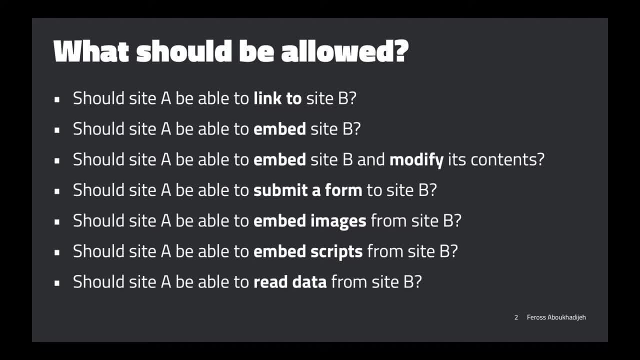 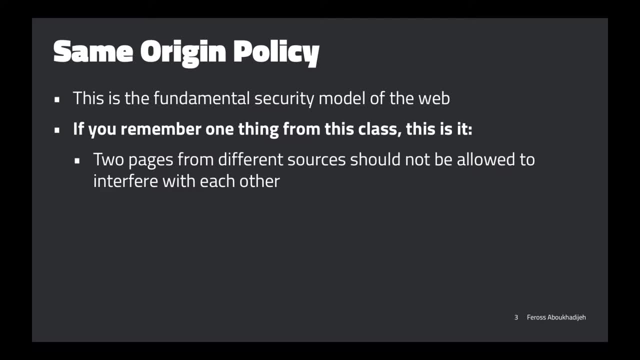 Should I be able to read a sites on our sites data? Okay, Well, okay, Let's, let's go ahead and go through and see what is the same for urgent policy actually actually say, and what does it allow? Okay, so so this is the fundamental security model of the web. 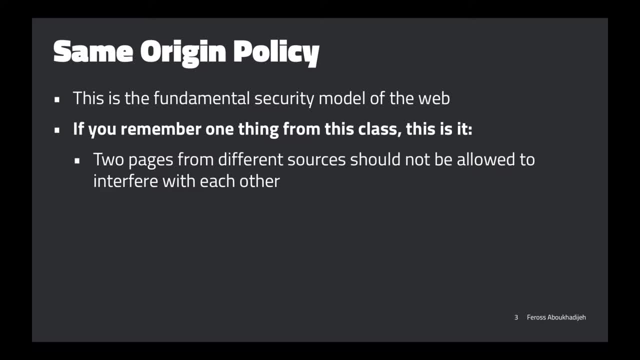 If you remember one thing from this class: that this is the, this is the thing to remember, The idea, the key idea is: two pages from different sources should not be allowed to interfere with each other. So if we, if we can accomplish this, then this seems like a good. this seems like a sort of a good. 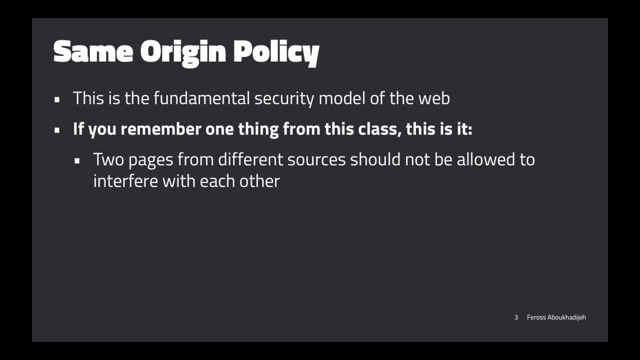 Philosophy to have when we're coming up with with all the different security rules we want to have. So yeah, I'll just say it again to two pages from different sources should not be allowed to interfere with each other. Now, now this gets complicated when we actually think about. what do we want to allow? what we know? 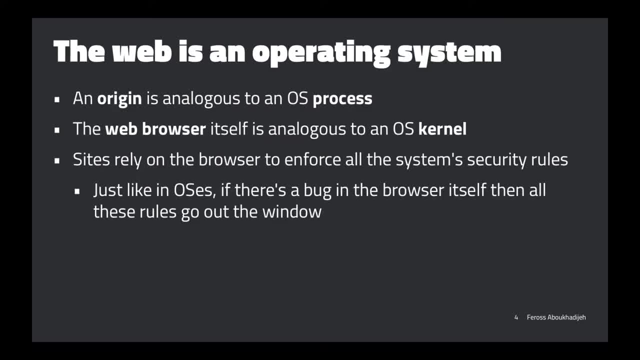 We don't want to allow, like we saw from the list of questions before. it's it's not. it's not so clear, But but but at a high level. at a high level. if you think of the web as an operating system, Then we can think of an origin as like a process in an operating system. 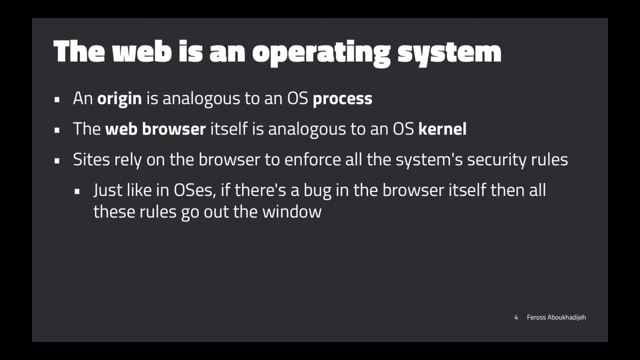 so the job of the operating system kernel is to Keep processes isolated from each other so they can't interfere with each other's memory contents or interfere with each other in other ways, And the browser is going to perform this role for us. So the browser is the, is the off is the operating system, and then every different origin is going to be a different process. basically, 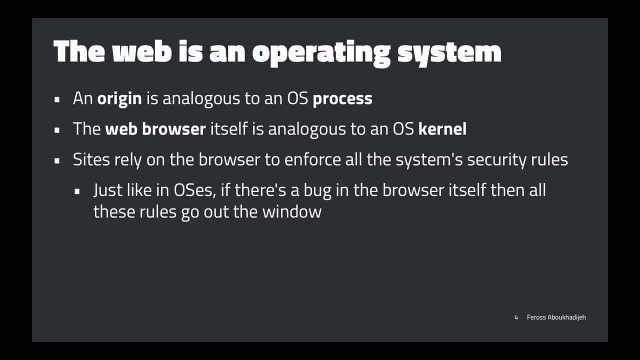 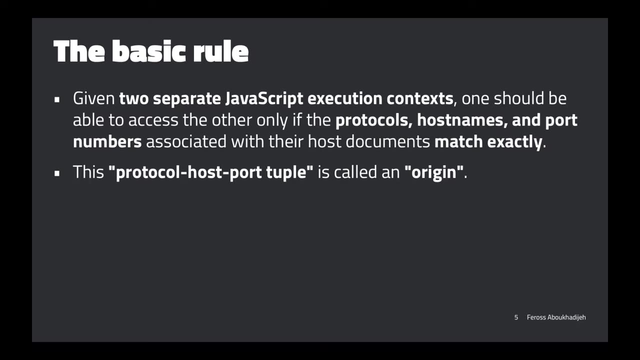 So so we're relying on the browser to actually enforce these rules, And if the browser has a bug in these and its implementation of the same origin policy, then then anything could happen. So we really need the browser to do this right. So So the basic idea is given two separate JavaScript contexts. 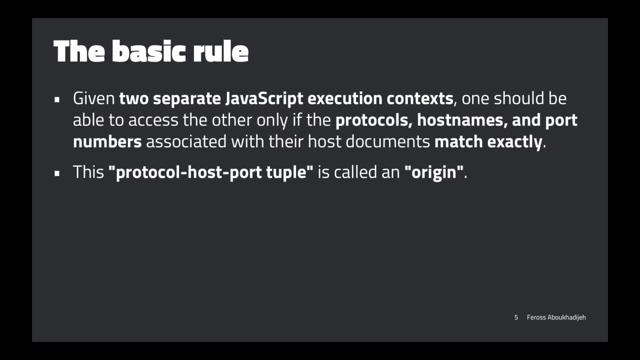 one from this origin and one from that origin, you should not be able to access the other. If the protocols, hostname and port associated with each of those. sorry, the other way around: If the protocols, hostnames and ports of those two contexts. 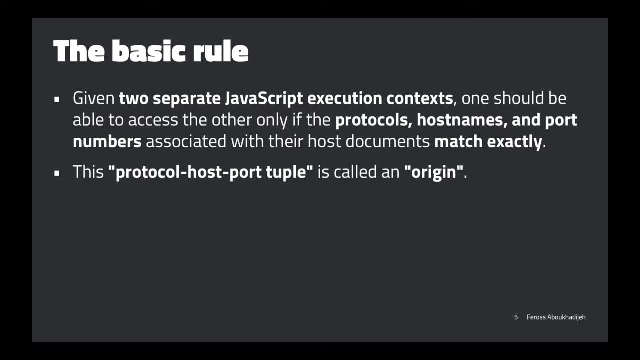 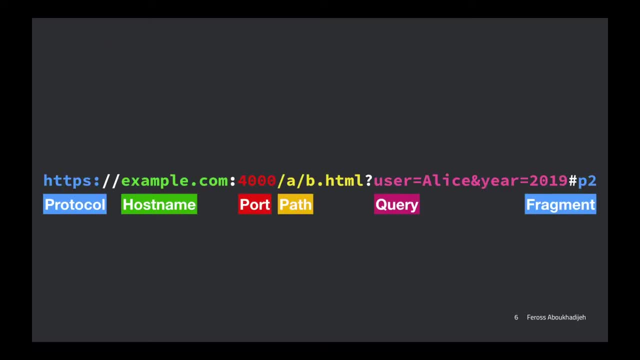 are the same, then they should be able to access each other. So we call this tuple of protocol, host and port an origin. So just a reminder, this is what the URL looks like. I showed this slide on day one. And specifically, if the protocol, the hostname, 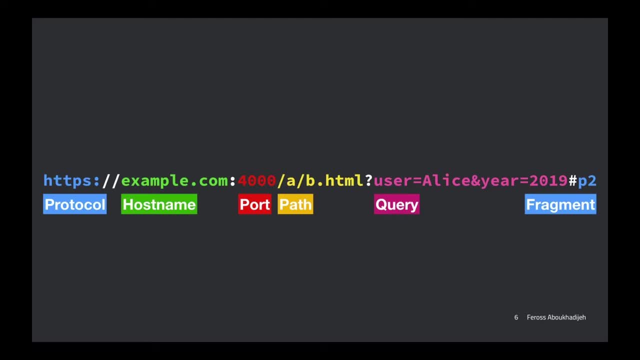 and the port are the same between two different contexts, then they are allowed to interfere with each other as much as they want, basically. So this is the part that we care about when we're judging whether something is the same origin or not, And this is like just to drive the point home. 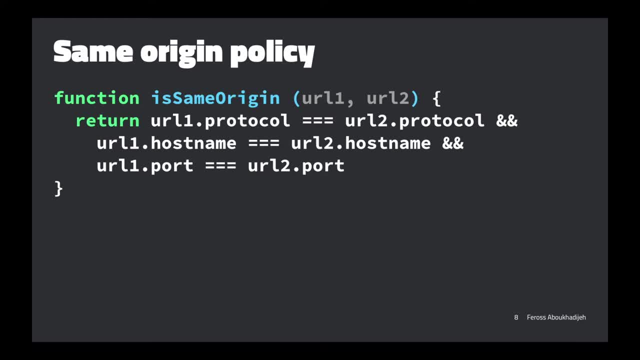 it's not that. the implementation of it is not that complicated. You could write this function yourself to decide whether two URLs are right or are same origin to each other or not. So that's one nice thing about the same origin policies: It's pretty easy to understand and to explain. 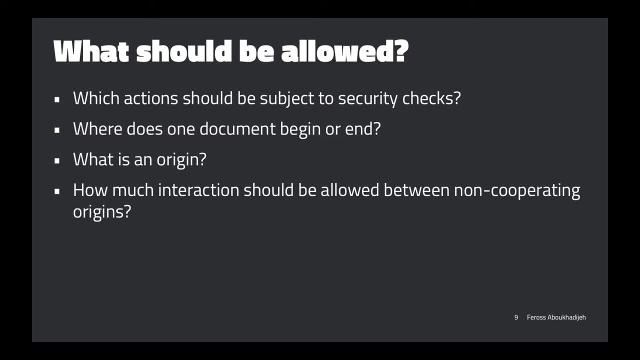 But it gets confusing when we actually think about: OK, so say that two sites are actually different origins. When do we exactly want to enforce different security checks, And how do we define where a document begins and ends? And I don't know why I have what is an origin on there. 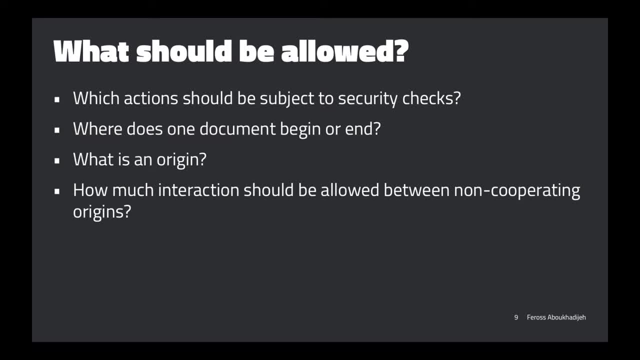 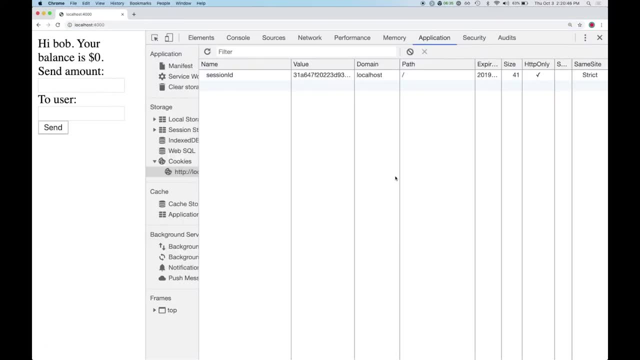 because we just defined that. But how much interaction do we want to allow between origins that don't cooperate with each other? So I thought I would just show something, show another little demo here. So I'm going to go to the 106 page again. 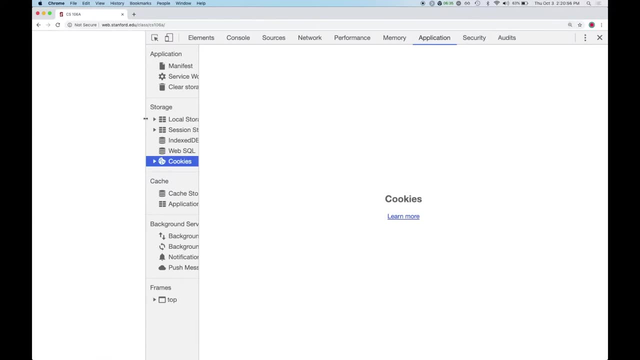 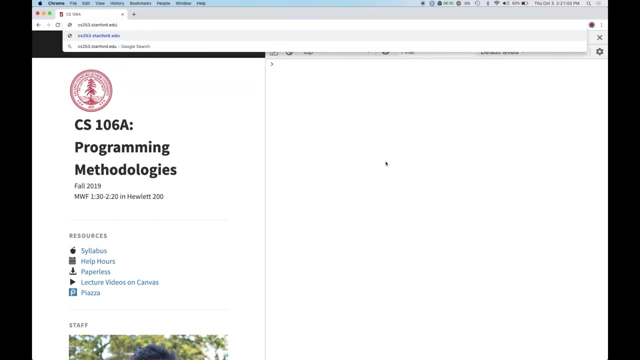 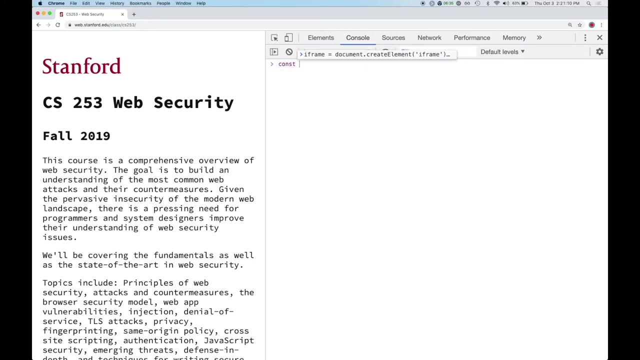 click on them again, And what I want to do here is just so. no, sorry, I want to go to the 253 page And I want to. I want to just just remind ourselves that we did last time we did this thing. 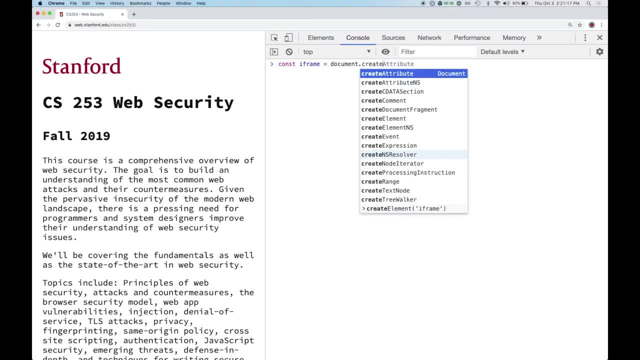 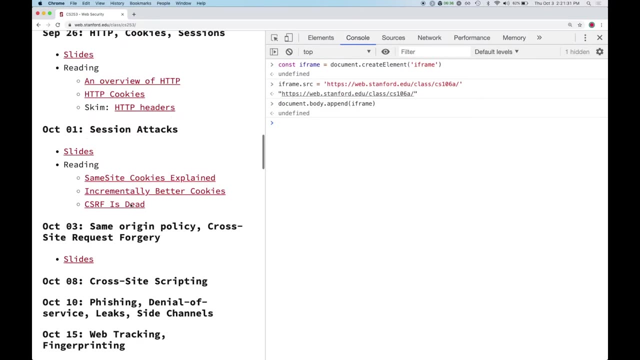 where we created an iframe and we put it into the page. How come I can't tab that? OK, yeah, so we created an iframe, We set it to the 106a URL And then we did this to add it to the page. 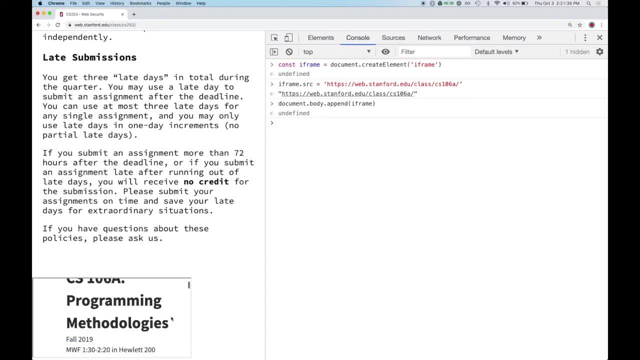 And then it got added and we were able to load it. So, even though these are- oh yeah, these are actually same origin. That's what we said last time. So the protocol and the host name and the port are the same between my site up here and 106a. 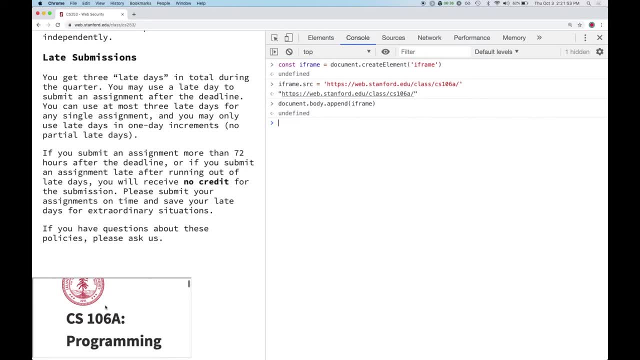 So basically, anything goes, I can do anything I want to this page. I can go into it and delete elements, modify things, et cetera, et cetera. But what do we think will happen if I do the same thing here? 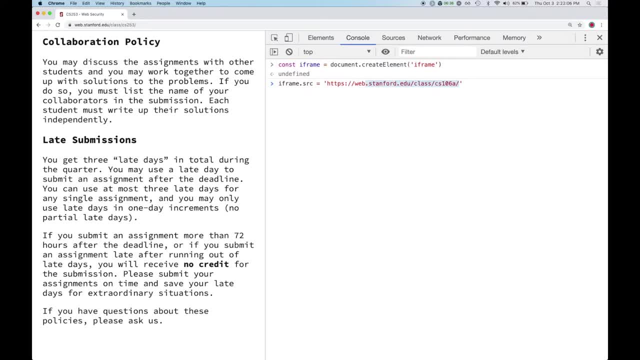 but I do it for a different page. Let's do cryptostanfordedu. Let's see how good is their security, So append this to the page. So, hey, do we think this is going to work or not? No, It's another origin, right? 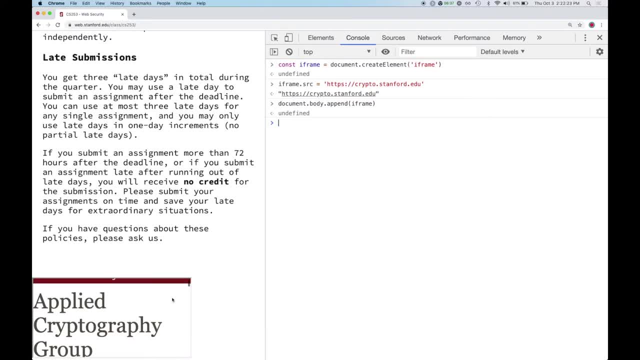 So we maybe think it hopefully wouldn't work. Worked OK, so what does this tell us? So actually, sites that are different origins are allowed to embed one another. That's interesting. Now can I do the same thing I did before to the 106a page. 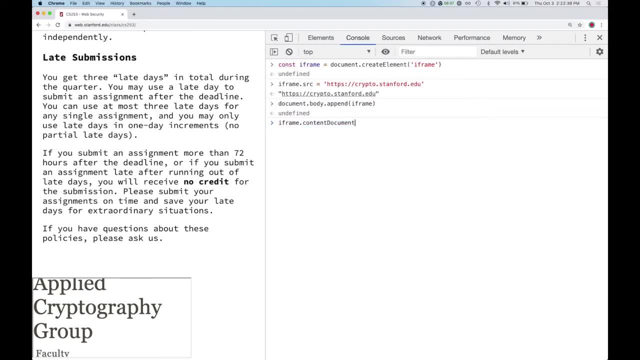 Can I do? iframe dot. what was it? content document, dot cookie. Does that work? Oh interesting, No, So if I try to actually see what happened here, the document is actually set to null, So I can't touch the document of that page. 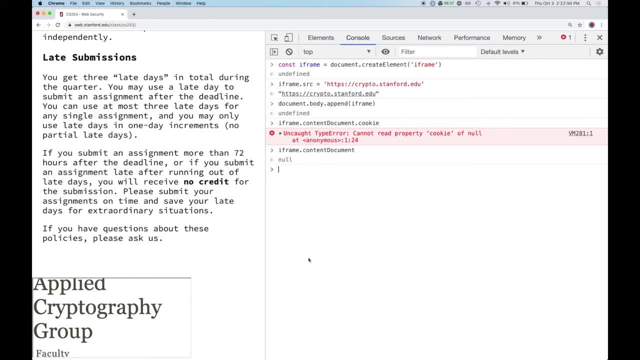 I'm allowed to embed it, but I can't reach into it and modify it. OK, good to know. OK, what else can we do here? Do we think I'll be allowed to do this? Can I reset the source of it to a new destination? 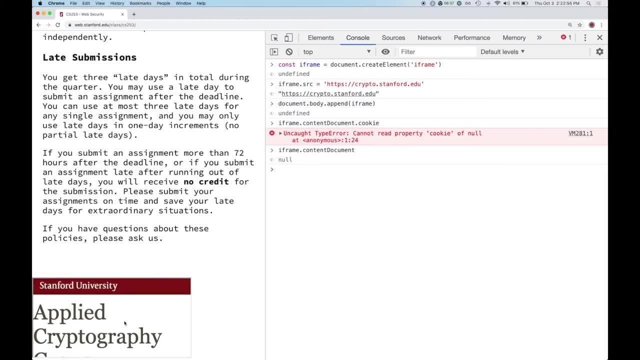 So let's see, Before I do this, let me just do something really quick. Let me make sure that I'm doing this right. So I'm going to do this, I'm going to do this, I'm going to do this. 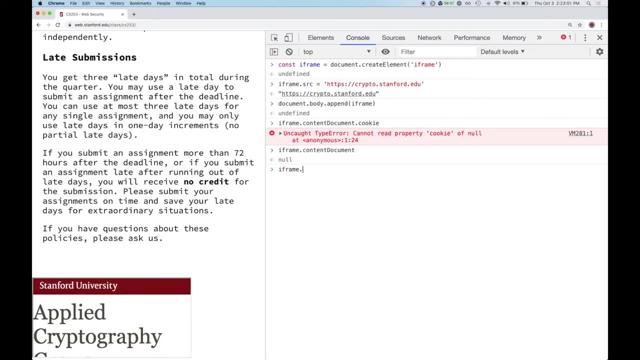 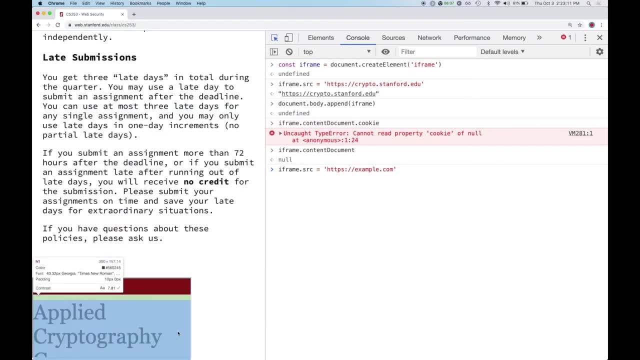 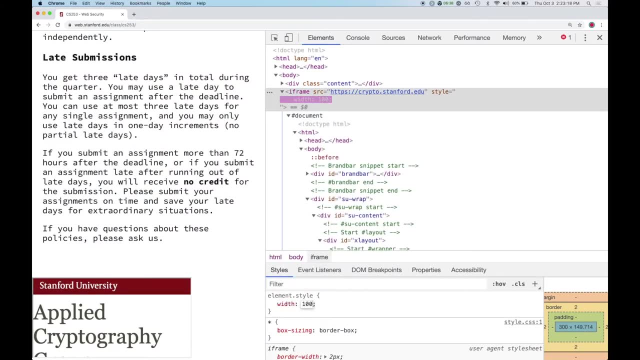 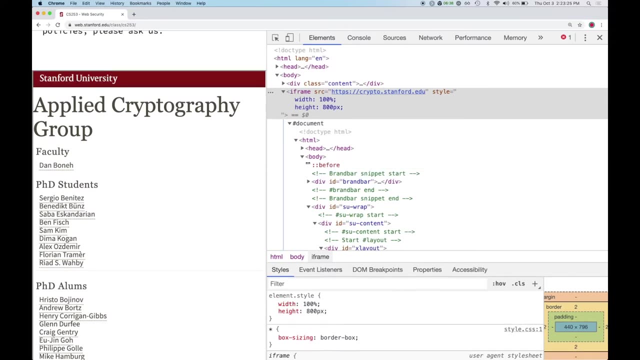 Before I do this, let me just do something really quick. Let me make this iframe less annoying to work with. I'm going to just quickly sort of make its width a little bit more reasonable, OK, So now. OK, cool, So I actually have kind of a bigger window to work with here. 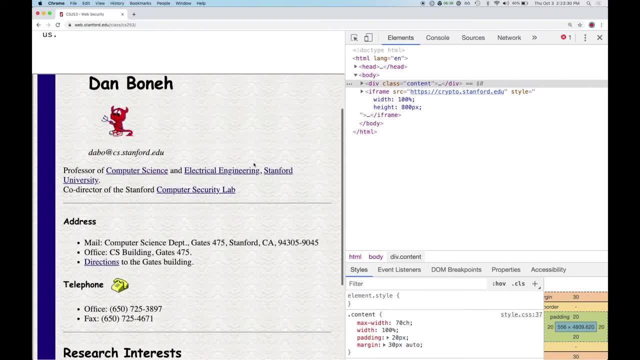 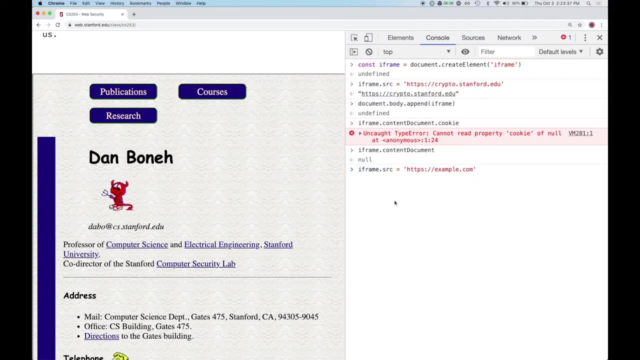 So say, the user sort of is like: oh, I'm going to learn about Dan, read about Dan, blah, blah blah. While that's happening, do you think that the site should be able to run this code sort of change the destination of the iframe? 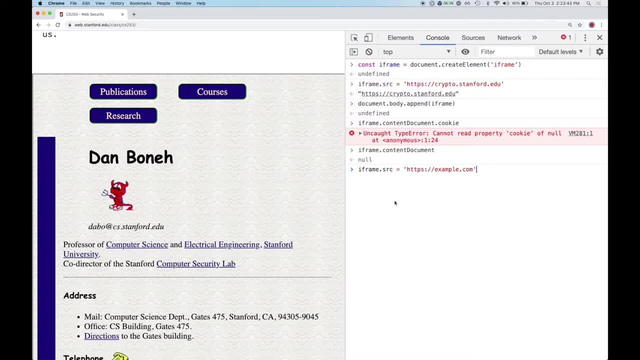 OK, who thinks, yes, it should be allowed? Mm-hmm, It should be allowed. Or why should it be allowed? Yeah, yeah, why? why? Because you created the iframe inside Uh-huh, So you were in control of it, right. 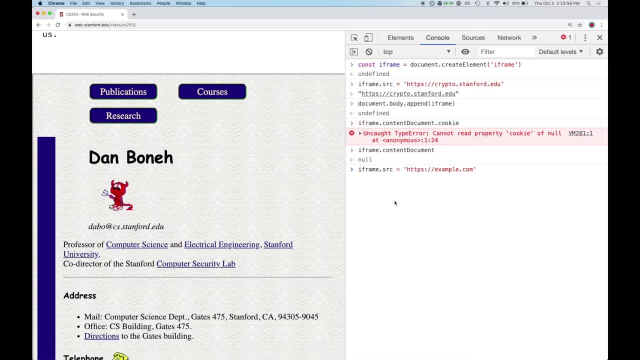 Mm-hmm. Well, I wasn't allowed to go into it and change it, But you still think I should be able to change its location? Yeah, OK, who thinks, no, I shouldn't be, I shouldn't be allowed to do this. 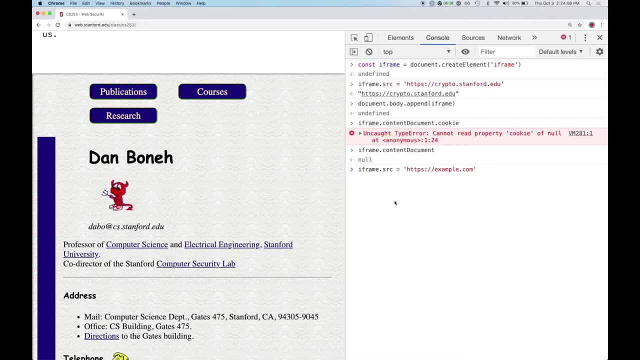 Mm-hmm, You could eventually like change it to like a fake version of that site and like embed that instead of like Wall-E, Wall-E can push it on the same site. Yeah, I mean, hopefully they would look at the URL. 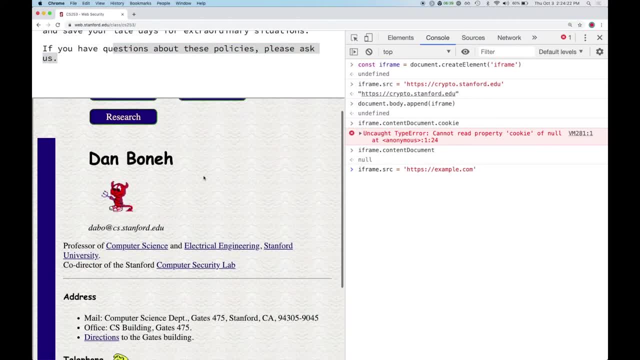 and see that they're on the 253 site right now and not on Dan Bonet's site. But yeah, yeah, that seems like a concern, So let's see if it works. So if I hit Enter, what do you know? 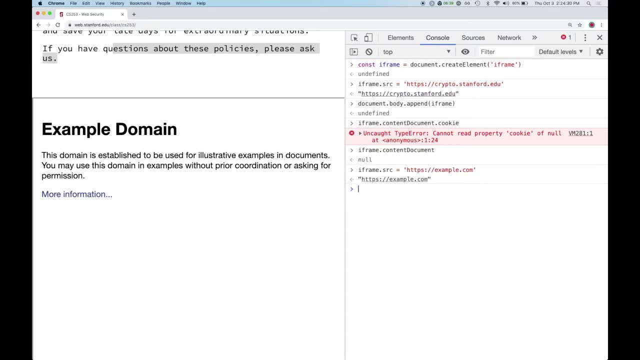 It works. So, even though this is a context that's another origin and I'm not allowed to modify it, I still can navigate the frame as a whole. That's kind of interesting, OK, what about? well, let's do one more thing. 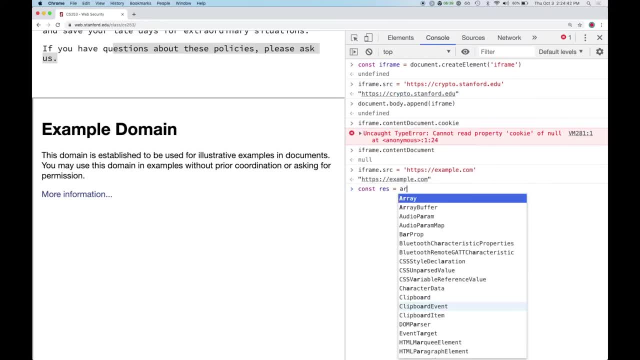 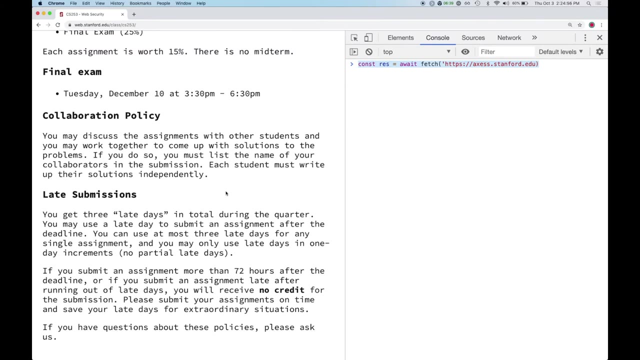 What if I use the fetch API, which is a way to sort of fire off an HTTP request? And what if I fetch? let's fetch. how about access? See if I can actually. let me just refresh the page here to emphasize that we're not doing anything with the frame anymore. 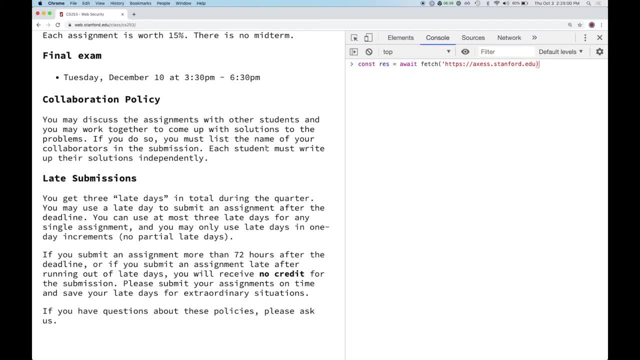 The frame is gone. What we're doing here is we're just we're on the 253 site and the 253 site just happens to be interested in data from access in order to serve its functions. So if I run this, do you think I should be able to read the response? 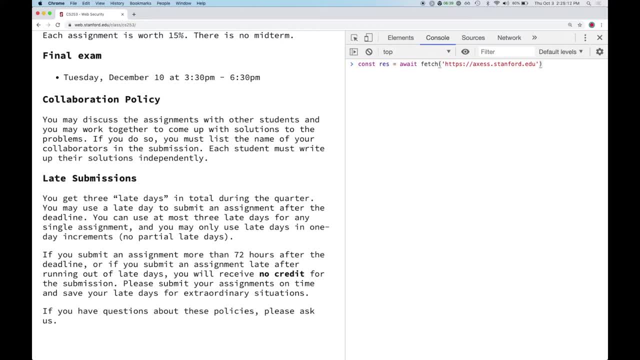 that this site sends back and maybe do something with it. Should I get back a string and be able to see what's in it? Yeah, Why do you guys think that I should be able to Thoughts? No, what I'm doing, I'm actually not navigating the window. 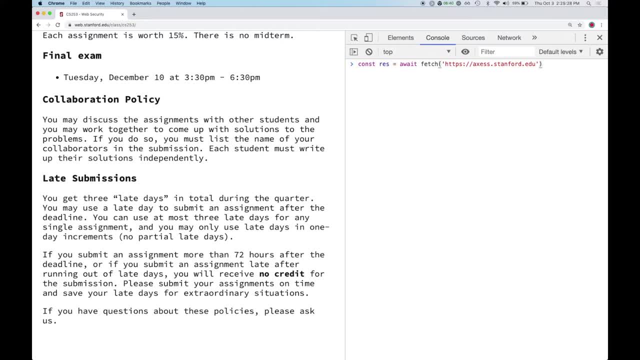 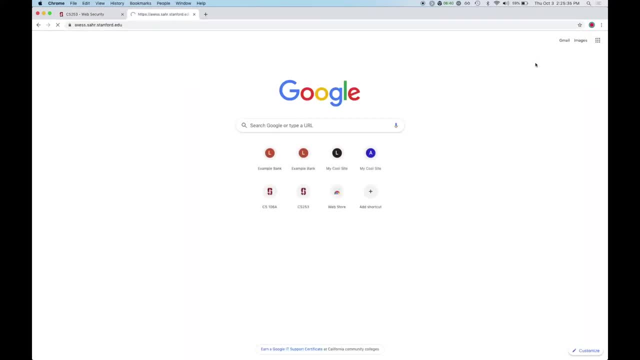 I'm literally I'm trying to get back like a string that I can sort of look at the HTML that I could see if I were to say: you know, if I were to visit it directly and then view the source. I'm trying to sort of do that. 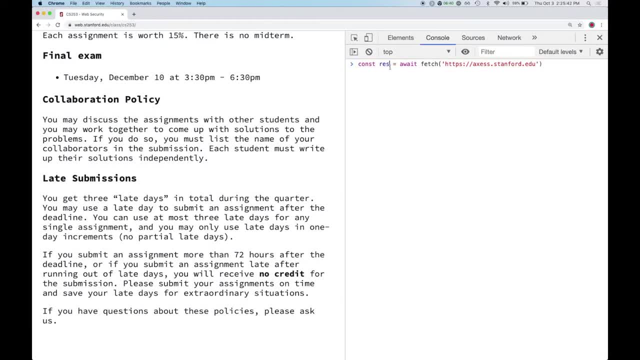 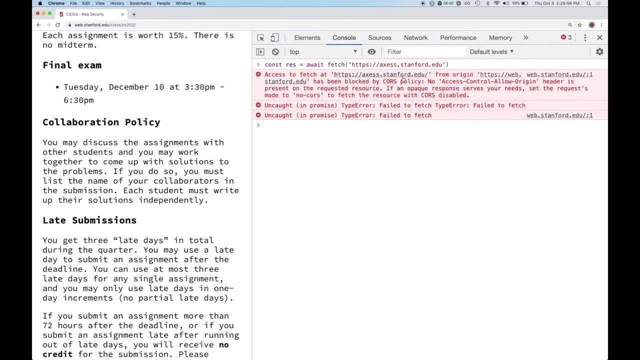 like I'm trying to get this back as a string and then, you know, do something with that string. Seems reasonable, Okay, Well, let's just see what happens. Okay, so I got a really scary message. Access to fetch at accessstanfordedu. 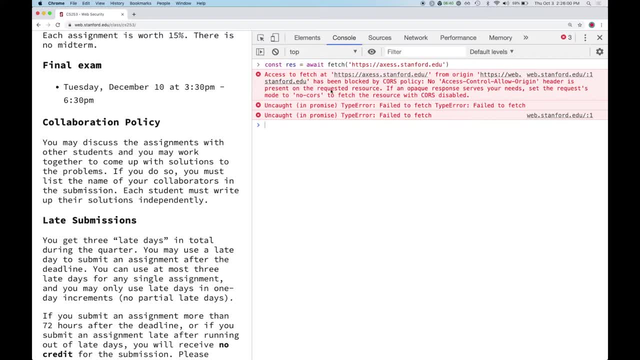 from origin, webstanfordedu, has been blocked by core's policy. So what this is saying is that the browser was going to attach my access cookies to this request and it was going to fire it off, and then, because of that, it doesn't want to actually give me back the result. 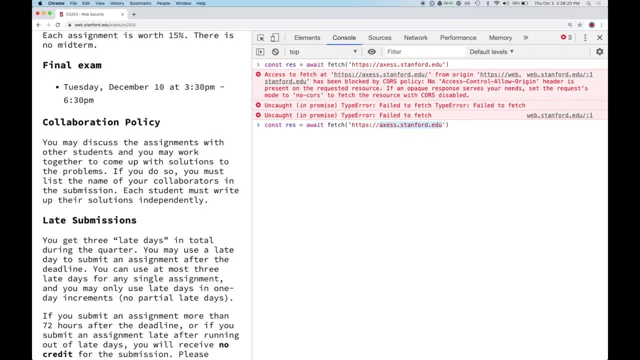 You can imagine if I did this for something like Gmail, right? Just think about what's going to load when I go to Gmail in my browser. All my emails, right. So it doesn't. it, doesn't? you know? you really don't want to let an arbitrary site. 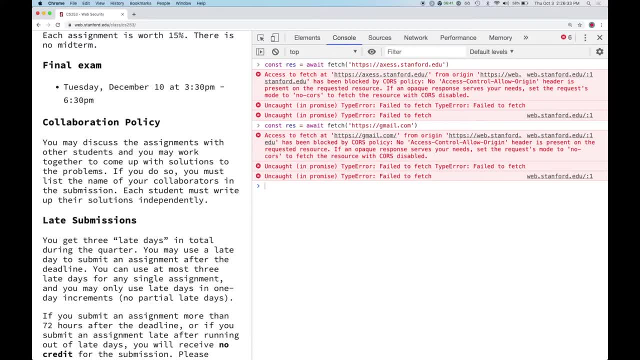 make a request to Gmail with your cookies attached and get back this sort of page that's full of personal information and let a different site read it. This is very different than my own server could make a request to Gmail. I mean, anyone can make a. 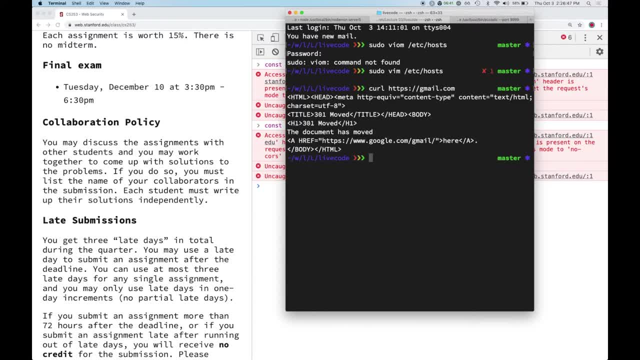 I could curl Gmail here if I want to and just sort of see what is Gmail going to send back. Oh, I guess it moved, But I mean, obviously anyone can make a request- and moved again. Okay, Keeps moving. Oh my gosh. 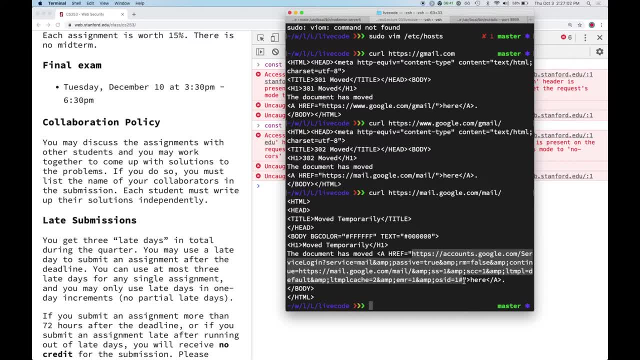 Are they serious? Are they serious? Oh, it's trying to log me in. Wow, That's why it's so slow. It sort of redirects to redirects, to redirects. Anyway, the point is, eventually, this would give me my emails back. 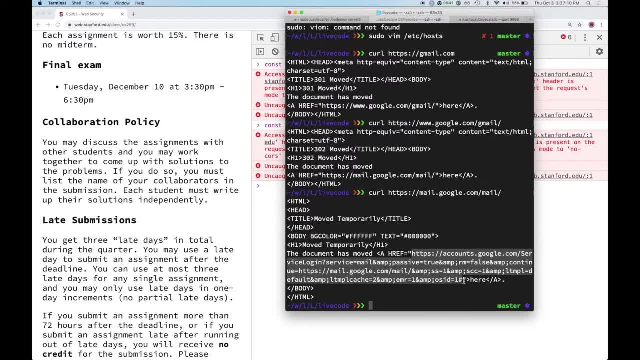 if I was logged or no. sorry, it wouldn't give me my emails back because my browser cookies are not being sent with this curl request, which is why it's no big deal, But in the browser context my cookies are going to be sent. 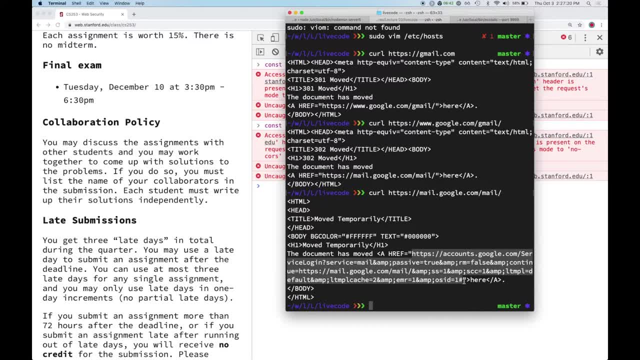 and I'm going to get back all my emails, So we don't want to let other sites see that. So this is enforced in the browser. so, like Chrome and Firefox could have different policies, Or even different versions of Chrome could allow some of this. 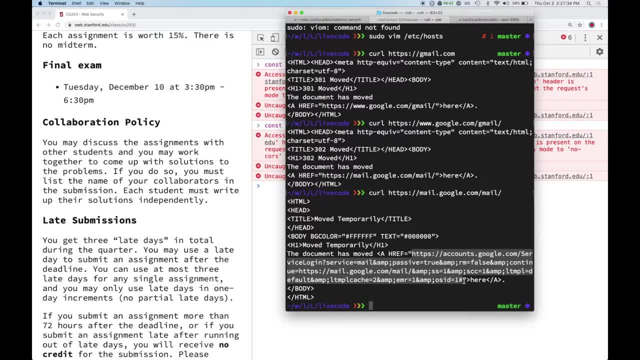 Yeah, we're relying on the browser here, But fortunately, when it comes to the same origin policy- this is like since it's the most fundamental security model of the web- it's implemented pretty consistently across browsers. There have been a couple of sort of implementation bugs. 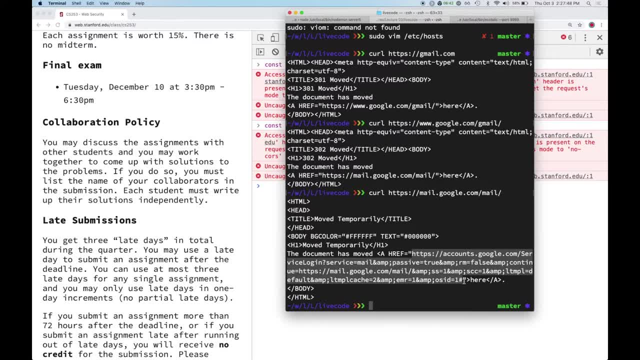 that have happened in the past And I hope I have time to, not today but in the future. I hope I have time to mention one of them. that was really interesting. But yeah, by and large this just works pretty well. 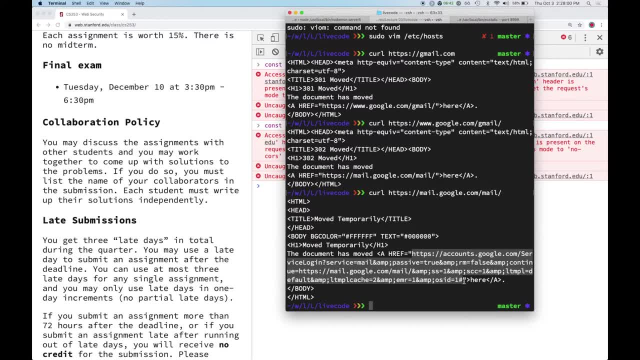 Yeah, it's sort of a the same origin policy, I believe was created a year after cookies were created, so like 1995.. By the way, that explains why they diverge in their definitions. right, It's because same origin policy came after. 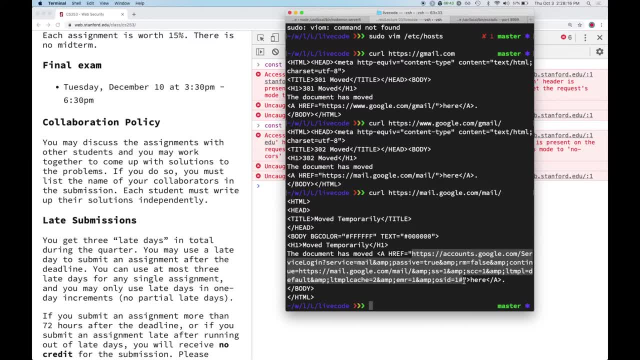 But it's really old and it's really sort of stable and everybody agrees on it. Yeah, Sorry, so when you're executing stuff in the console there, I thought it was coming locally. So I had a question. I guess I'm confused why. 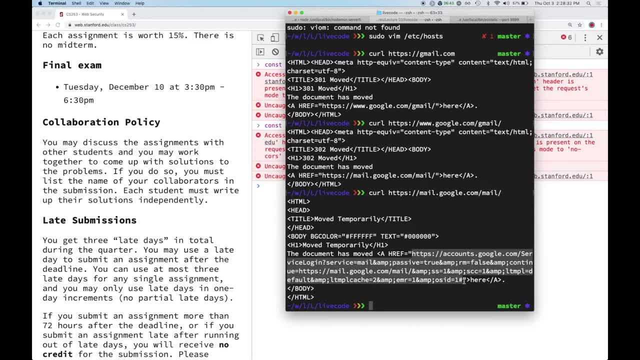 Why the cookies aren't attached, No, like why. why can't you just fetch any site? And it's like I guess it's confusing to me because it's not Gmail that's saying no, you can't access them, you can't fetch them. 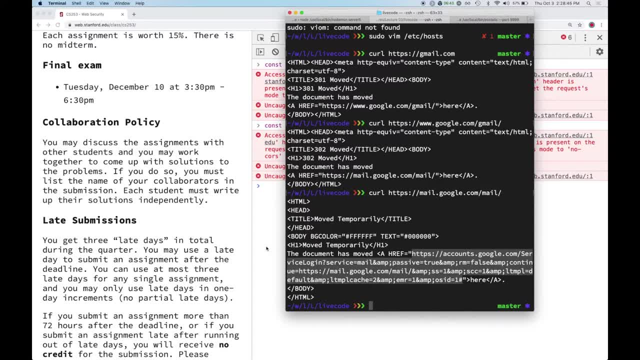 It's the browser saying that. Yeah, the browser is saying that. so in the browser. right, if I go to, actually, I probably shouldn't show this on the screen. I was going to show you my Gmail cookies, but that would be a bad idea. 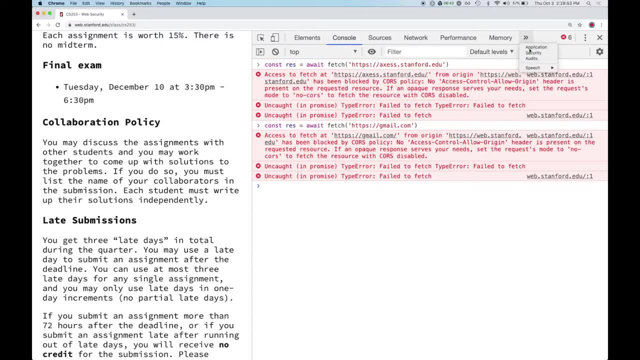 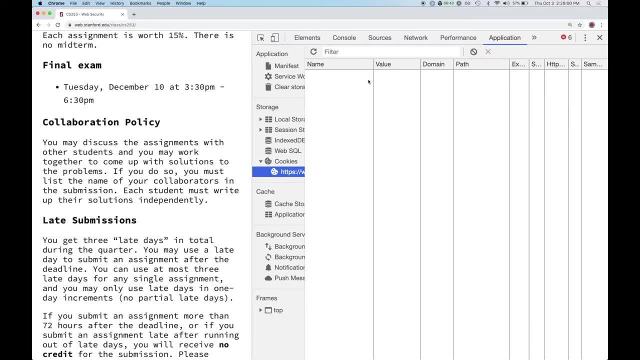 But if I were to go to Gmail and then open up this sort of cookies tab for it, you know we would find. we would find a bunch of cookies for Gmail here that identify me to that server And because the browser was going to attach those, 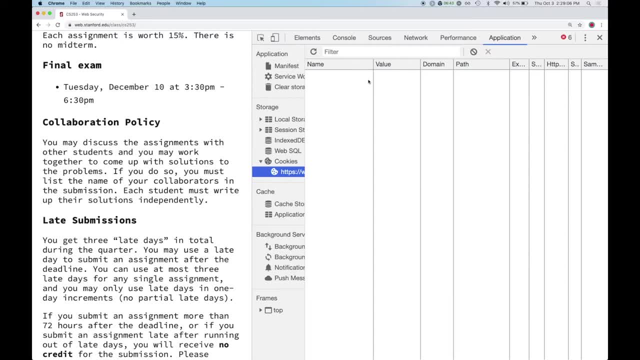 to the requests. that means that the response that comes back could potentially be, you know, personalized to me, right, And the browser? so the browser doesn't want to let an arbitrary site do that. So it's not that the browser is trying to prevent you. 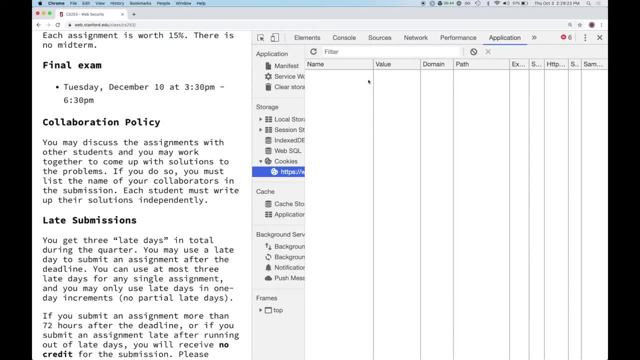 from logging in the console and doing your own thing. Yeah, yeah, It's that. it doesn't want that code being executed from the site that you're working on. It doesn't want it to be executed with the ambient authority of my cookies, right. 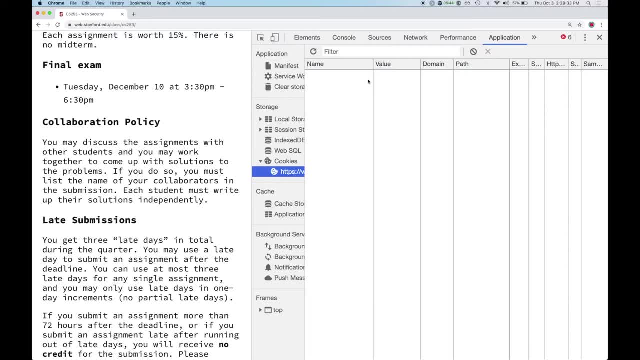 Now the thing that's really maybe a little confusing to you guys about this is that we just saw, like a second ago, that I can submit a form across origins. right, That's what that attack just was before, where that attackercom caused Alice. 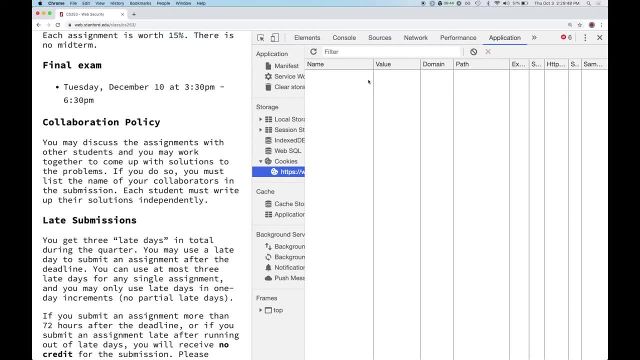 caused Bob to transfer $100 to Alice, right, That is like not intentional, That is like a bug. basically, That is sort of an artifact, like if we could do it over again, we would have everything follow this same origin policy. 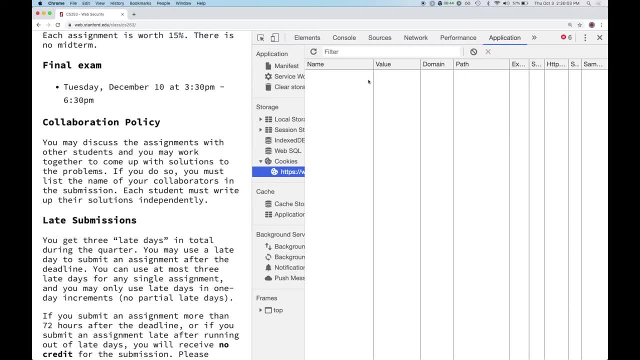 That's just sort of an exception to it for backwards compatibility reasons of you know, forms were able to do this in the early days of the web and nobody has sort of wanted to break that ability, even though it does seem to sort of fly. 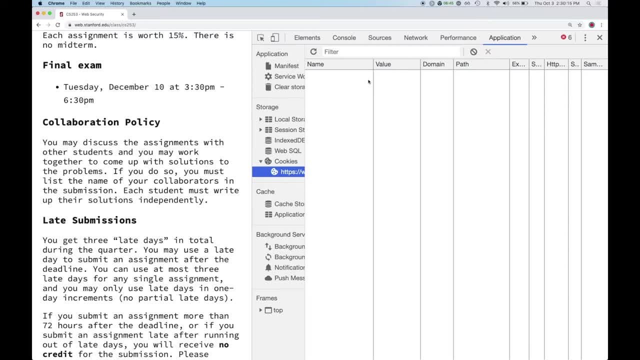 in the face of this same origin policy. because that is, you know, that is literally. you know, site A submitting a form to site B, right, But that's how it is. Yeah, in the back. So is this? because Gmail's? 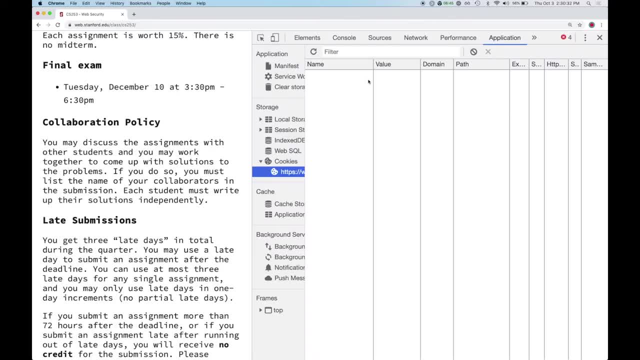 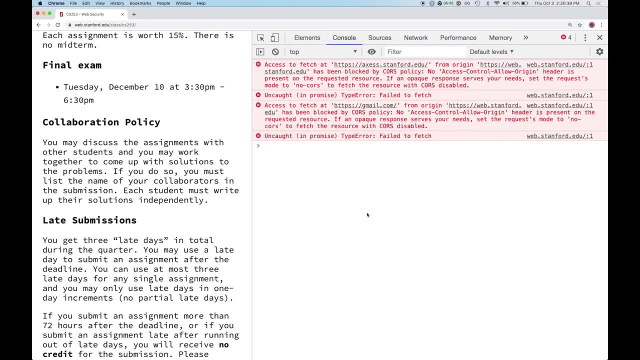 is. the reason it's not working is because Gmail's cookies are set with the same site as the last. I'm wondering: would this work if you, if the Gmail's like session ID cookie or whatever was set to the same site? 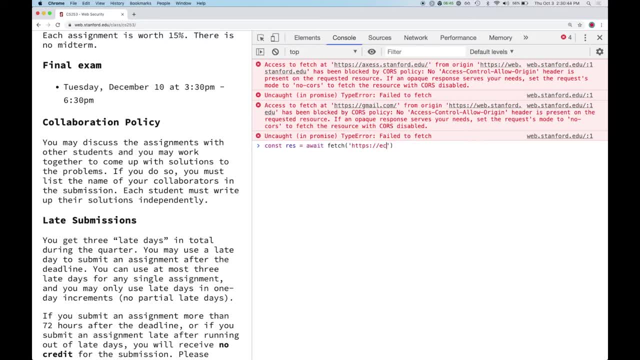 No, no. So it's literally going to, just it's going to block any site, Like I could try anything here. Anything, you know, whatever I put in here is going to fail because it's a different origin. So this whole API just sort of. 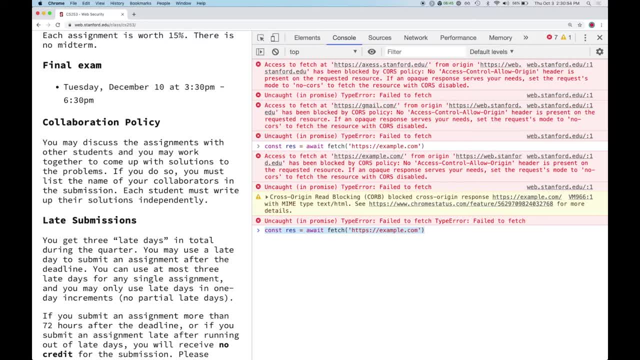 perfectly enforces the same origin policy. This is like a newer thing, so we're able to sort of just be like we're going to do this one right. So this one, you know, this one behaves the way we'd expect. 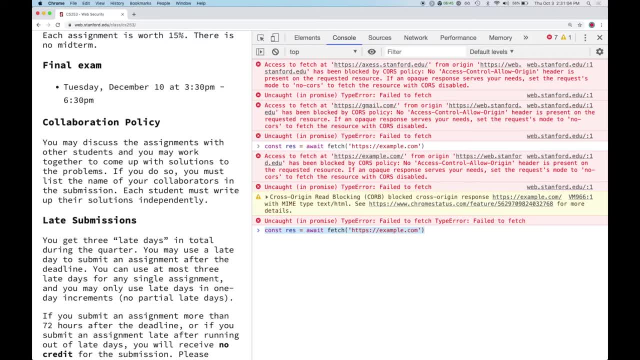 Sites can't. different sites, different origins, can't interact with each other. Yeah, Now there are ways to sort of opt out of this, Like if you're building some kind of an API, you know, and you want to allow developers from different sites. 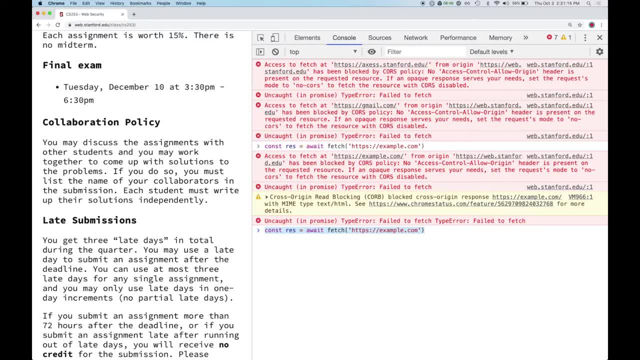 to interact with you. you can relax the restriction, but the default is what we want. It's defaults to being secure. So, like, same origin policy using this API, same origin policy like takes precedence over like the same site could be secure. 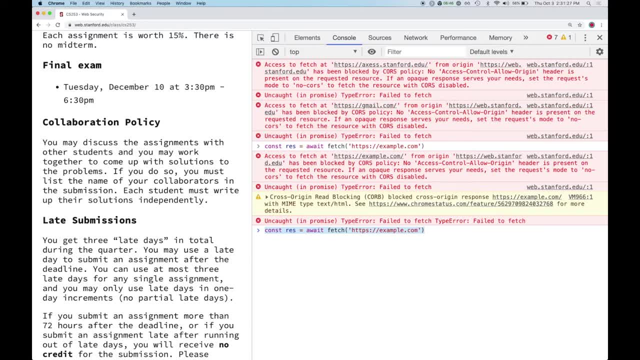 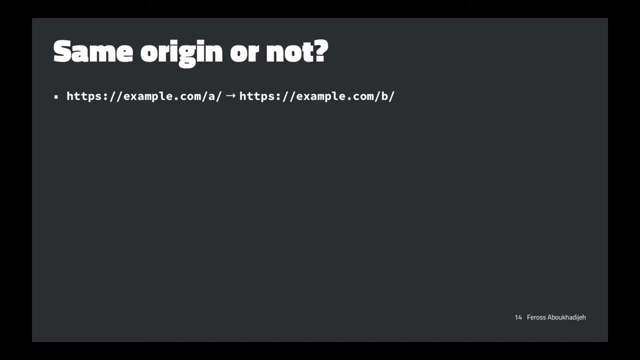 Yeah, Yeah, Okay, I think I need to move on. Okay, so cool. So yeah, a quick review. So are these two sites going to be the same origin or not? Yeah, they are right, Because protocol and hostname are the same. 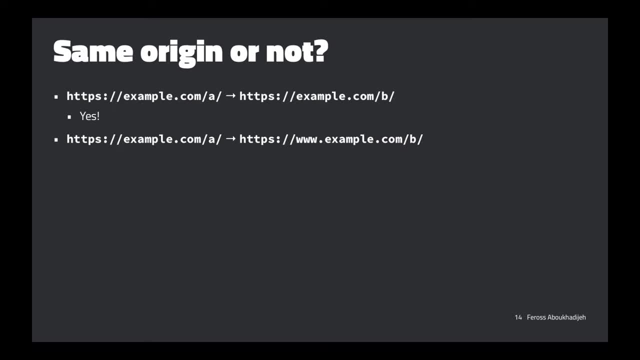 What about these two? Just shout it out. If you have an answer, shout it out. No, Yeah, because wwwexamplecom is different than examplecom, So these are actually different origins. Yeah, a little intuitive, but that's the way it is. 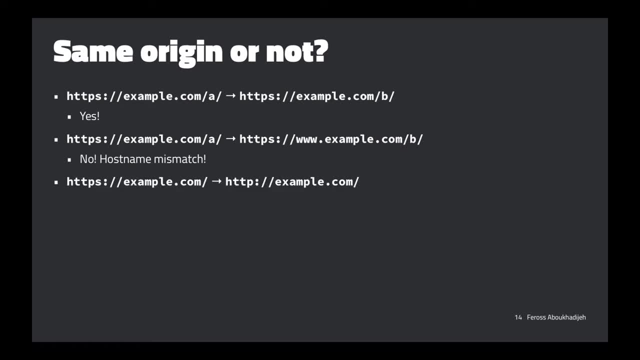 Hostnames do not match. What about these two? Protocols are different, right, Okay. what about these two? No ports are different, because the default port is 80.. What about these two? Yes, yeah, so they're both 80.. 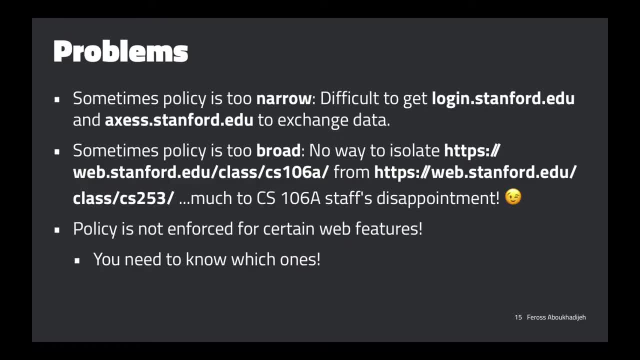 Okay, cool. So the problems with same origin are: sometimes it's too narrow, so sometimes it's restricting us too much In the case of like loginstanfordedu. maybe it wants to cooperate with access, Maybe it wants to allow access. 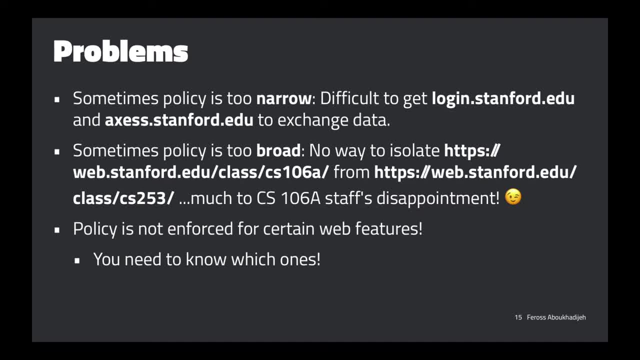 to read the loginstanfordedu cookies, The way the same origin policy works. I guess this is more like cookie policy, but yeah, these aren't allowed to exchange data. And then other times we find the policy is actually too broad. 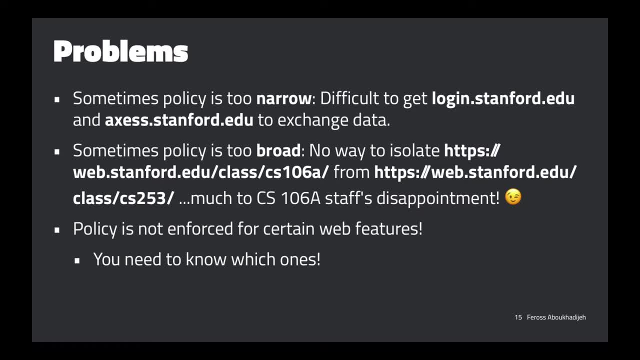 It allows too much stuff. So, for example, with the 106A site and the 253 site- because the origins are actually the same but the actual sites are owned by different organizations- we might want to sort of specify like we want to keep these separate. 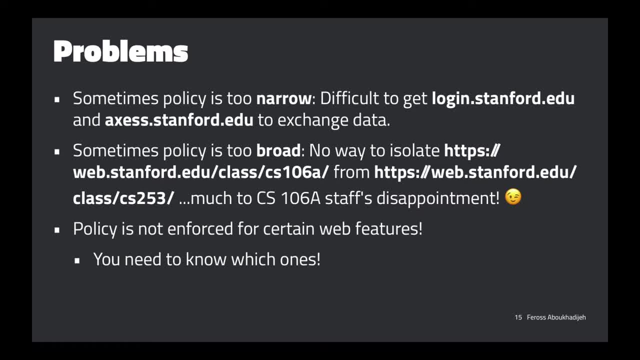 Well, the same origin policy doesn't give us a way to do that. So sometimes it's too narrow, sometimes it's too broad. But yeah, this is what we have to work with. At least it's consistent and at least it's simple. 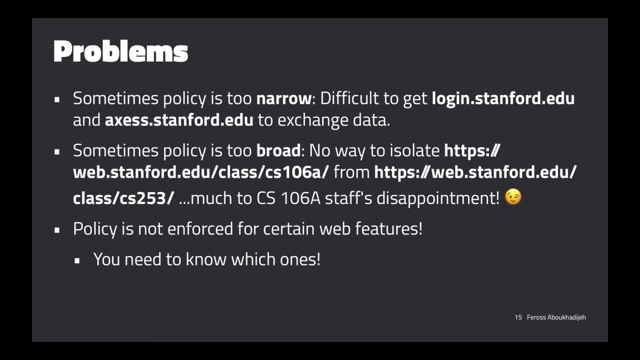 And oh yeah. and then, of course, the other problem is sometimes it's not enforced for certain legacy web features like form submissions, and we need to know which things in particular it's not enforced for. If we don't, then our site will be vulnerable. 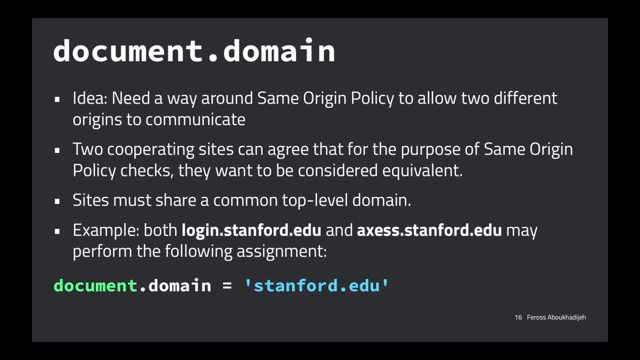 So yeah, So let's talk about a couple of ways to relax the same origin policy when we want to cooperate with another site. So we need an idea. the idea is we need a way to sort of two sites to sort of say: 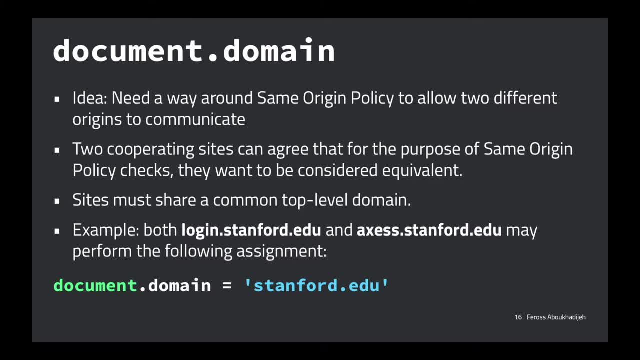 we like each other. we want to talk to each other. How do we do that? So one idea is: this is actually a really, really old API that people threw into the web as a sort of way to do this, But unfortunately it's a really bad idea. 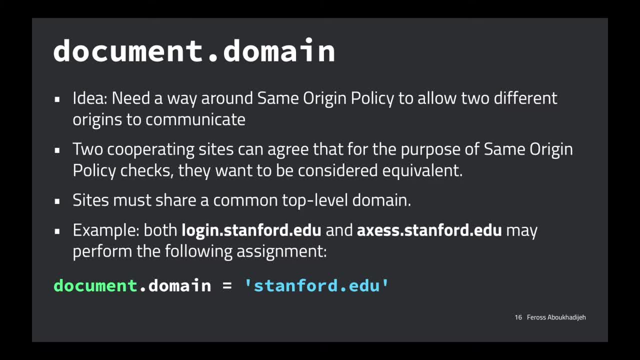 It has a lot of bugs, It has a lot of problems, But we're just gonna go over it quickly so you can see why it's such a bad idea and in case you see it, you'll know to be scared, basically. 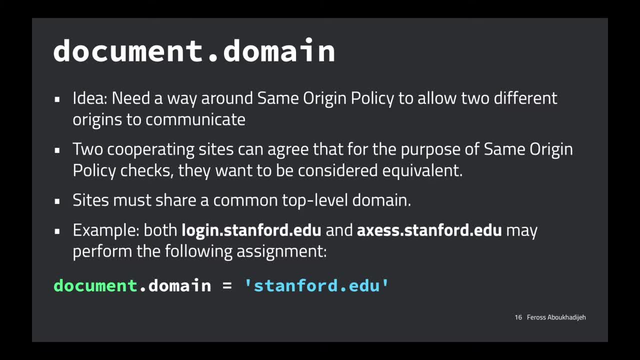 So the idea is- it seems like a good idea at first. The idea is: okay. so say: loginstanfordedu and accessstanfordedu want to cooperate with each other, So they can both run this line of code which says: 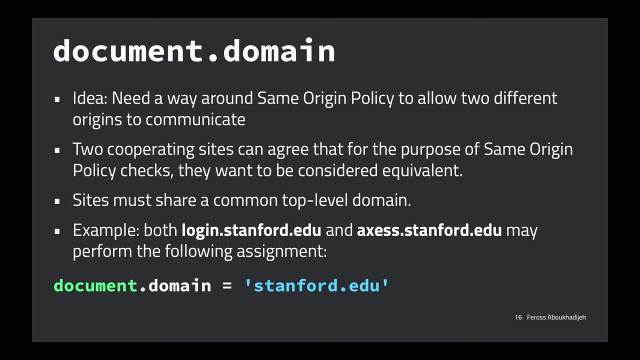 hey, for the purposes of the same origin policy, please just pretend that this is my domain. Okay, Now you can't set this to anything right? Because that seems like it would just break everything. So all you can do is set this to something more general. 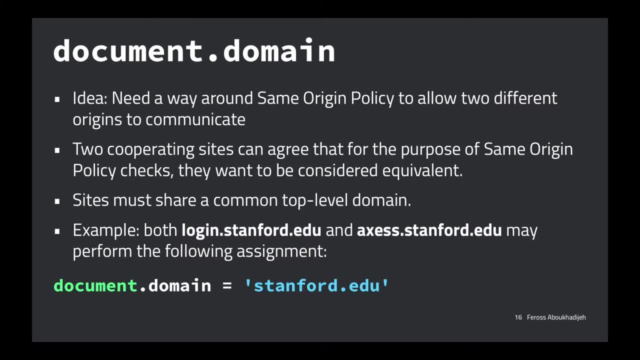 than your domain. So you can log in at stanfordedu. you can sort of chop log in off and it can pretend that it's stanfordedu. In fact, you can even chop off the stanford part and you can pretend that you're edu. 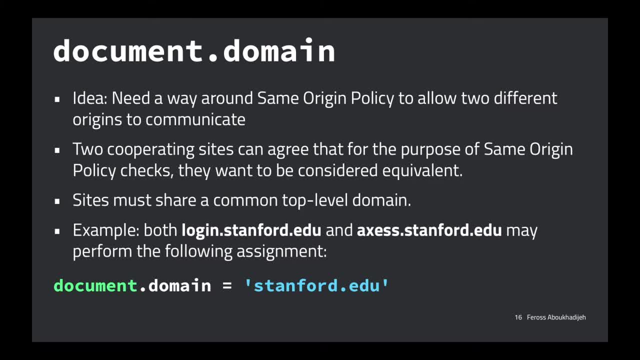 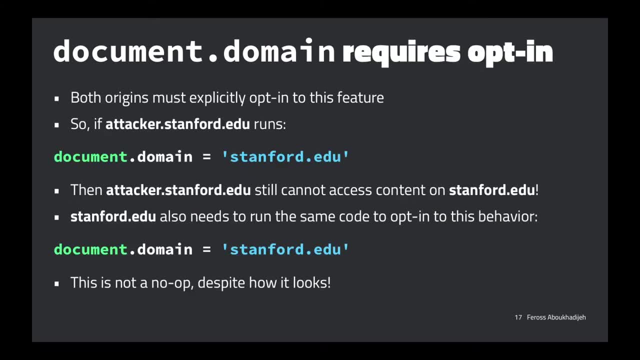 and let anyone any other edu site interact with you. Probably a bad idea, but you can do that. So the idea is both of the sites have to opt in, And so one obvious problem with this is some other person. 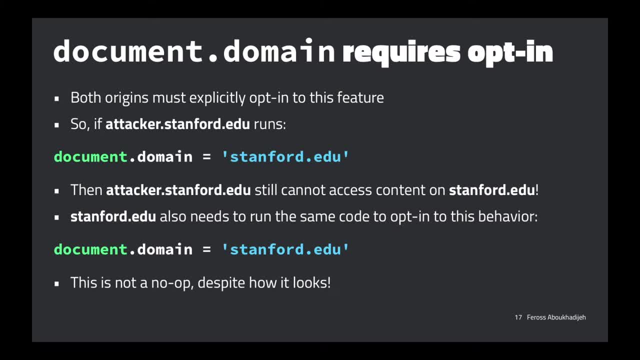 like attackerstanfordedu can also sort of join the party. They can say: oh hey, I also want to be treated as stanfordedu, just like those other two pages. And now suddenly wait, the attacker is still not. 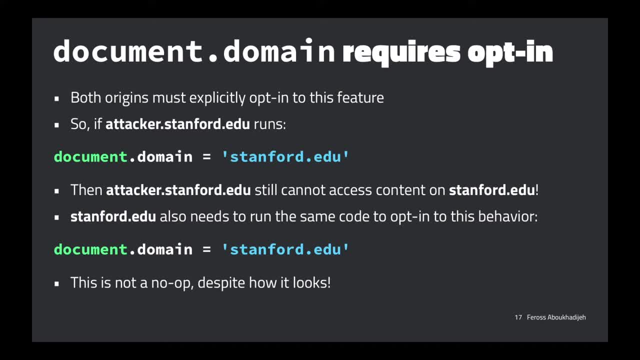 Oh right, right, right, Yeah. So yeah, that's a problem, But what this is saying here is actually slightly different. What this is saying is to say that say that stanfordedu didn't run any line of code here. 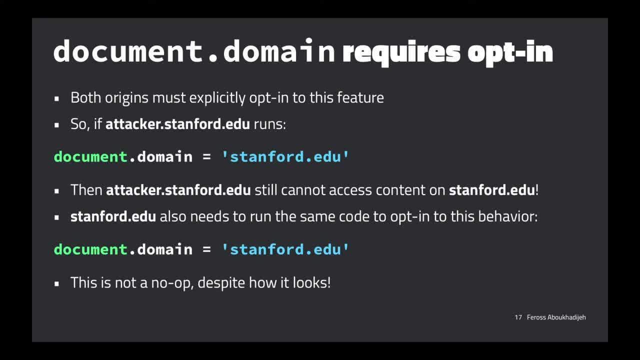 stanfordedu just didn't do anything with documentdomain. Could attackerstanfordedu decide, hey, I want to be stanfordedu for purposes of the same origin policy? It turns out actually no. So stanfordedu itself has to also agree to opt into this. 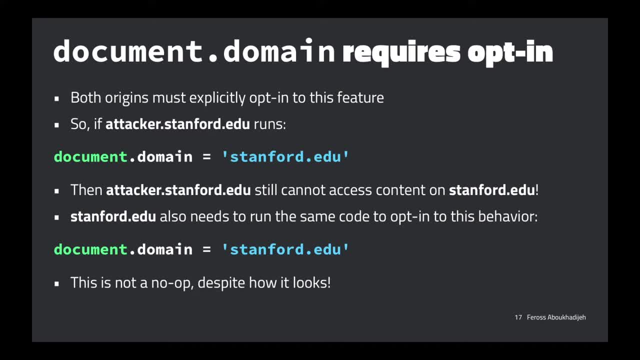 And the way it does that is by setting its own documentdomain to stanfordedu. Now this might seem kind of silly, because you'd think isn't stanfordedu's domain already stanfordedu? So it turns out like: 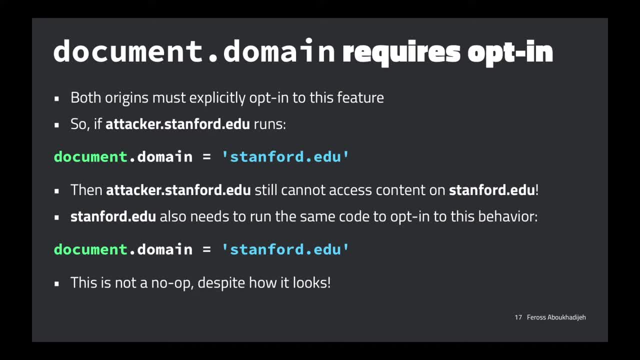 this is not an OOP. This is actually significant. This is sort of stanfordedu indicating that it would like to join this sort of party of like anyone who wants to sort of say that they're stanfordedu, Okay, Yeah, so it's a little confusing. 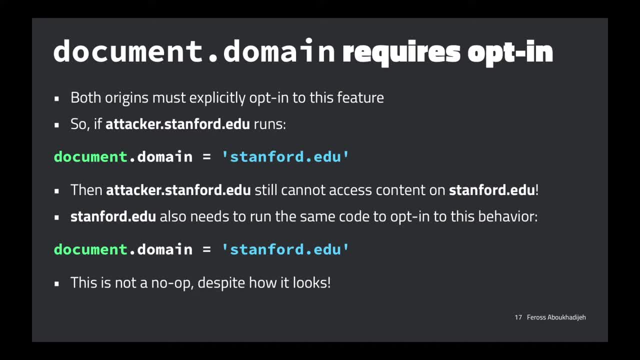 The other thing that's really weird about this is protocol and port are also not settable at all, So you have to both be on the same protocol and port. That part of the comparison can't be changed. You can only change the domain. 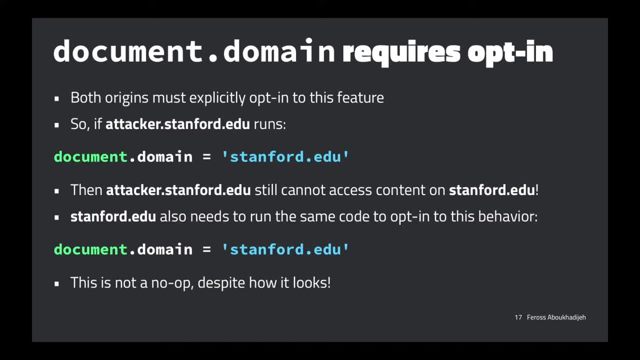 Yeah, question. So if I'm on attackerstanfordedu and this runs and then like a request runs, it will grab stanfordedu, run the JavaScript and then wait to see if documentdomain is going. No, no, no. 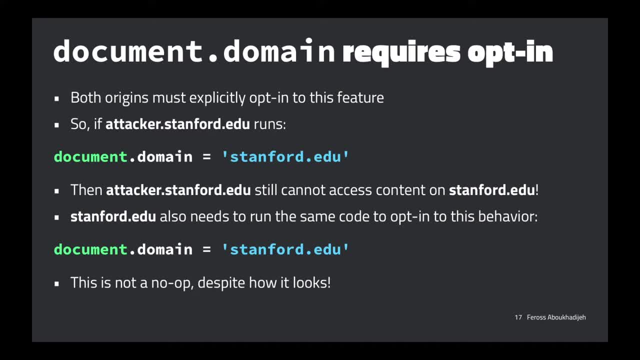 How do you know what they set their thing to? Yeah, yeah, So this is assuming that there's. So if you're trying to interact from attackerstanfordedu and interact in some way with stanfordedu, you must have like. 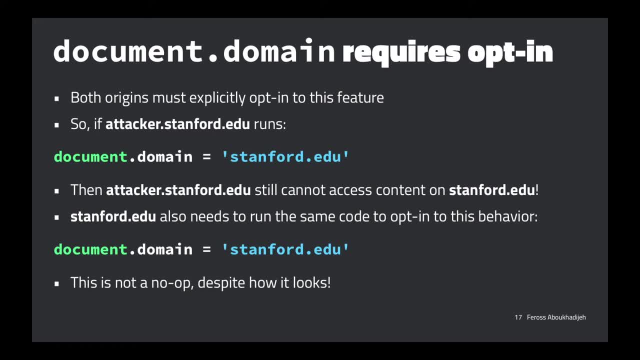 a handle on that, like a reference to a window that is, that has that other site in it. So if you're trying to interact from attackerstanfordedu and interact in some way with stanfordedu, you must have like. 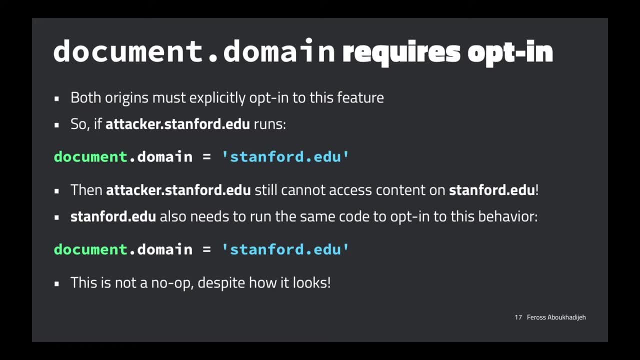 a handle on that, like a reference to that other site in it. So that could be like an iframe. If you have a reference to an iframe with the site you're trying to do something to, then that's when the check will happen. 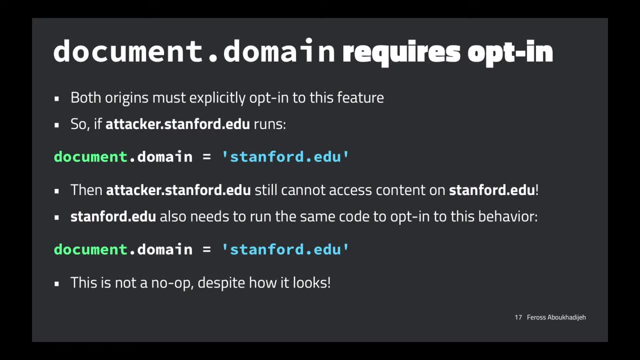 is when you try to actually cross that iframe boundary. It could also be that maybe you open a pop-up window to another site and you have a reference to the window you just opened. That's the same thing, So the boundary is sort of enforced there. 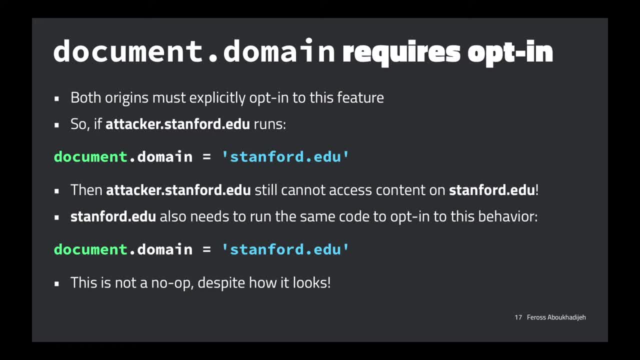 So when it goes to do the check, that page is already ran and if it has done this, then that changes the rules, right? Yeah, question. So just to clarify: when like sets its domain to that and it starts to act. 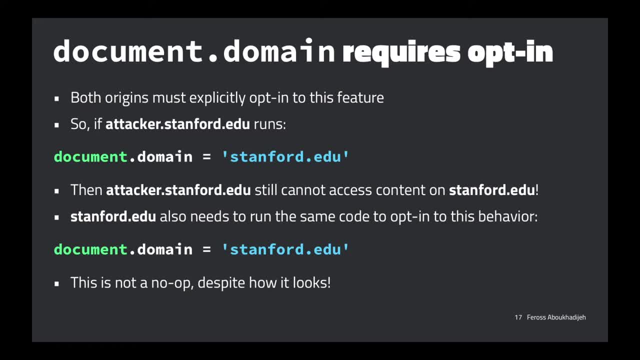 at stanfordedu. stanfordedu decides at that point whether or not it wants to opt in based on No, no, no, So either at the time that attackerstanfordedu is attempting to sort of cross that boundary, if this has been, 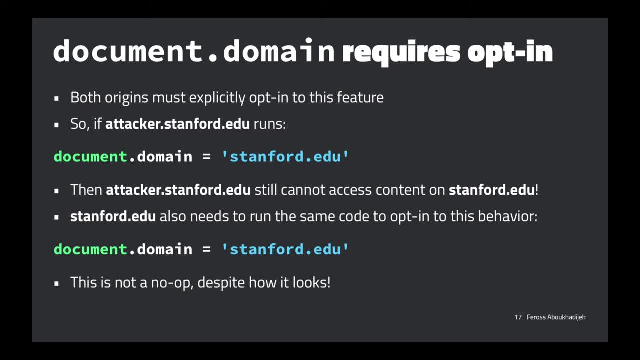 set before, then that will succeed. Oh, so like if another site, like if stanfordedu, agreed to communicate with cstv3.stanfordedu and then set its domain, then attackerstanfordedu could. Yeah, so. 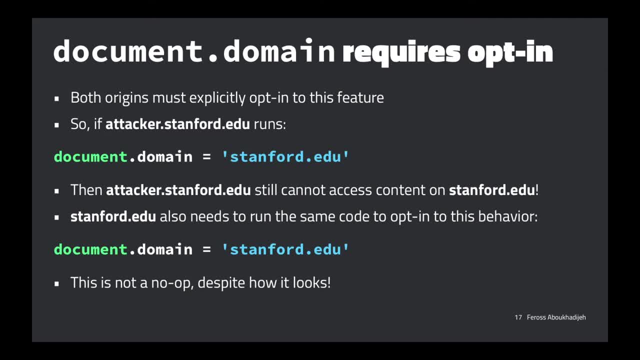 like if the attacker was trying to set its domain to stanfordedu and then stanford already agreed to that. Yes, Yeah, stanford agreed to sort of let anyone on stanfordedu talk to it. Yeah, if it does that. 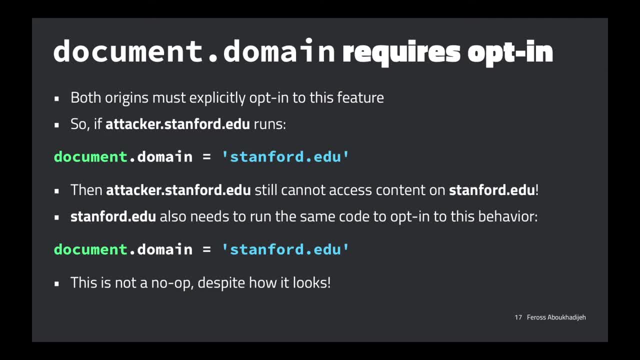 Yep, Yeah, question, Just to be clear: regardless of any of those attackerstanfordedu can by default access all of stanfordedu's pictures, right? Uh, yeah, That's a good point. Yeah, good, good. 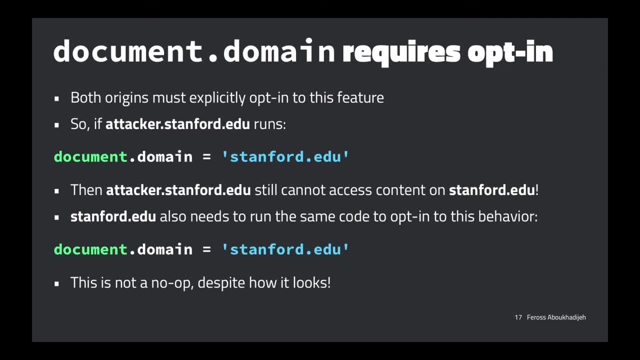 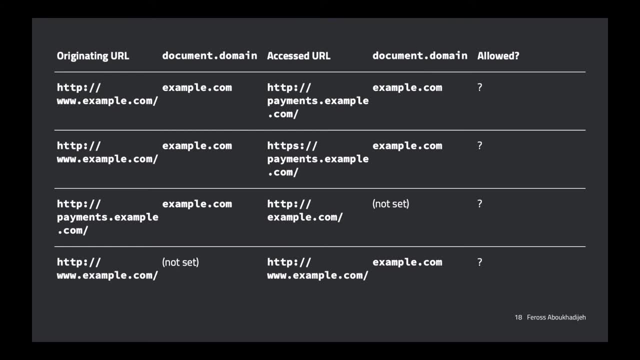 good check. Yeah, that's because the way cookies work right. So, yeah, Yeah, That's a good point. Yeah, but this is sort of okay, so so I think we'll skip this. This is not too important. 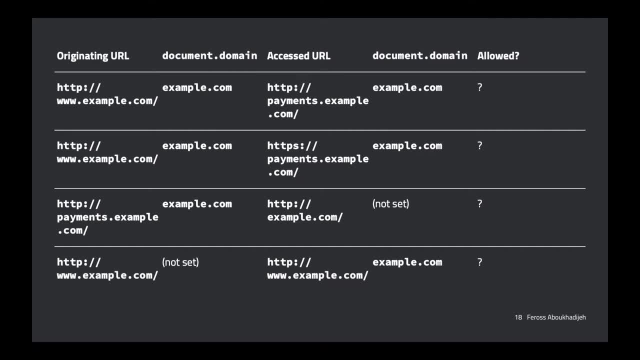 This is just sort of ensuring that we all understand the way that you know all the things we just talked about of sort of how how setting documentdomain or not setting it affects whether something is allowed or not. But you can go ahead and take a look at this. 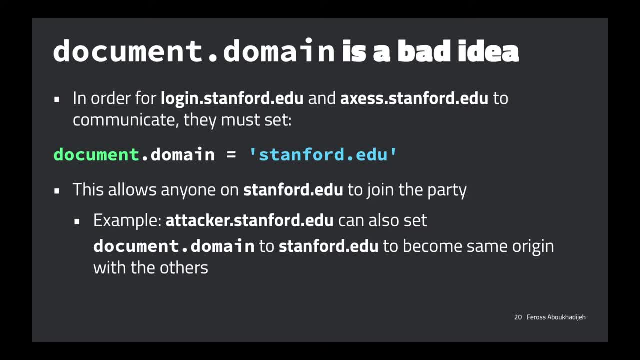 in the slides, if you're curious. It's not too important, But but just to emphasize why it's a bad idea, right? It's that if login and access want to talk to each other, they're gonna run this code and then now anyone on. 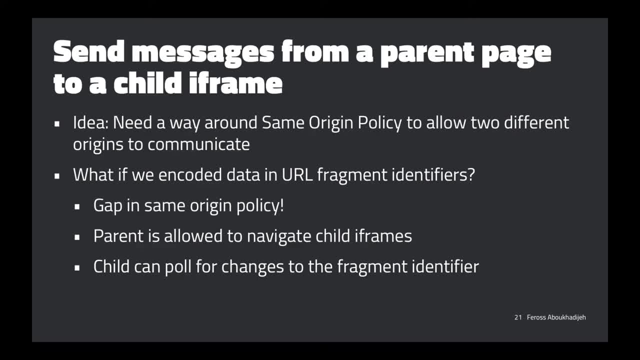 that page. So this is a problem, Okay, So, so let's, let's just rule that out. Never use that. Forget about it. If you see it, you know, just be afraid, and make sure you look at all the details. 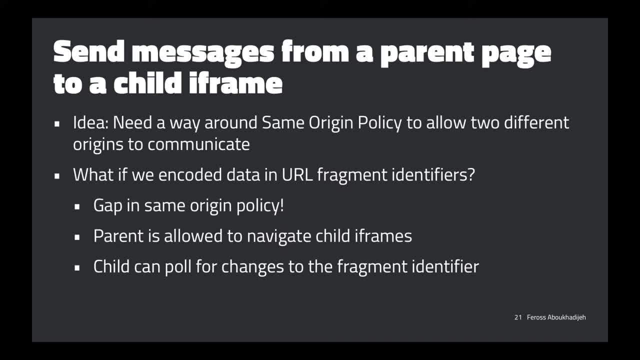 because something's probably going wrong. But but so let's talk about another way you might be able to sort of get around the same origin policy if you want to communicate with another page. So again, we're gonna try and find a way to get around it. 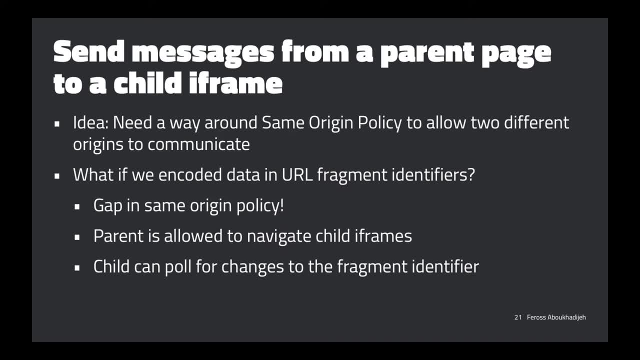 Hopefully it's not as bad of an idea. So create a a setup where so say, access wants to talk to loginstanfordedu, So could could access put maybe an iframe in the page that contained the loginstanfordedu page? 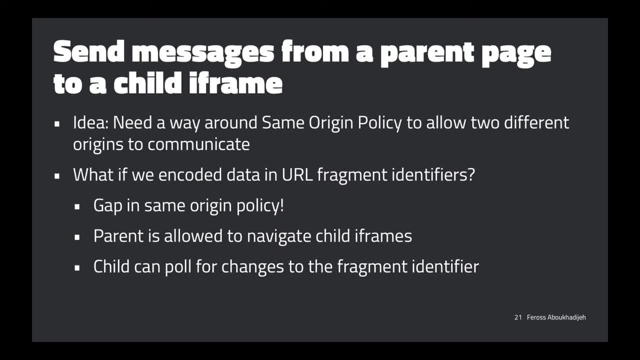 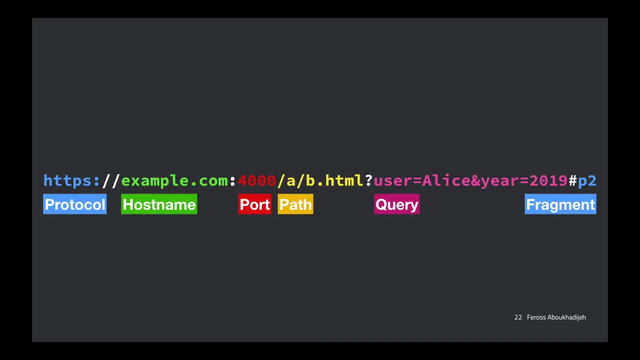 and then and then change. this is. this is so, so gross, but do you remember the, the fragment identifier in this part of the URL? Okay, So so, if I so? we just said that iframes can change the source. 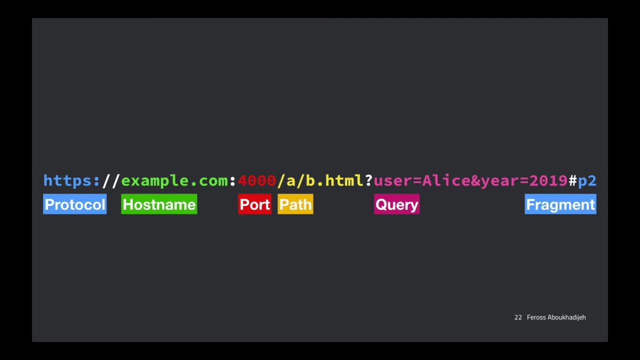 of their. if I created an iframe, can navigate it to new URLs, right? We just saw that I. I set the crypto, I moved crypto to examplecom. So what if I I do that, but instead of actually navigating it to a new page? 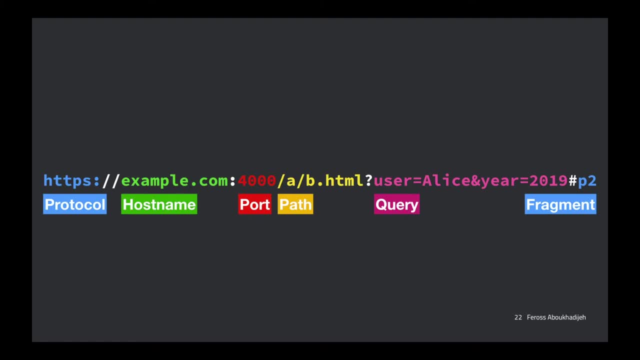 I just change the the fragment part of the URL, So this actually doesn't cause the a page to reload. What this does, is it just sort of it jumps the user to a different part of the page right Based on whatever. 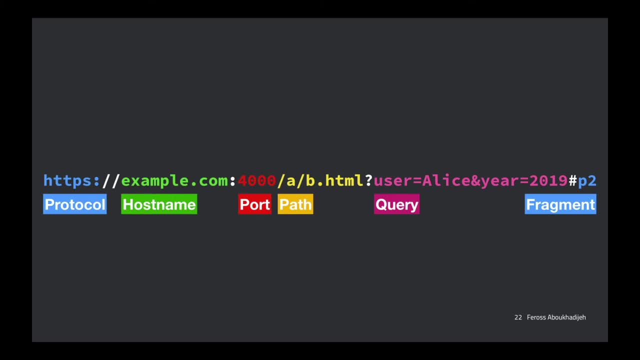 this fragment is. But if the fragment doesn't exist in the page, or if the page doesn't exist in the page, then what happens is: if the page doesn't exist in the page, then what happens is: if the page doesn't exist in the page. 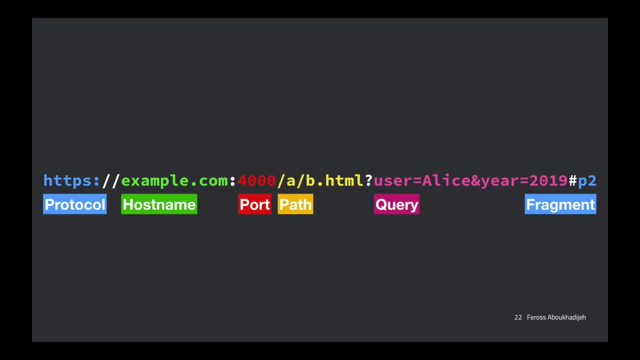 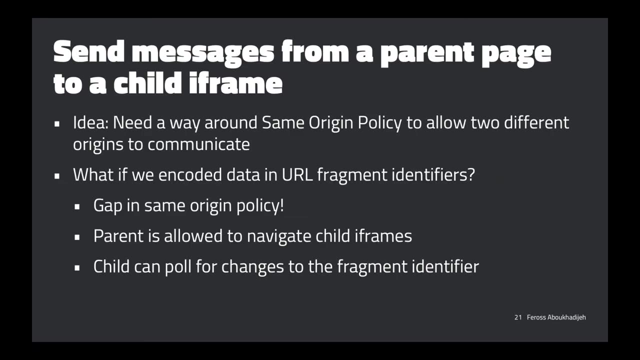 then what happens is, if the page doesn't exist in the page, then what happens? So if I did that and then the page repeatedly checked its own URL to see what the fragment was, we could use this as a communication channel. So this is really. 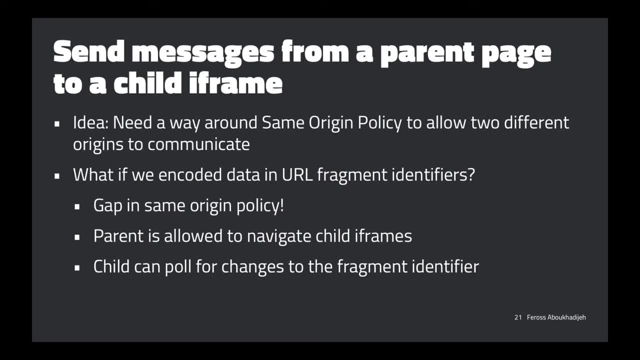 kind of ridiculous, but let's just make sure we all understand So. so so parents are allowed to navigate through the web, and then they can navigate through the web. So this is actually the way that we got around the same origin policy for like a really. 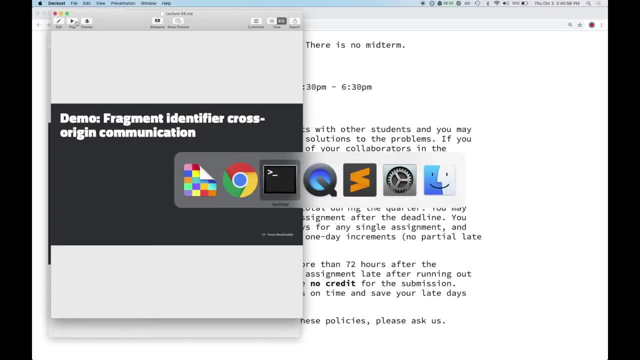 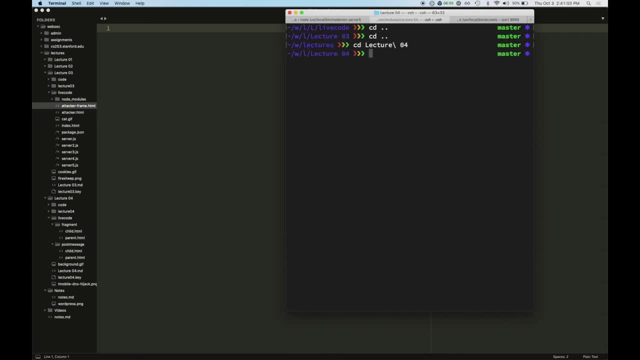 really long time on the web because there was there's no other way to sort of opt out of it for this use case. So yeah, so we're just gonna just gonna show you this for like sort of historical reasons, because I think it's. 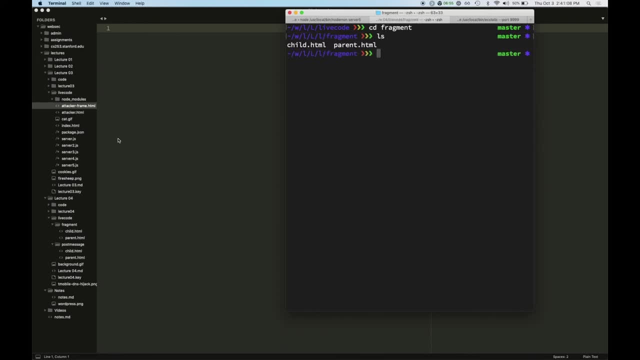 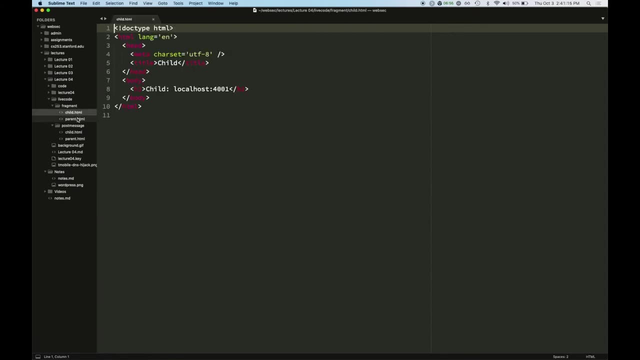 I think it's actually just hilarious. So go to lecture 4 live code and let's actually try to try to implement this. So okay, so let's, let's go ahead and let's see here. So in the parent. 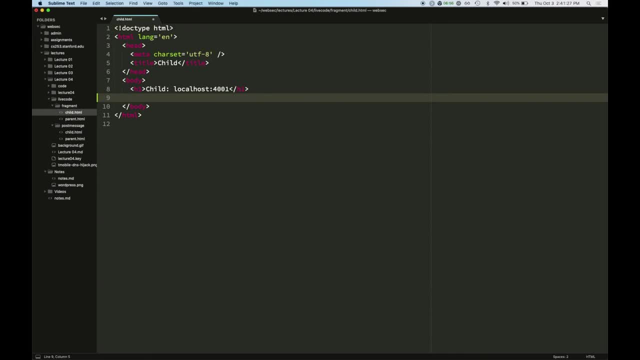 what I want to do is actually: let's start with the child. So let's start with the child. The child is going to- let's say it's it's whole job is it's just gonna try and display the, the fragment. 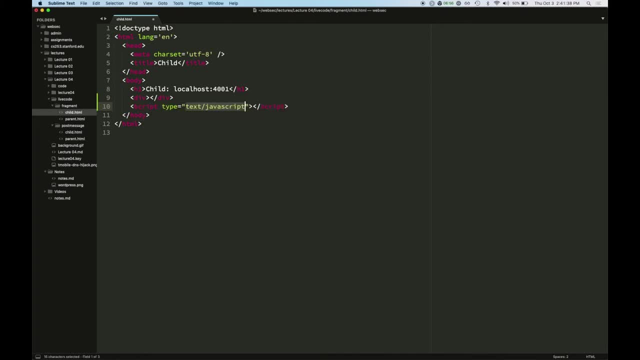 that it's been given. So this is sort of the message from the parent. So we'll include a script here and we will just get this div that we, that we just created above and I'm just going to put into the div, sort of the. 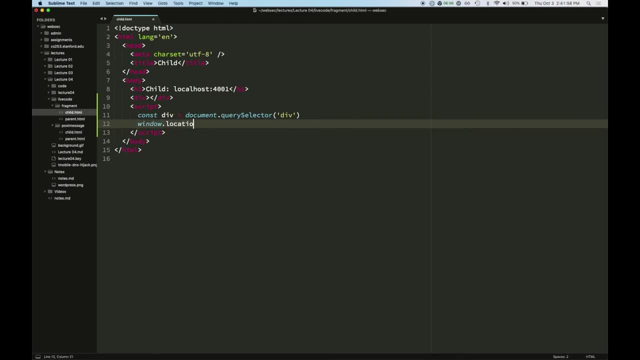 the result of, basically the result of what, what is in the window, dot location, dot hash- which is that that fragment identifier and I'm gonna decode. I'm just gonna decode the contents of it so that it renders a little bit nicer, and I'm gonna slice off the. 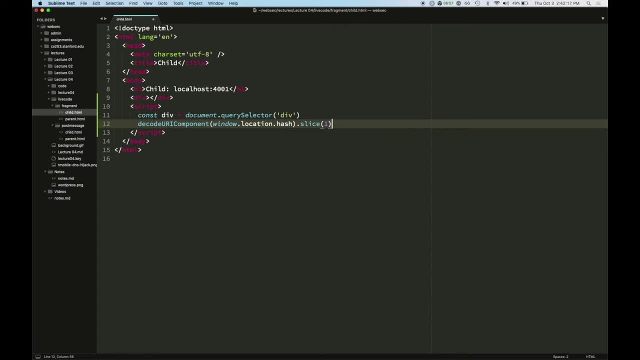 this is gonna slice off the leading hash, So we just get this stuff after the hash, and what I'm gonna do is I'm gonna repeatedly pull: Yeah, this is I kid you not, this is how it was done, It's. 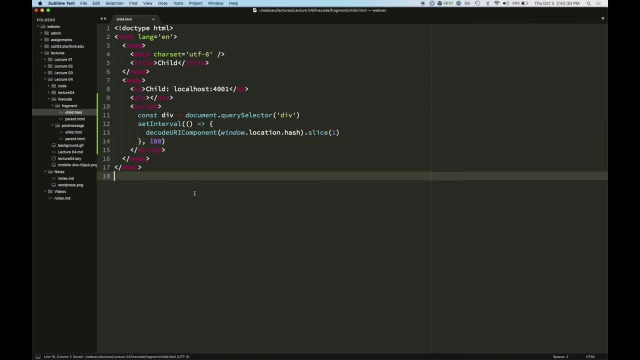 it's incredible. Okay, so every tenth of a second we're just gonna see: hey, is the hash different? and oh yeah. and then what I wanna do when I actually get it? I actually wanna, I wanna set it to be the contents of the div. 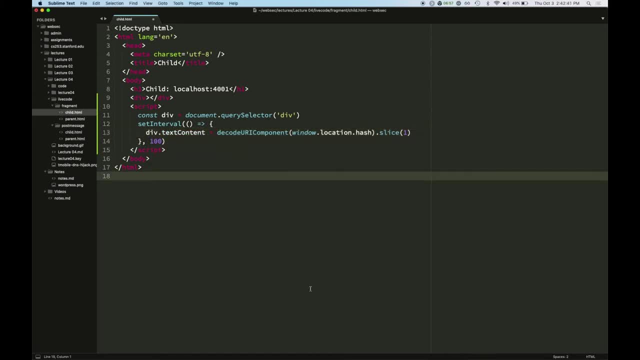 just so that we can see it. So I'll just do div dot. text content equals that. Okay, so cool. So now now in the parent, this is going to. obviously this needs to embed the child iframe, and so that'll be. 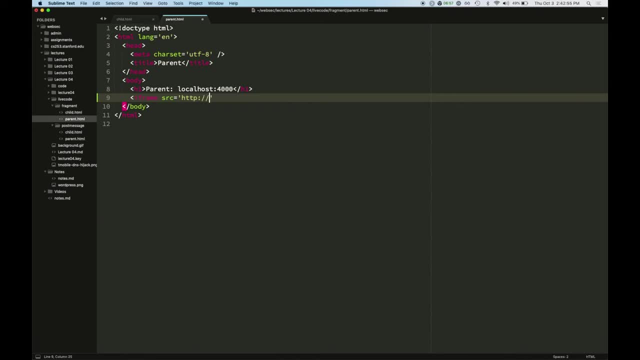 this is gonna be now. to simulate that we're dealing with two sites here, I'm going to, I'm going to use a different origin. So so the parent is on 4000 and the child is on 4001.. Okay, 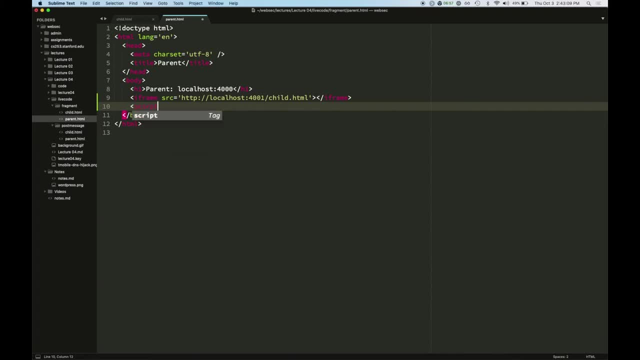 so we're gonna include the child, just like that. and now let's, let's create a way for the parent, let's let's create some mechanism for actually sort of talking to the child. So what I'm gonna do is I'll make an input. 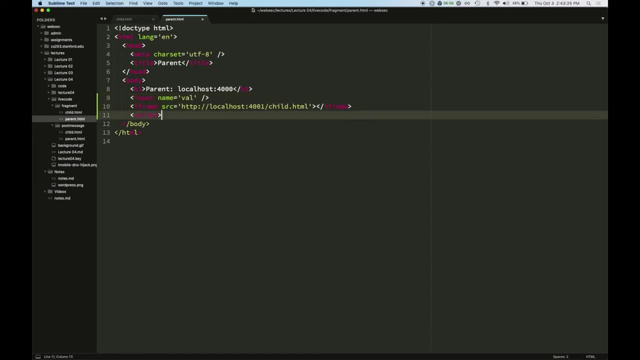 which will have the name val, and then I'm gonna make my script sort of: yeah, actually, let me add some new lines here too, really quick, Okay. so then I'll make my script look at that input value and just pull that off of the. 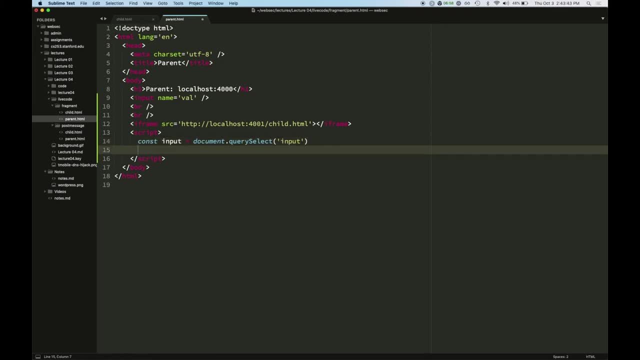 the input and I will get a reference to the frame as well. Oops, query selector. Okay, and then I need to now basically listen for key key presses on the input. So we're gonna listen for an input event and whenever that fires. 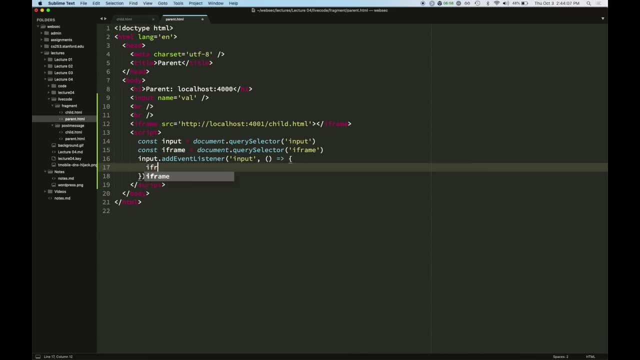 we know that the user's typed something into the form, So what we're gonna do then, is set the iframe source to be- let's basically set it to the same thing that it was before, except for we're gonna tack on hash, and then we're gonna basically do. 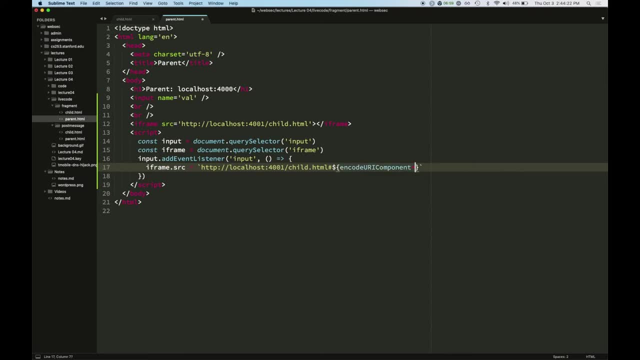 encode URI component of the input's value. Okay, all right, Everybody follow that, So I'm just gonna keep setting its source and because it's a fragment hash, it's not gonna actually navigate the frame to a new new page. Okay. 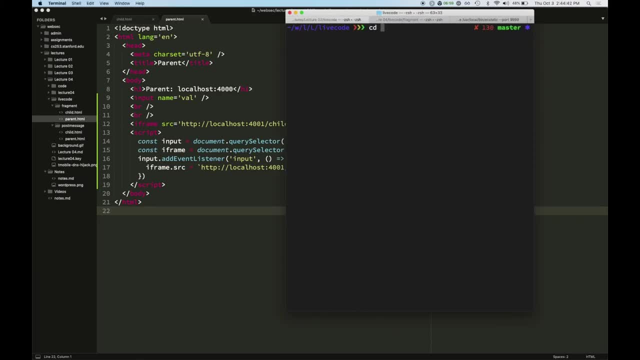 so now, if I, if I run this, so how do we run this? So okay, so we need to make sure we're in the right folder. We need to start two servers, one on port 4,000 and one on port 4,001.. 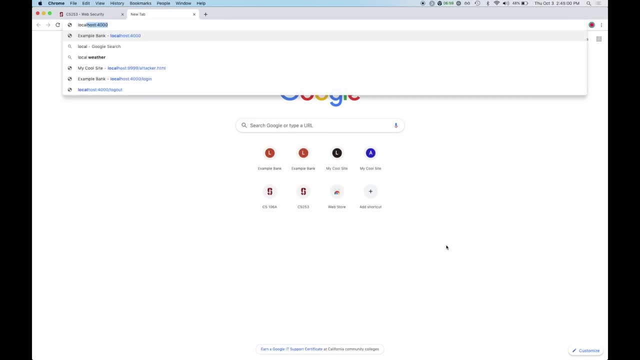 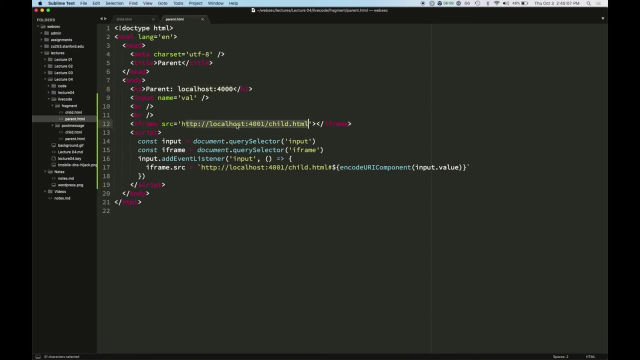 Okay, and then what we can do is we can go to. so just to confirm, so the parent is on 4,000.. So if we visit the parent, it's gonna embed the child in an iframe on 4,001.. 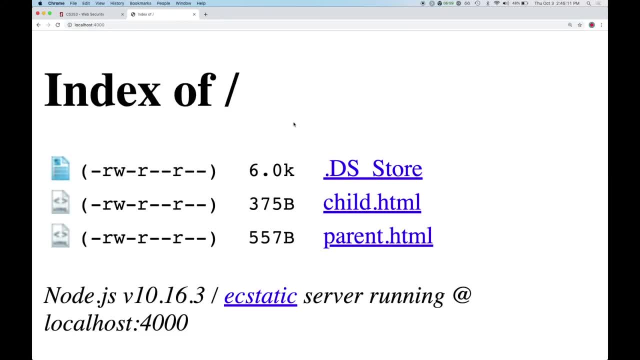 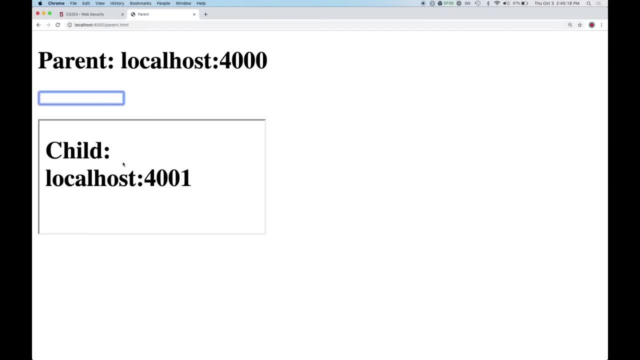 So I should. it should just be enough for me to go to 4,000 and then go to parent. Okay, so that's what we got. So we got. here's the parent page. It has an input box, and then it has. 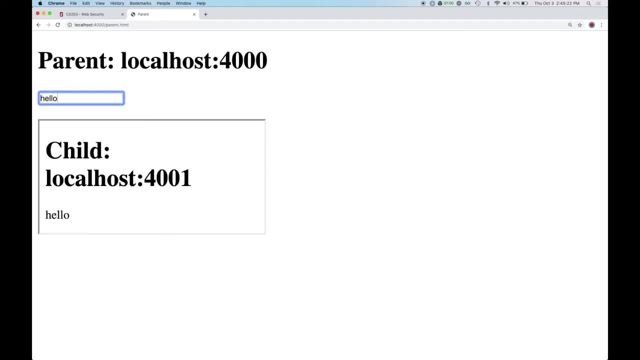 this child iframe And if I now type in here, you can see that with a little bit of a delay it's copying over the the text And if we actually- here's the cool part- If you actually pull this open and you look at the iframe. 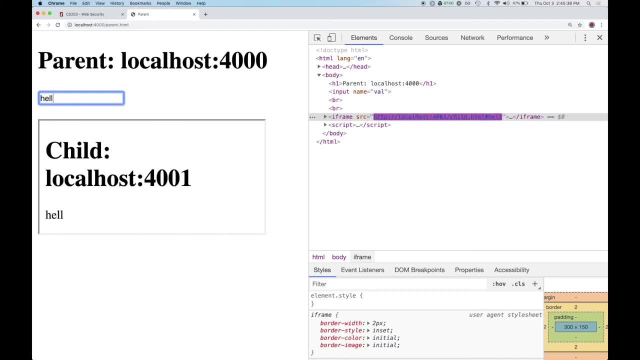 check out the check out the source, As I, as I type it, actually it actually updates. So that's actually that's. that's that's cross-origin communication, right there? Yeah, Cool, So let's see here. 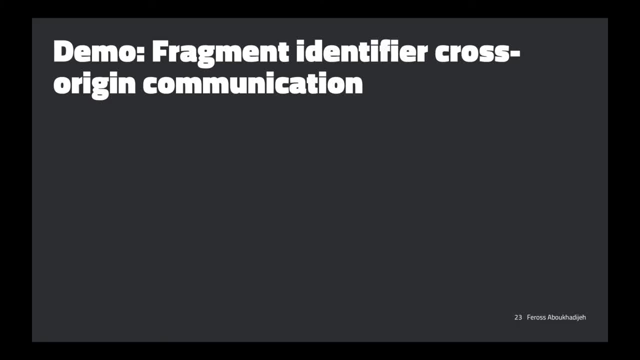 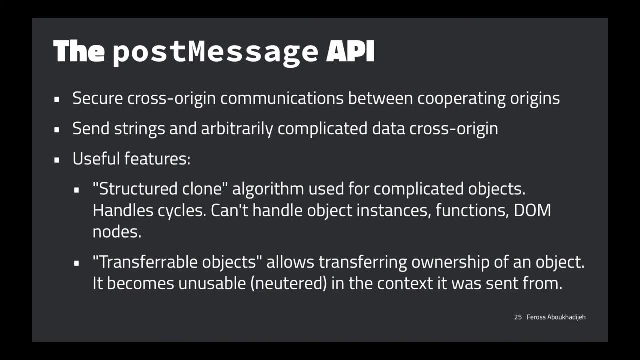 We have five minutes. Do I have time to show more things? Yeah, I think we have time for one more thing, So let's see if we can do it. So so this is obviously gross. So eventually everybody grew up and decided to actually 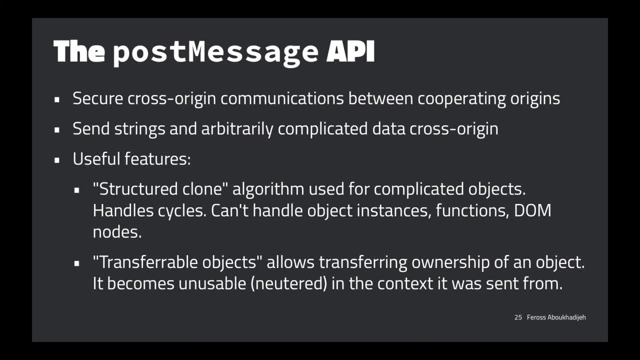 make a proper API for for allowing communication between sites, And this lets you basically send any kind of string or any kind of object that you want between two, two origins, And it has some nice features. So one thing it does is, if you have 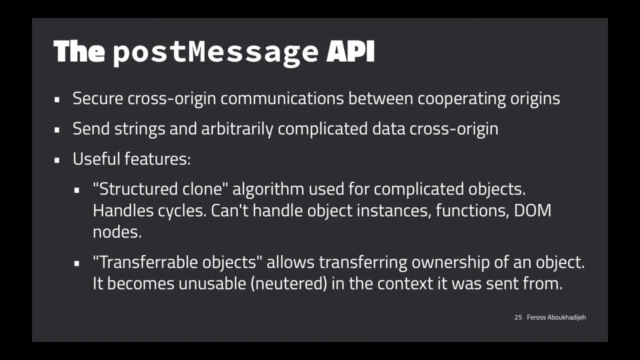 a complicated object with, like maybe you know, many properties and subproperties and arrays and all kinds of different things in there, it'll actually clone that across and reproduce it on the other side And it'll even handle cycles. So if the object 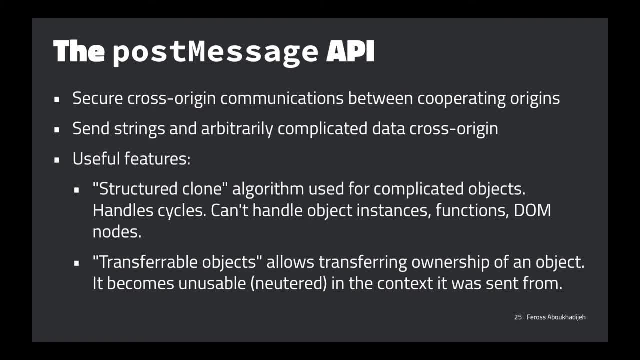 has something that references another part of it, that'll, that'll work. You can't send across functions for DOM nodes or instances of objects, but, but it works for lots of things And you can even transfer ownership of an object. So I could send. 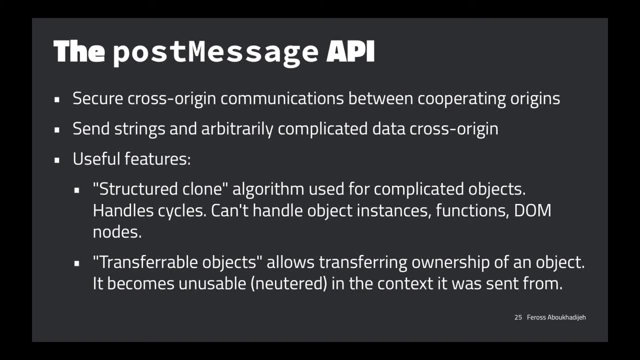 like, say, I have like a gigabyte array of like graphics data or something and I want to send it to another page. That could be really slow to sort of copy across, because I need to give that page an entirely different copy of this data because in JavaScript, 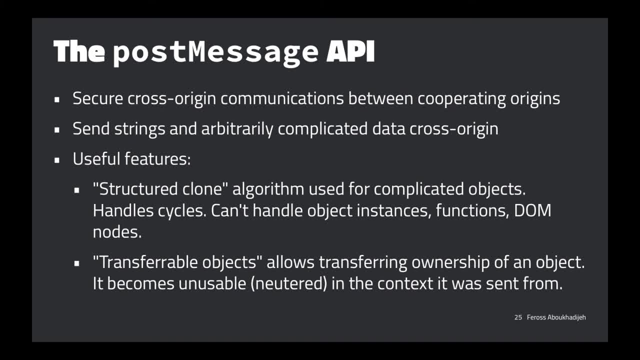 we don't. we don't have like threads or any ways of sort of sharing memory. So one thing you can do is, instead of copying that, that gigabyte array, across to the to the other page, you can use this thing called transferable objects. 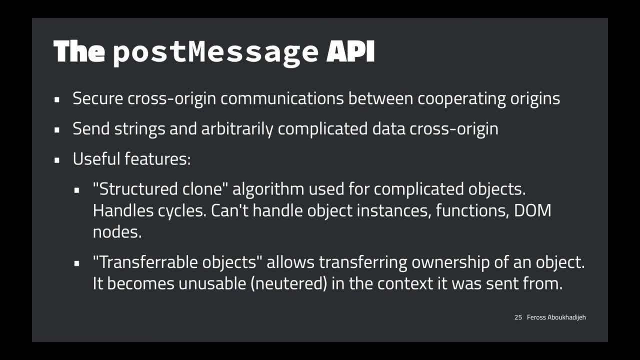 where you sort of say: I want to basically give this object to the other site and then you lose your handle on it. You've sort of gifted it to this other origin and that happens like instantaneously, So you can actually do sort of zero copy. 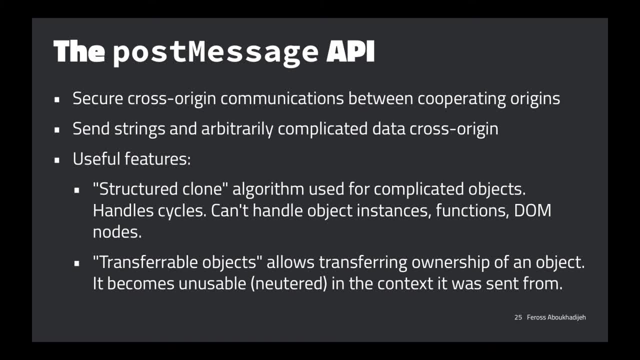 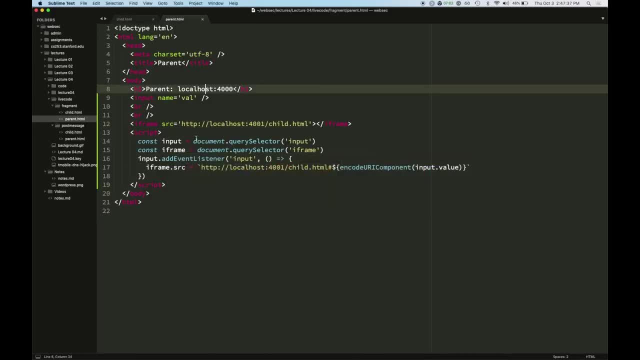 transfers of of data, but then you lose your reference to the object, which is, it's kind of interesting, Anyway. so, okay, so let's see. so all we need to do to use this API is just make a couple of changes here. 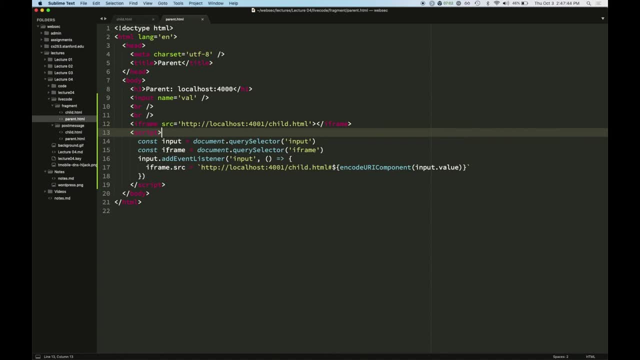 So so how about now? whenever we type, instead of doing this jank thing, what we're going to do instead is we're just going to on the iframe, we're going to get a handle on the window and we'll call post message with the message. 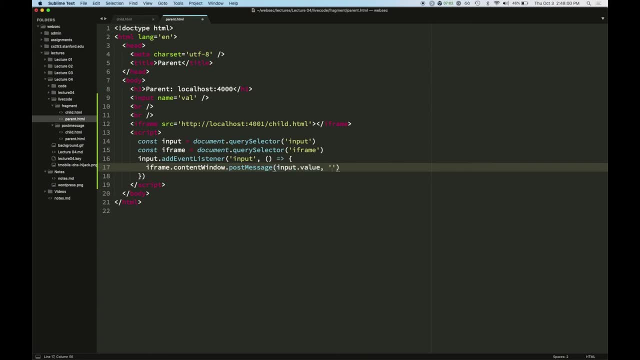 which is inputvalue, and then what we put here is: this is the, the origin of the site we want to talk to. So I'll talk about why that's important in a second, but for now, just look at, this is the value that we're sort of. 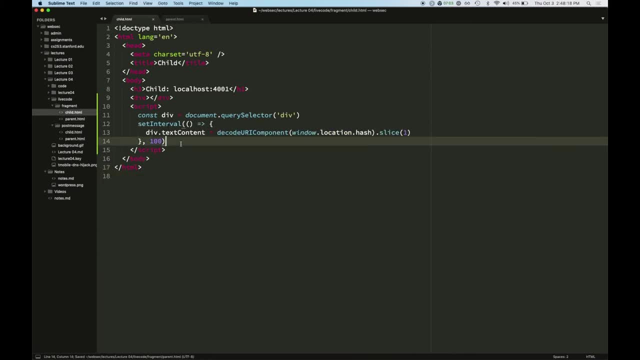 messaging into this iframe. Okay, so then, what does the iframe need to do? Well, okay, we can remove this stuff. It doesn't need to pull every hundred milliseconds anymore. Now, what it can do is it can just, it can just register. 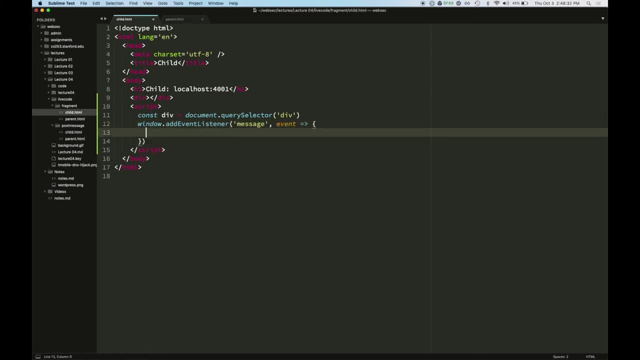 the fact that it's interested in these message events by saying on message: basically, Whenever a message happens, just run this, this function, and update the content of the div with the data that was sent across in that message. Yeah, and one other thing I'm going to throw in here. 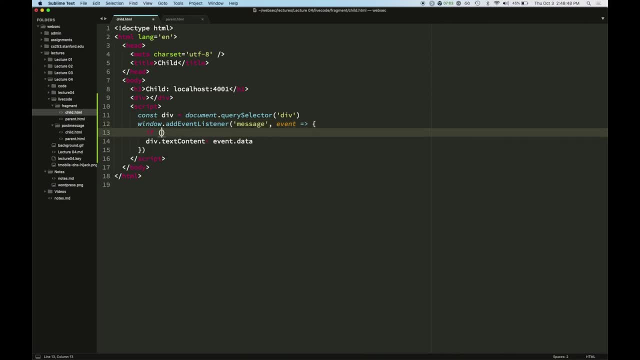 is. I'm going to just check where this message came from. I'm going to mention next time- I guess because we're out of time now- why I need to do this, but really bad things happen if you don't do this, But so all I'm doing here. 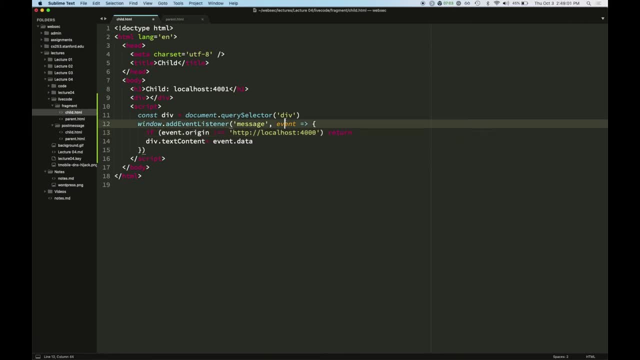 is. I'm saying: where did this event come from? If it didn't come from the parent in in, in which is this origin? then just return and don't actually do anything with this message. Otherwise, go ahead and display it And the parent. 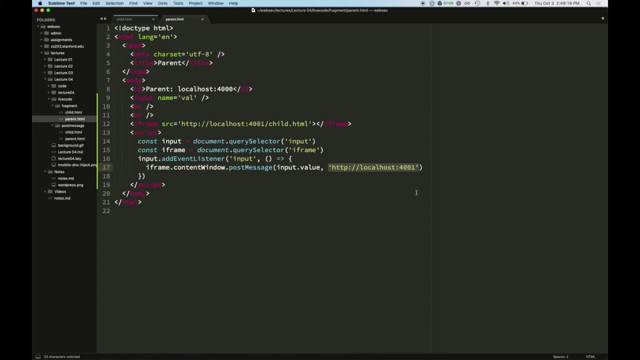 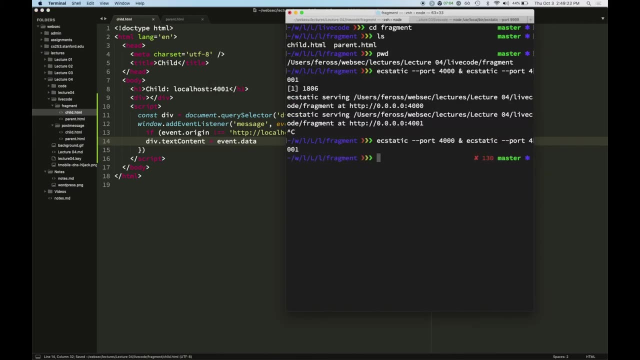 has a sort of analogous thing on the other end, where it sort of ensures that that its message is going to who it wants to go to. Cool. So so now let's go ahead and just see what happens here. So I will. 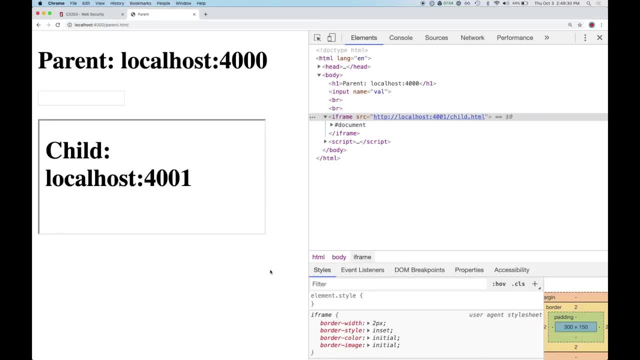 restart the servers and we'll see. see what happens here. So so now, if I type in this box and I say hello, you'll notice that the URL will show up. So that's great. we're not using the old method and it's. 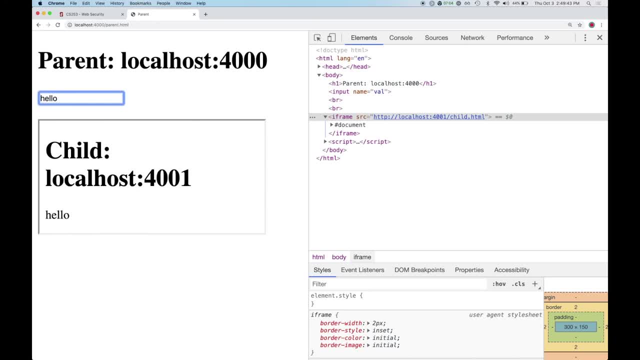 it's instant, so it's it's faster and nicer. So yeah, this is one way to get around the same origin policy. if both pages want to cooperate with each other and communicate some useful information and use post message- Cool. So I think we're out of time. 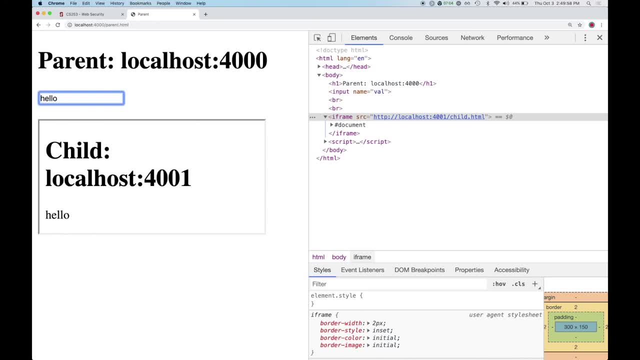 but thanks everybody, and I'm having office hours now from 3 to 5, so if you have questions you can, you can come to that. But yeah, thanks, Have a great weekend.